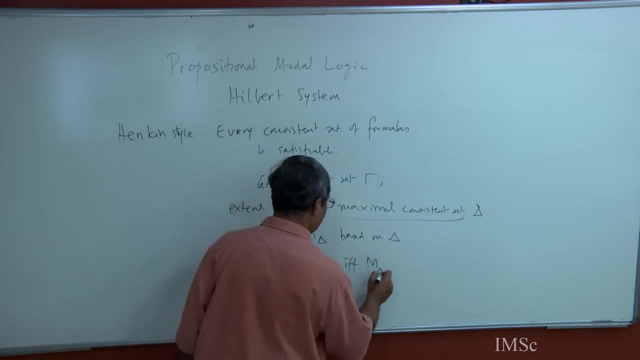 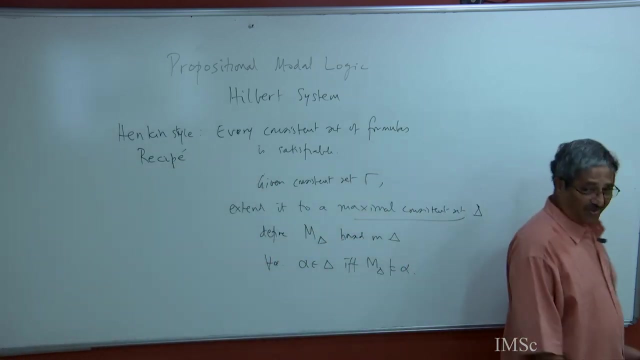 to delta if, and only if, right, remember. So the idea of truth in the model is reduced to membership in the set right. And this is the recipe, This is the general recipe, So, and that is what you are going to do as well, Except that and the idea of consistent, 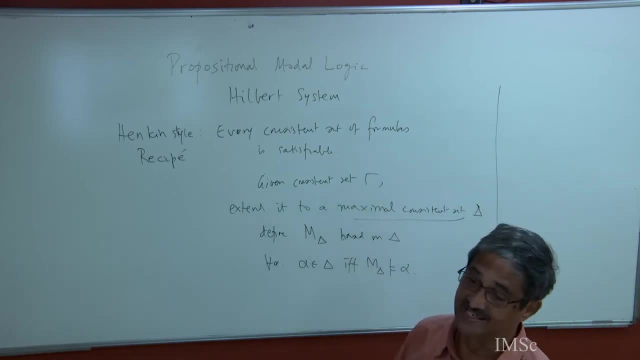 is what A set is consistent if you cannot derive a contradiction from it. So it is: gamma is consistent if there is no beta of the form. beta is derivable as well as negation. beta is derivable, right, and this is our idea of consistency. So it has something to do. 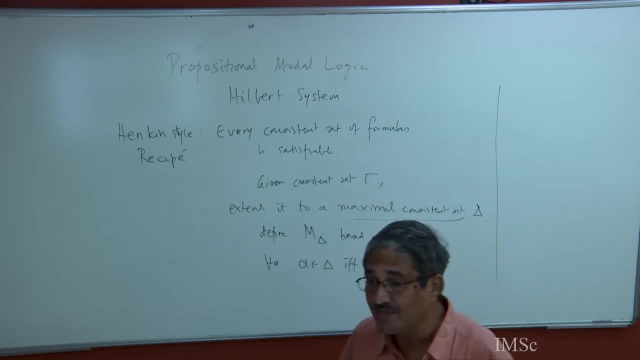 with derivations. and finally, when you do Now there is a problem. what is that? you take a model, set of model formulas extended to a maximal consistency. somehow you define the model m, delta. and then now, when you say: well, we do not have this notion of alpha being. 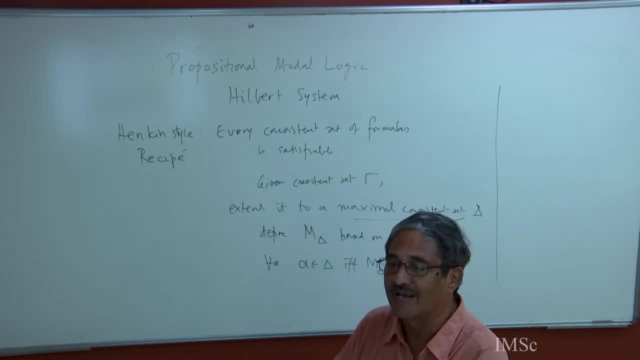 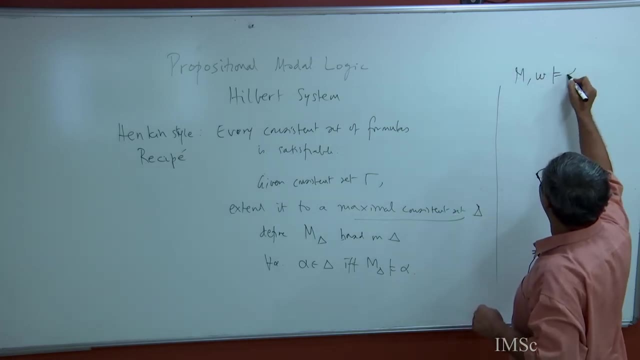 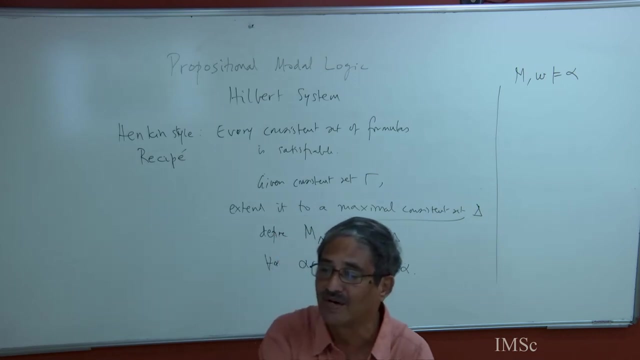 true in the model, because in model logic a formula is true at a world in the model. right, because we Have in the model m, at w you say alpha is true. right So this: because a proposition p can be true at world w 1 and false at world w 2. right, So it can be false, true in one. 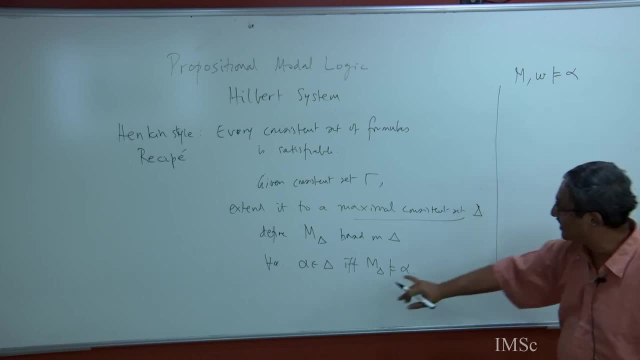 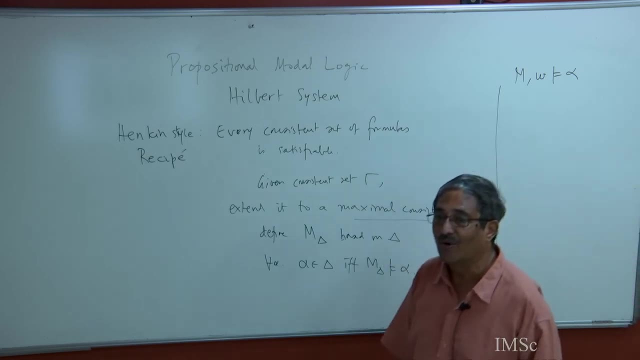 state and false. So it depends on where you are talking about. So you, on the left hand side, you have only a delta. on the left hand side, you want something extra. So how is your maximal consistent set Going to talk about different ones? and this is really the idea. Now look at the case. 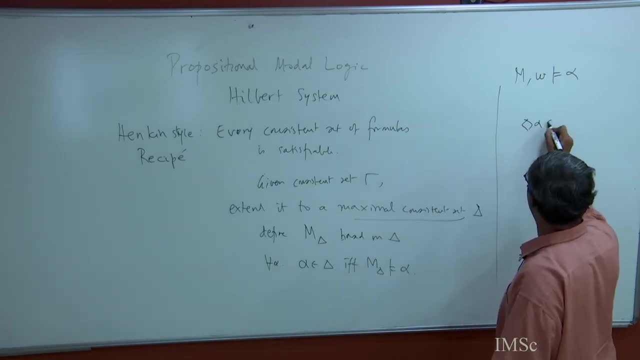 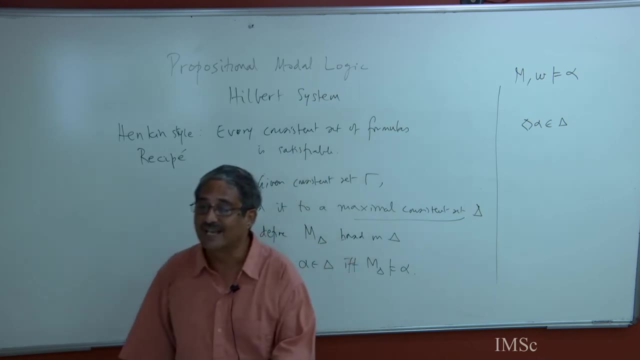 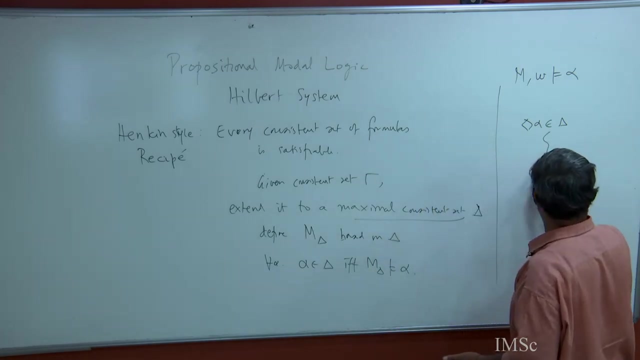 where you say, in particular, when you say diamond alpha belongs to delta, You will want to say, wherever you are, diamond alpha holds here right. and then that means that alpha must hold somewhere else right. So from there we will want to get to some alpha belonging. 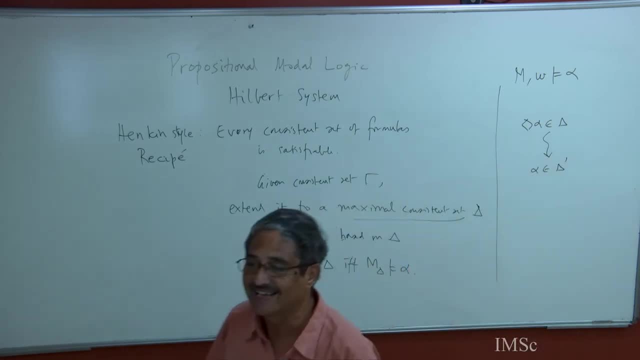 to some delta prime. that is clear, right? If diamond alpha is here, then you want alpha to. in general, if diamond alpha holds in a model at a w, it means you have to go to some other world where alpha holds. So you need to have not one maximal consistent set, but 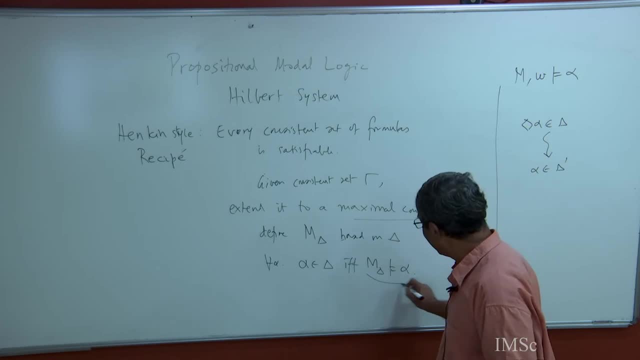 a whole lot of maximal consistent sets. So what would be your guess for what? we need a world here, right? Where are we going to get that state from, state or world or whatever you call it? right, You understand the question, right? The same idea can be used for what? 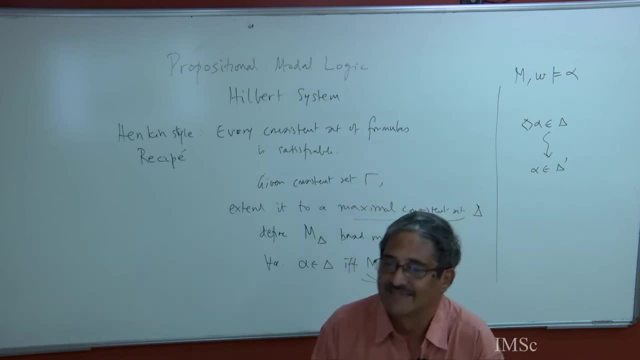 is called model logic. except that our main thing about Hanken style recipe is reduce membership to truth, right, Reduce membership, I mean sorry, Reduce truth in a model to membership in a set right Now. the problem is, you want this notion at different worlds, right You? 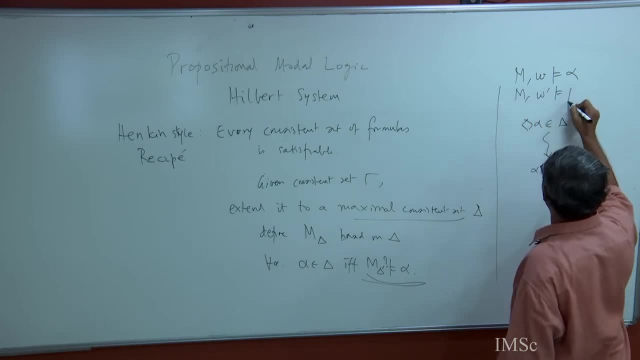 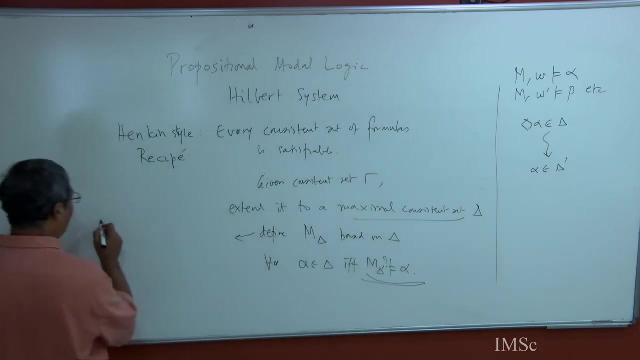 want so. So you cannot do this with just one maximal consistent set, but several maximal consistent sets. right, And we need to somehow define the model: m delta, b delta, what delta going to be Set of worlds, a relation and an accessibility relation and evaluation on it. this is what 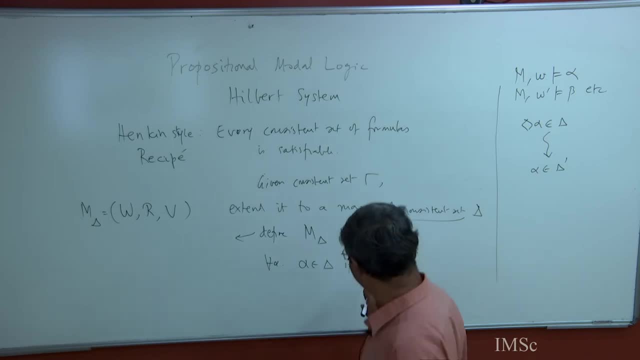 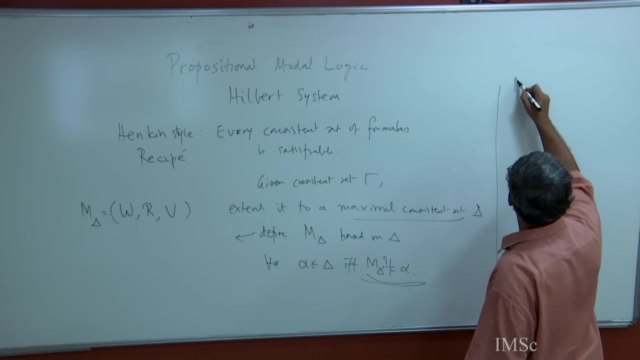 we want right? How are we going to define it? It is clear that we need different worlds and already the hint is here. because if, what is the definition of? let us look at what is the semantics of diamond alpha. Diamond alpha holds at a world w if and only if, there exists a w prime and alpha holds. 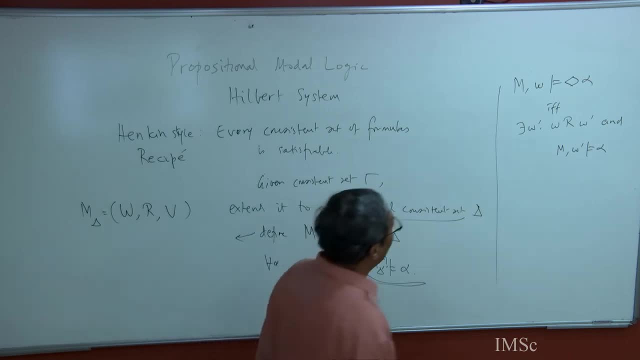 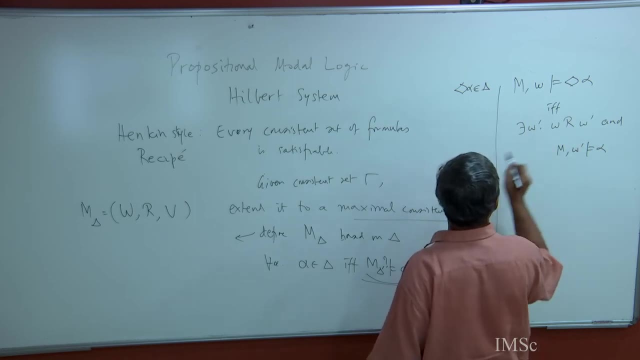 here, right So? So you want to start with diamond alpha belonging to delta and somehow say that there is a some w prime related, and somehow you want to get to alpha belonging to some delta prime, right So somewhere your w delta and w delta prime are to be related by r. this is what we want. 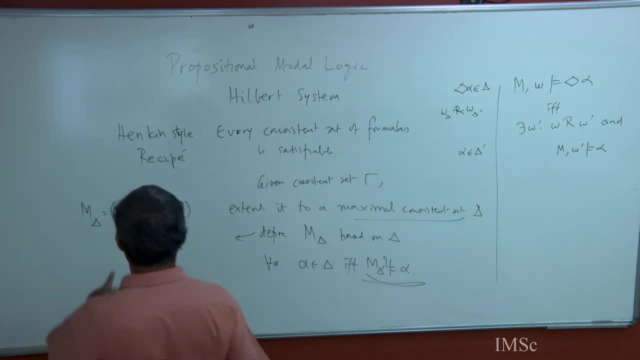 here. So how are we going to manufacture this set of worlds? right, we need to manufacture a set of worlds and tie them to delta, Right? So how are we going to manufacture this set of worlds? We have to give the set of worlds to delta somehow. 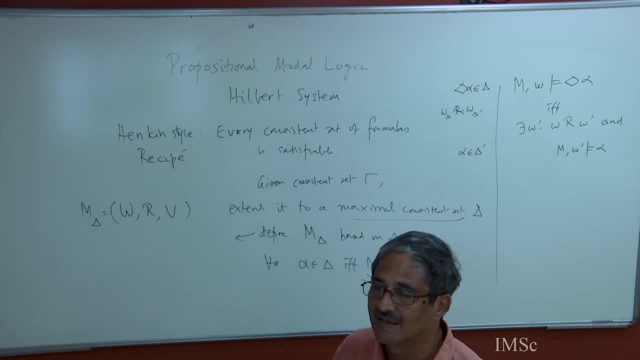 Any ideas for how we shall do it. Remember that here this delta is tied to this w. here this w has to be tied to delta somehow. right, How do we do that In propositional logic? right, that delta was the valuation. right, the said delta immediately. 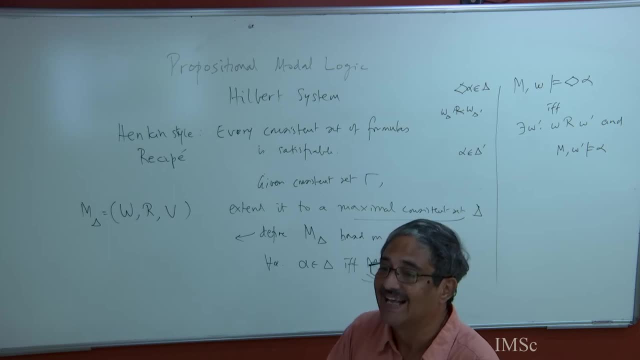 gives you the valuation. When you went to first order logic, that delta gave you the definition of how to interpret predicates, how to interpret pretty much everything after that right term, equality, everything right. So the delta is our reference. we have to base it on delta, right, or rather, but then. 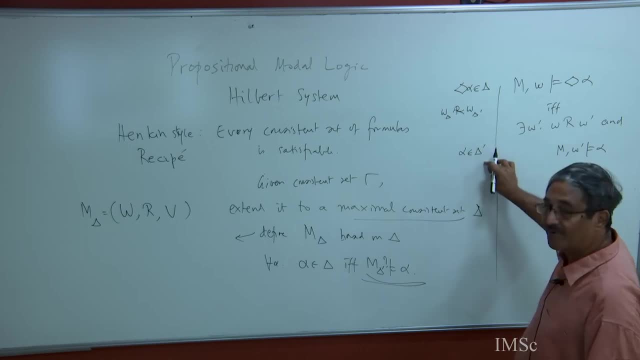 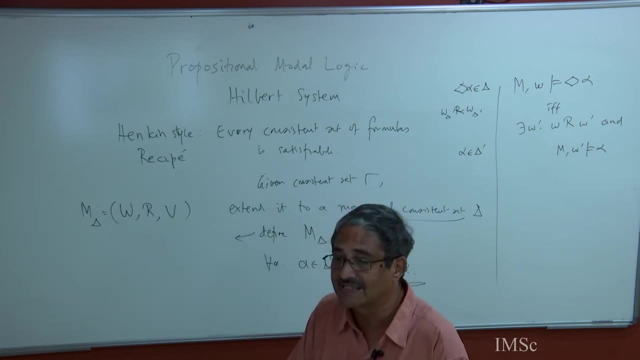 we realize that it is not just one delta that is important, but several delta prime. How many such so we need in our model? when we construct, we should be referring to not one maximal consistent set, but lots and lots of them. So how do we define W? What is the? 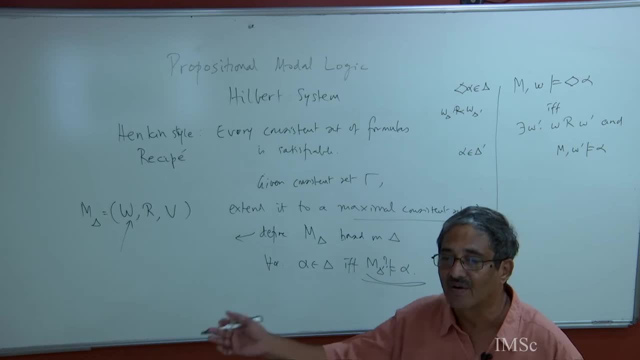 information available to consider all these different ones. Ok, let me remind you of what we did in the last class. In the last class, what were we doing To check for satisfiability? you given a formula alpha. How did the tableau construction go Down, close it right? you take a formula down close. 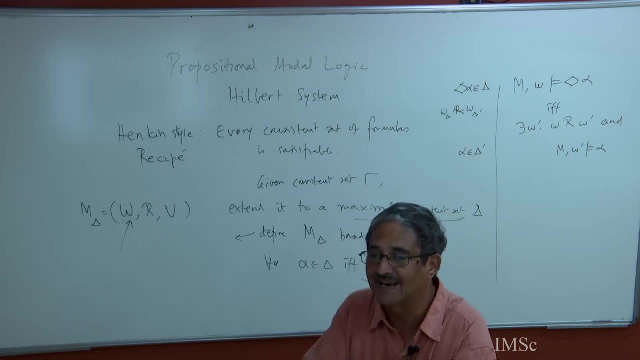 it That has a. so that is basically all those formulas that are consistent with that particular formula. That is all it means to say down close. no, Whatever is consistent, right. ok, Not maximal consistent, but some consistent subset of the set of sub formulas, right, And? 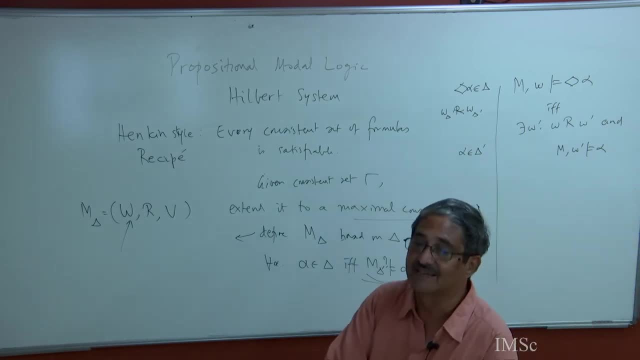 then, for diamond, what we do, We create an successor right and that successor again is labeled by some set of formulas. So in some sense, these maximal consistent sets will be labeling our words right, That is really what we are doing here. ok, So it is difficult to guess how to solve the problem. 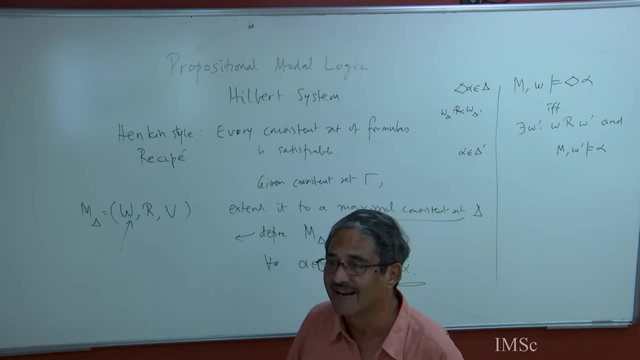 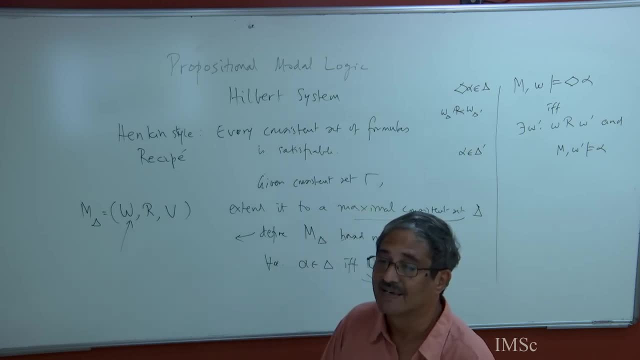 of domain right When we did completeness proof for first order logic. How do you come up with a domain? There is no other thing. Domain can be goats, it can be anything. Finally, what did we do? The domain was simply the set of all terms in the language right Use. 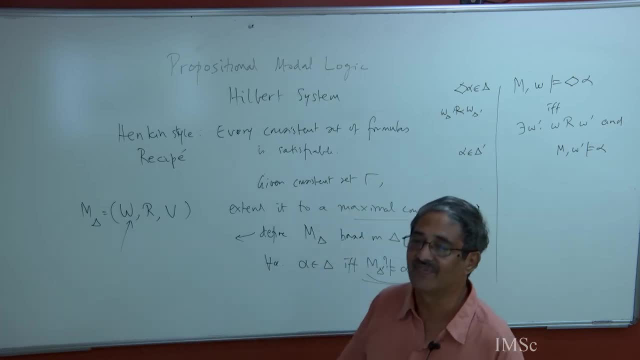 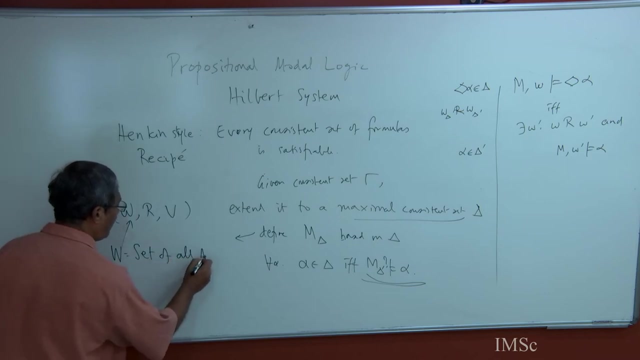 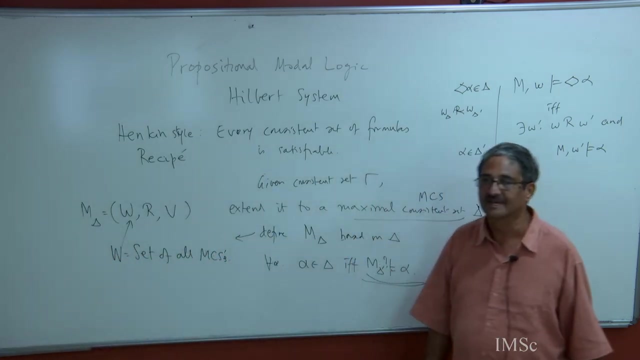 syntactic devices. that is all. The domain was simply the set of terms, right? So you have no other information on the set of words, So you should use whatever you have got, and so the simplest definition is: W is simply the set of. let me write. So what is the advantage of doing that? I will write it as what is. 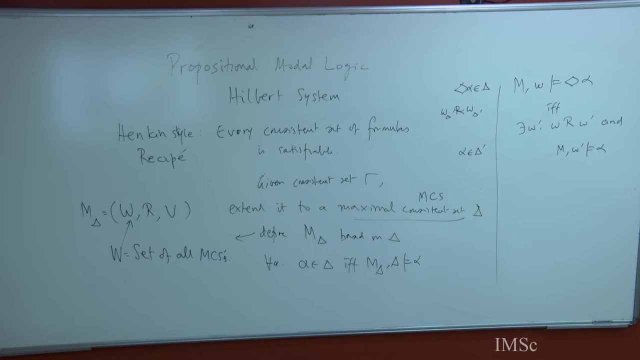 this some nonsense about. yeah, is what is the cardinality ofpools Delta? It is a count of. I can read Siddhar's lipsFlaps. 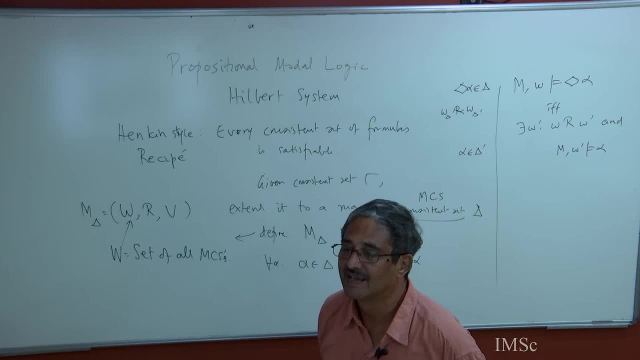 Yeah, even though he is on mute. You said count of the infinite set, Right? yeah, That is exactly what it is. So Delta is a countably infinite set. So now, what is the Smart? It is a count. So Delta is count of the in. Yeah, It is a countably infinite set. So now, what is the 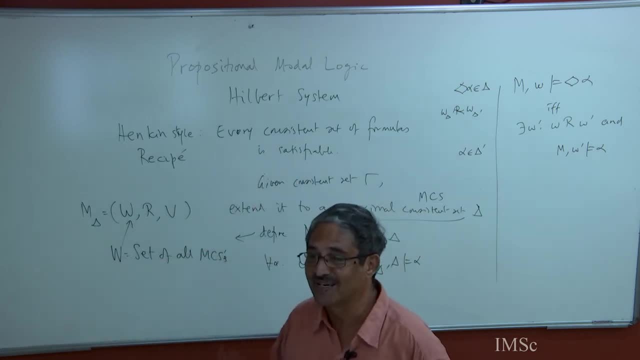 card of this. It is a set of all maximal consistency. What cardinality is the continuum, the set of katri, rival, consistent set, reason: right, We did the change of the فيn, the weightI was지도15 it for the way which makes plainness. 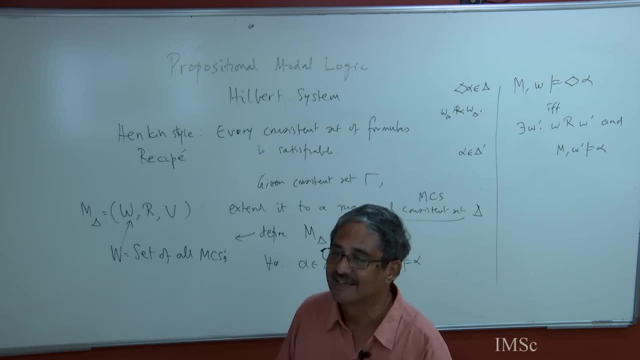 right, of course it is right. set of all, such will be the cardinality. who cares, right? what do we care? you are not afraid of uncountably many worlds, right? so that is easy. So now, when I want to move to alpha and delta prime, I just have to say alpha belongs to 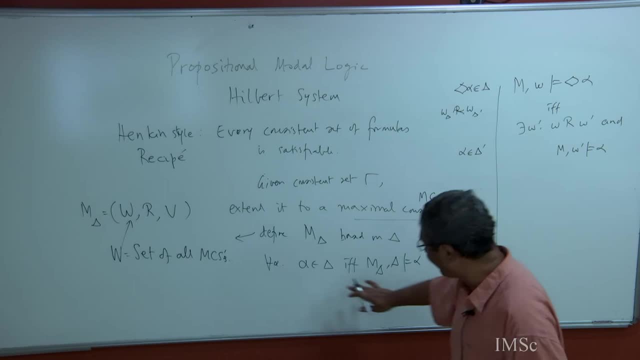 delta prime, again right. so it gives a uniform way of handling this. My truth lemma, the way to prove is exactly. So this already tells me what should be the valuation. valuation is easy, right. valuation is a map from w to 2 to the p. 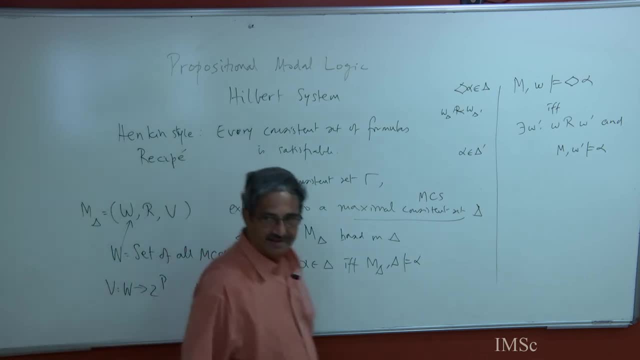 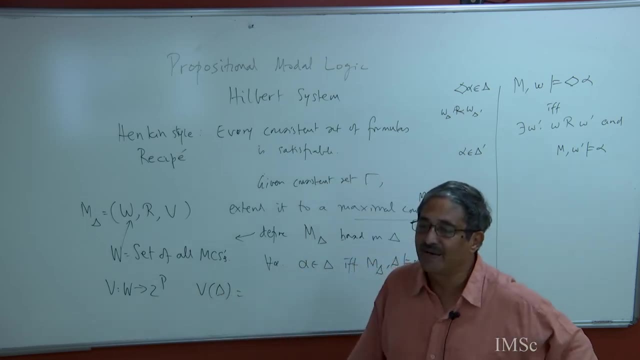 So what is Vf delta? delta is a world. I have to say, what is the valuation there? right, what should be Vf delta? which proposition should be true in at that world? you have no option, You have to consult delta, right. 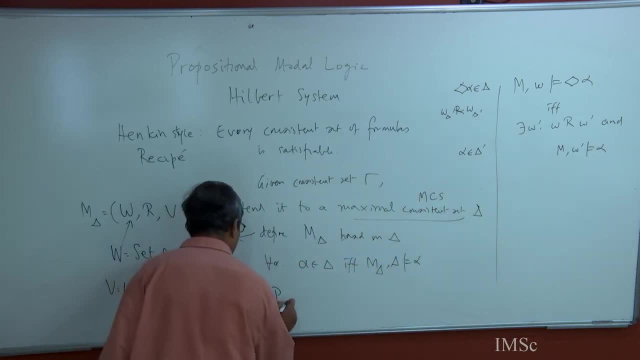 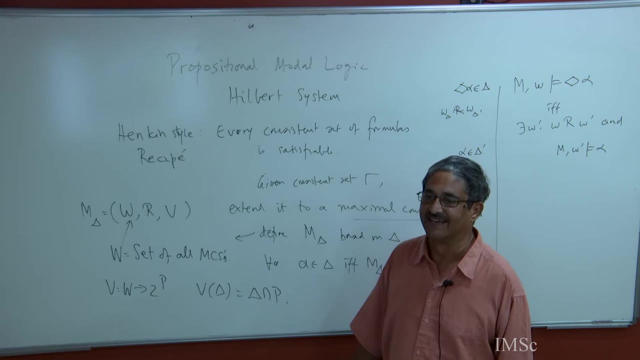 So this is just right. I hope it is clear. delta, intersection p in the sense that a proposition is true at that world delta: if it is there in it, it is false. if it is not there in it, it is a maximal consistent set. remember so for every proposition, in particular it. 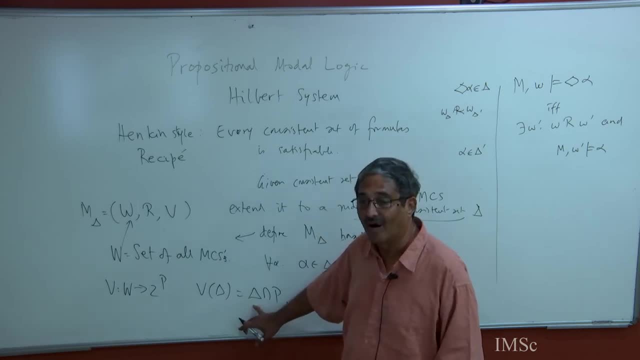 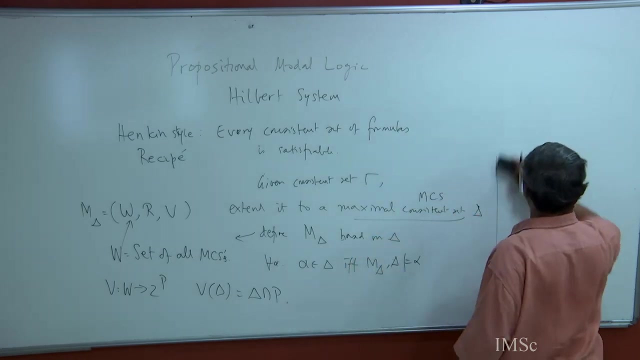 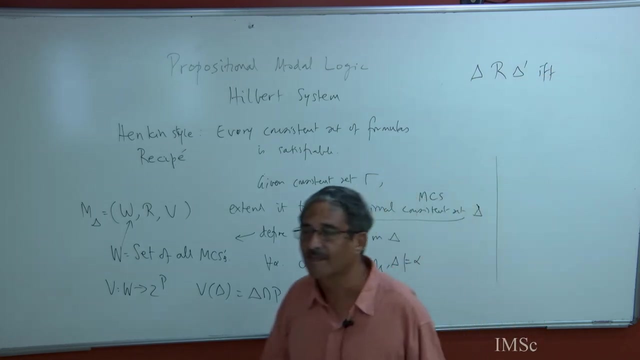 is going to put that proposition p in it or not right and not both. So it is consistent. and for every proposition it makes a decision. So you take this and you get a map, no problem. What about the relation between? now we need to define, we have to define the relation. 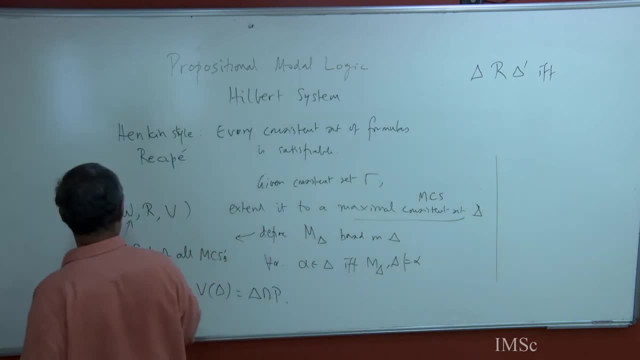 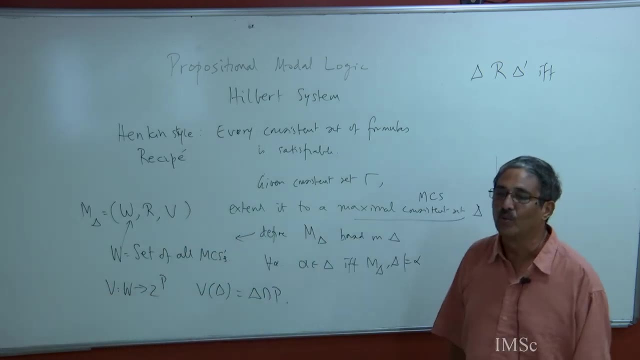 between these, right, I have to call it R, whatever it is okay. yeah, what is the relation between two maximal consistent sets? because you have to define this right to define a model Once again, look back to what was the. how did we do the tableau construction when I 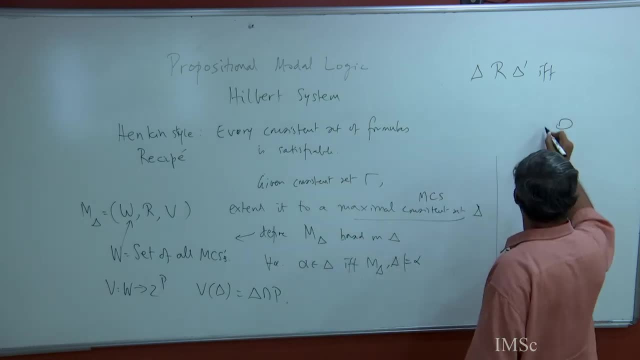 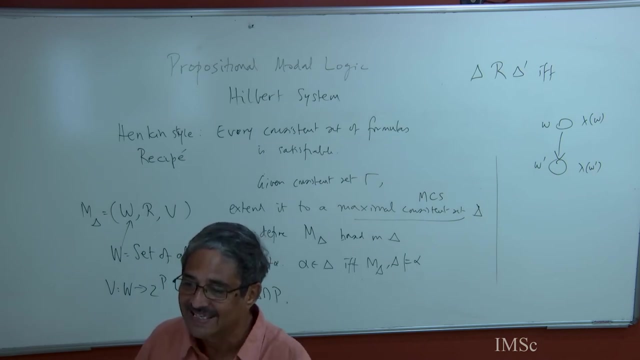 have a w and a w prime right. and then I had lambda of w and q, Lambda of w prime. these were the sets of sub formulas. true there, but what is the condition that we maintained? Whenever you add a child, what is the condition that you need to maintain? 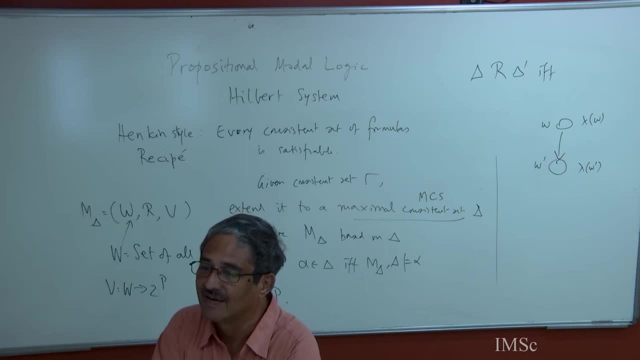 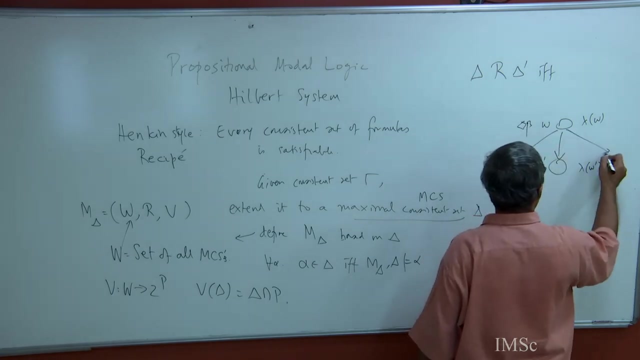 Why do you add a child? no, In a tableau construction I want to fulfill Right For a diamond formula right. So if diamond beta is there, I have to put in beta. but then there is what is the coherence? 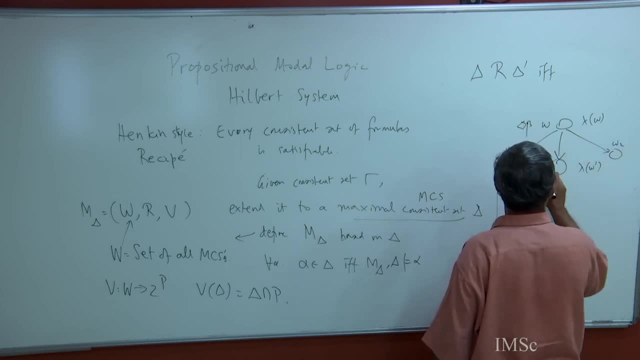 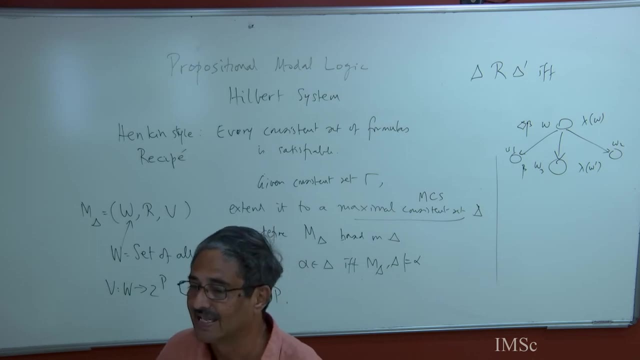 condition. Let us say this is w3. For all the children. what is it that I need to maintain If diamond beta is there? of course I am adding a child just for that purpose. I need to, But there is some other condition that is important. no, what is that? 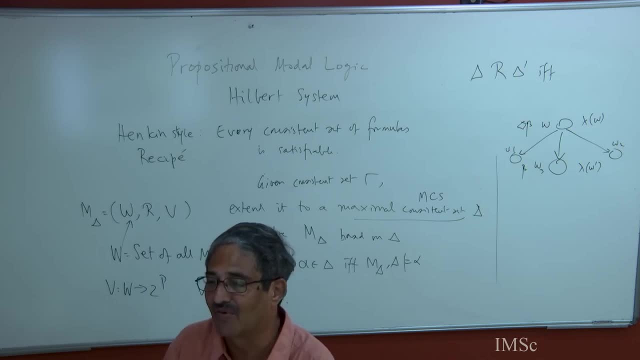 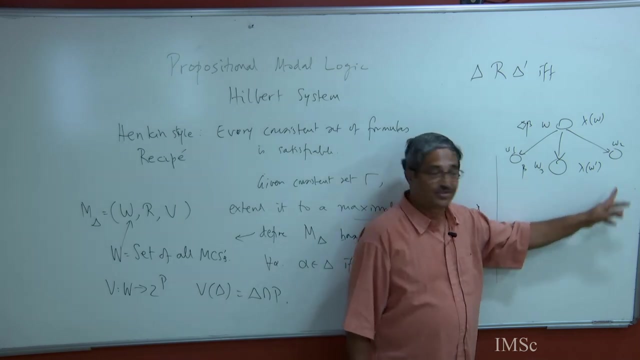 In modal logic there are two kinds of modal formulas. right, Diamond is the existential formula. what is the universal formula, Box? So if this fellow says box alpha, you must make sure that is there in all of them, right? So if box alpha is there, every child must have alpha. 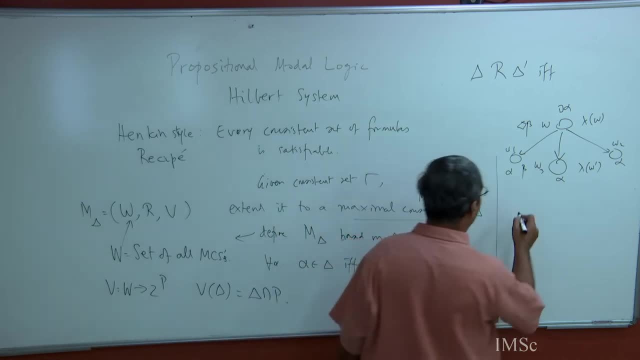 So we maintain the condition that on in the tree whenever you have an age of this kind, this implies box alpha belongs to lambda of w, then alpha belongs to lambda of w, prime right. This is the condition that we maintain, right. 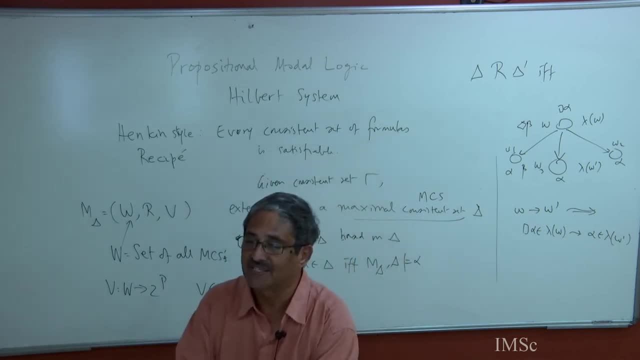 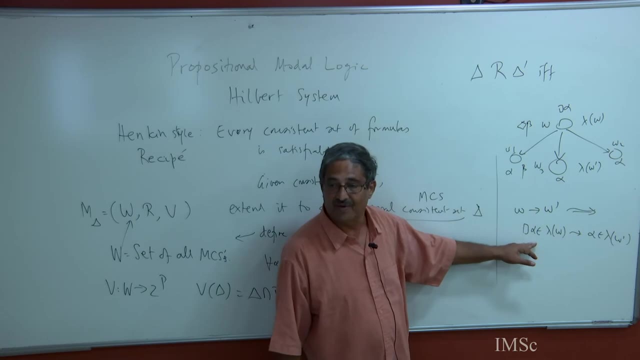 If you are going to reduce satisfaction of formulas to truth condition, if box alpha holds at this world, I want that means box alpha belongs to this- right then I have to make sure that alpha holds at this This world, which means alpha must belong to this. 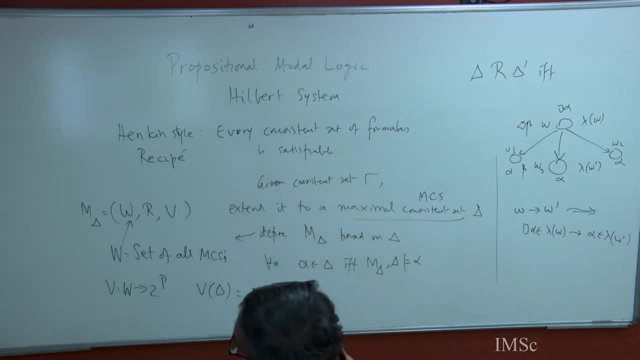 So, therefore, do you understand what I am saying? So the relationship that we need to define, you really have no choice. a or b. if, and only if, for every formula alpha box, alpha belongs to a, then alpha belongs to b. 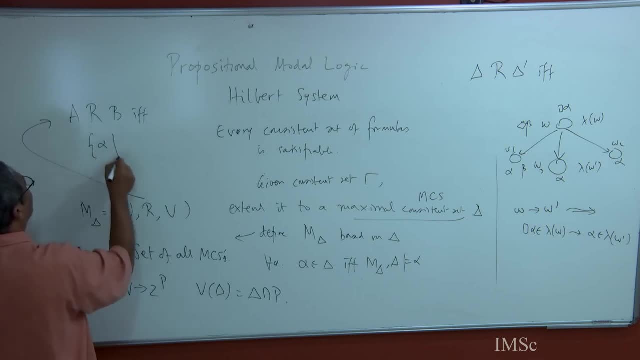 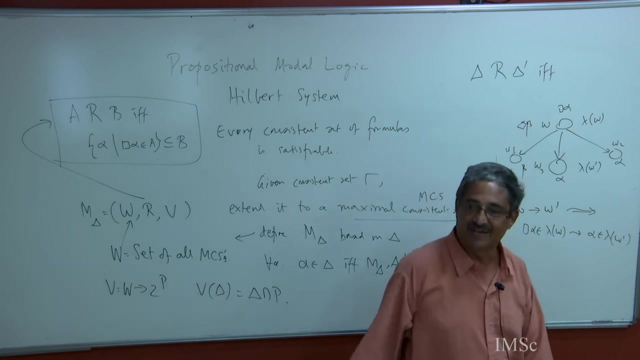 So the way I would write it is: the set of all alpha belongs to a to b. Okay, So we get the balance here right, such that box alpha belongs to A is contained in B. That is the coherence relation. This is exactly what we were doing earlier. Now, that was a condition that we had earlier saying. 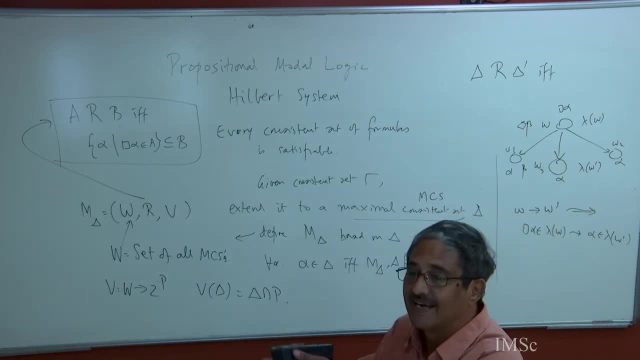 I am building the tree and if I put an edge, I maintain this condition. Here I am defining it to be if and only if, Because I am defining the relation. So it is going to relate all kinds of maximal consistent sets to all kinds of them. I do not care, I have no problem. 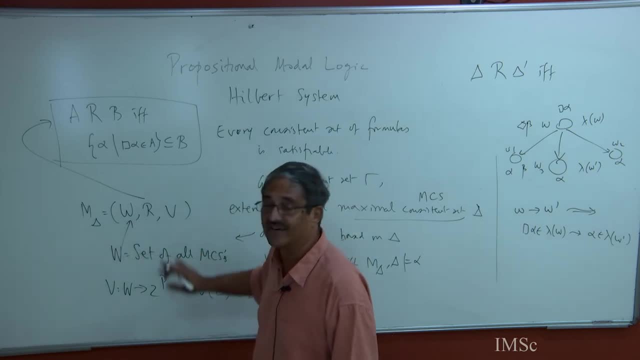 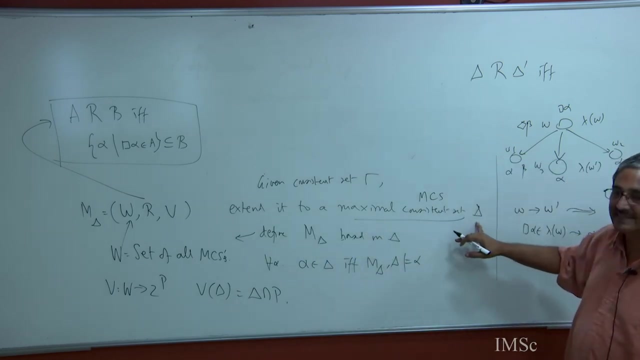 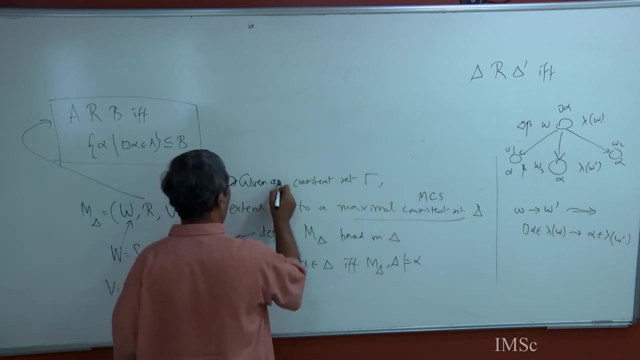 What is my problem? I just need a definition. Now I have got a definition. I started so I was given a consistent set gamma, given a consistent set gamma extended to a maximal consistent set. I know how to do this. So this is true for every given any consistent set gamma We can. 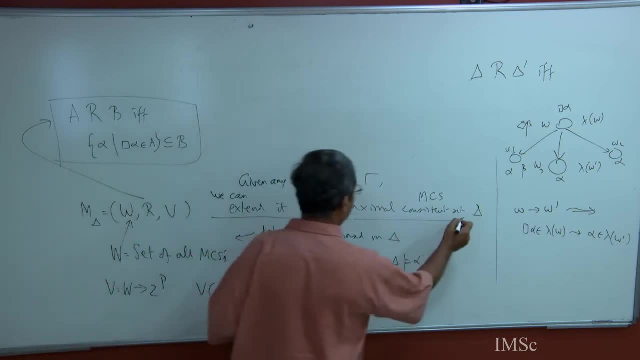 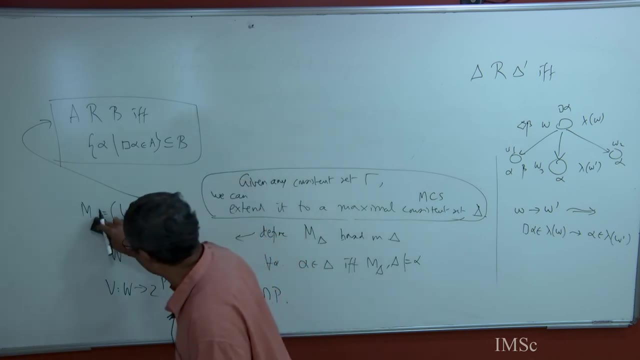 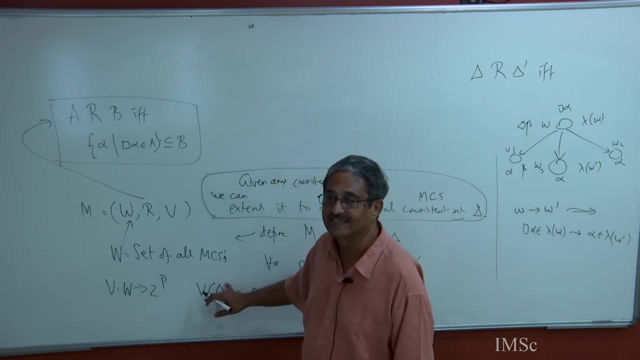 extend it to a maximal consistent delta. So this we know. Now we define the model based on not 1.. What is the model now? The model is simply consider the set of all maximal consistent sets, Define accessibility, relation defined this way, and evaluation defined this way. So let me put it all in. 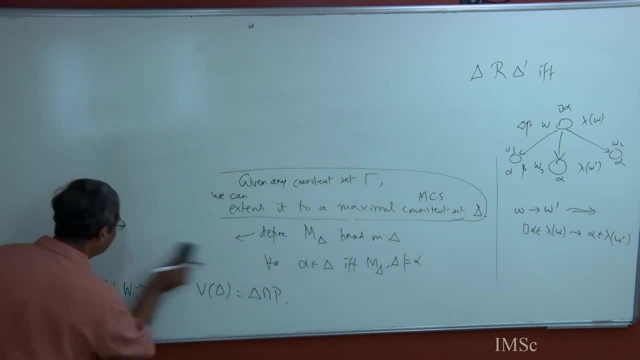 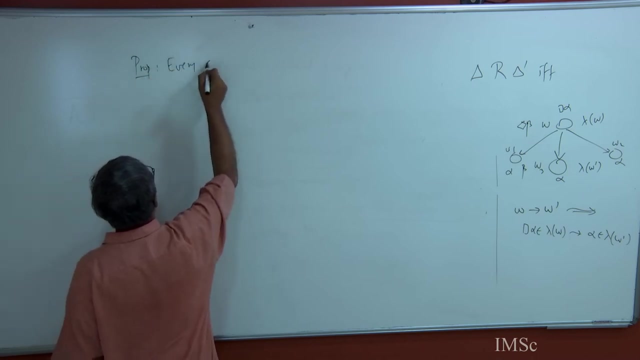 one place. So we can see now I hope the idea is clear. So this is the how the completeness proof goes. So first proposition: every consistent set gamma VS extra total. Now we want to consider the for each number set gamma. we. 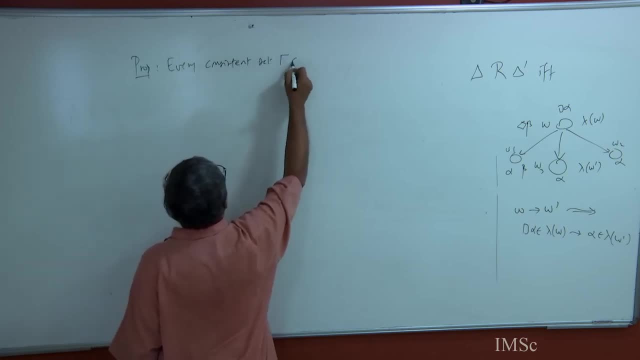 have given the complex offset somewhere to s. A maximum offset on a exponential set delta becomes n. This means that the Causバp between certain values, which can be true for real wherever we want toeffer Come to. so some bank, let us evaluate a minha. we will break this here. 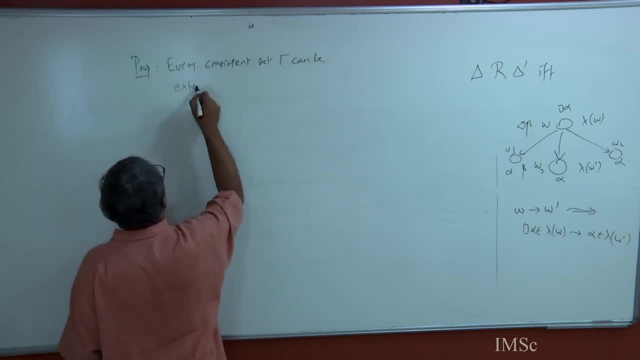 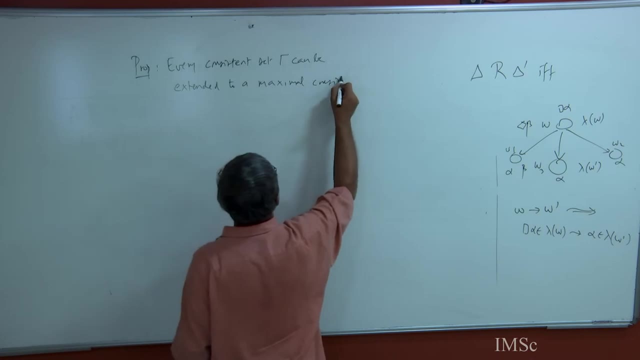 can be extended to a, and this is something we can make use of at every point. right, And remember that this proof follows from the fact that, whatever axiom system I am going to build, I am going to put propositional axioms into it. right, because this thing? 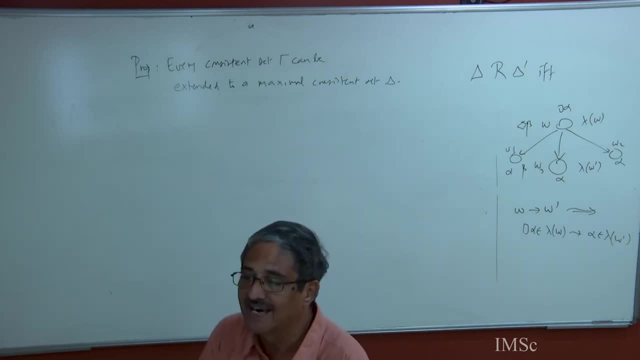 the proof of this depends only on propositional reasoning right. It does not matter whether I am talking about modal formulas or whatever right, because, for instance, this is a tautology. These are all tautologies of propositional calculus. Even though they are modal formulas, they are substitutional instances of propositional 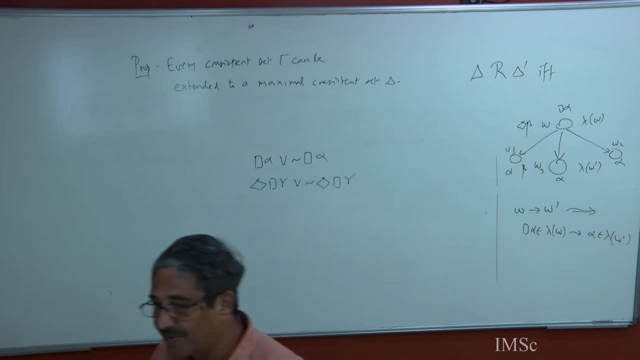 validities and that is all that we used throughout, right? So that part is all should go through then. So what I define just now is called a canonical model. okay, This is the canonical model. Why do you call it something like that? 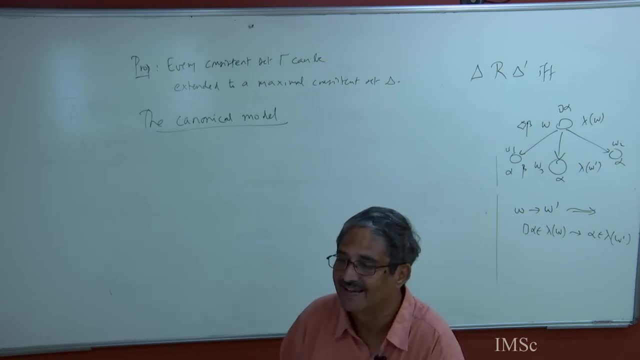 It is because it is not dependent on any particular formula right. It just depends on the logic right. Once you have the axiom system, once you have derivations and consistencies, When consistency is given, the canonical model is defined. Is this clear? 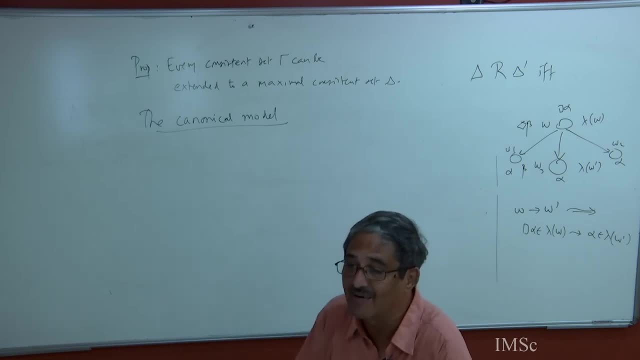 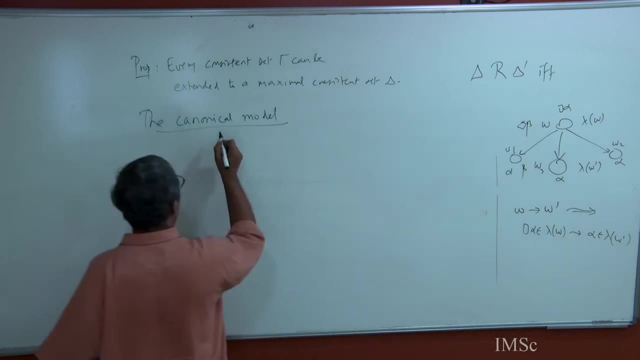 Remember, it is not dependent on any particular set you have given or anything, right? So that is why it is called canonical, in this sense. So the canonical model gamma. so this is associated with the system for your system H. Actually it is called system K because for Kripke, Sol, Kripke was the one for system K, So what? 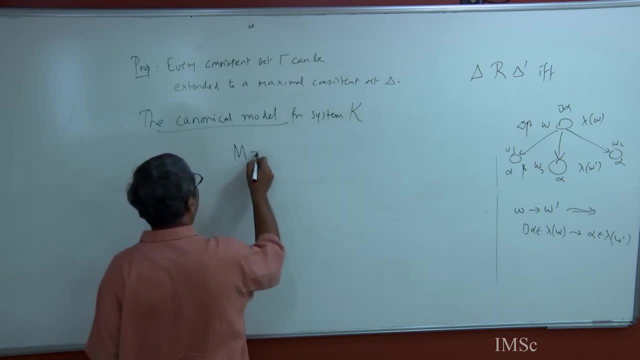 is the canonical model for system K. W is the set of all maximal consistent sets and MCS stands for maximal consistent sets And R is defined by. so let me just use A, like last time. I did A, R, B if, and only if. 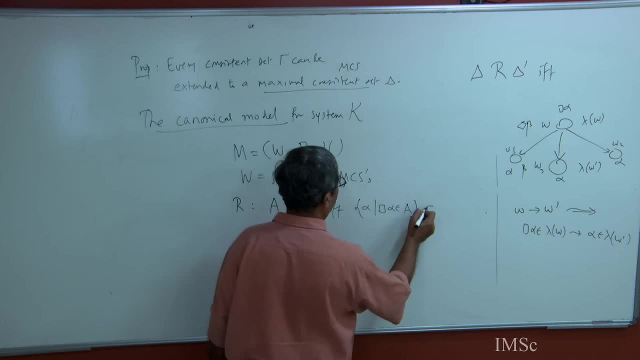 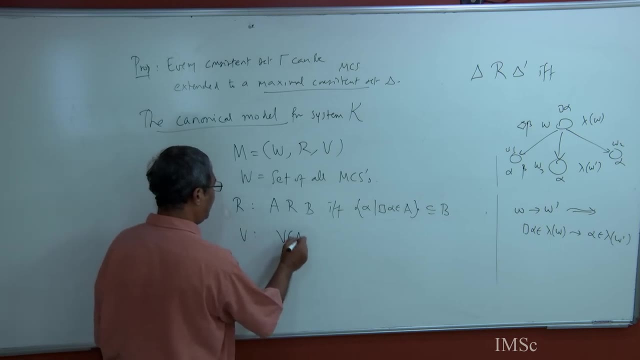 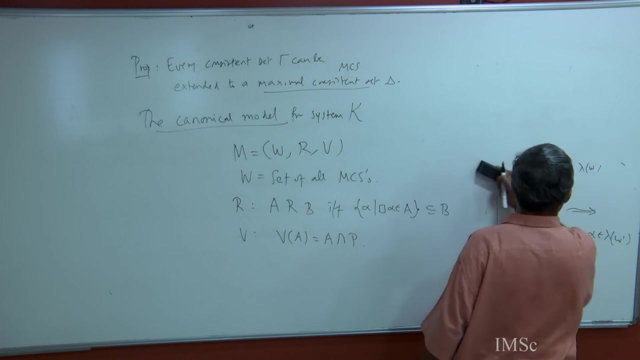 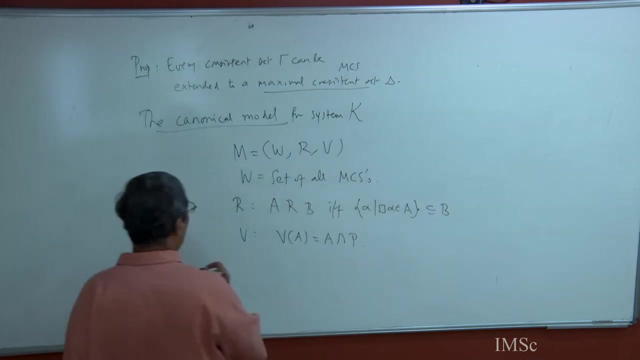 set of all alphas, such that valuation is defined by V of A equals A intersection B. Okay, And that is it. So now, here you have this. Yes, So for completeness, it suffices to prove that for all alpha, for all maximal consistent, 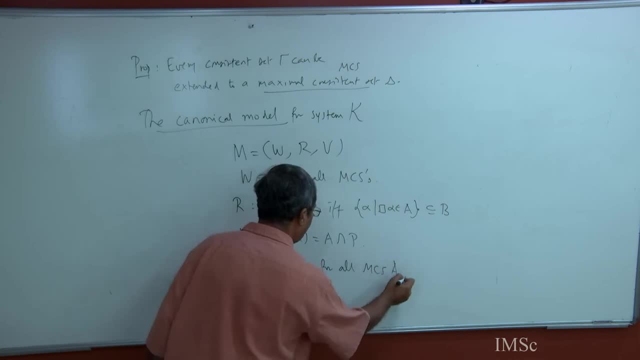 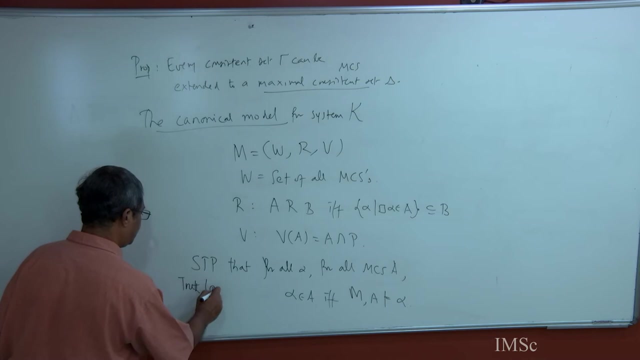 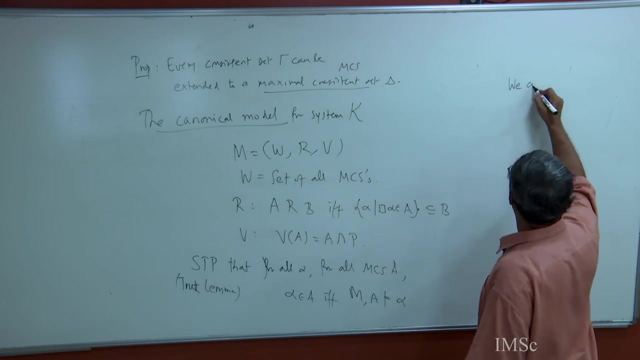 sets MCSA alpha belongs to A if and only if. right, this is the truth lemma. Why is this sufficient? We are given consistent set MCSA, So gamma 0, let delta 0 be. oh, I have called it AB now, so let me call it. let A naught. 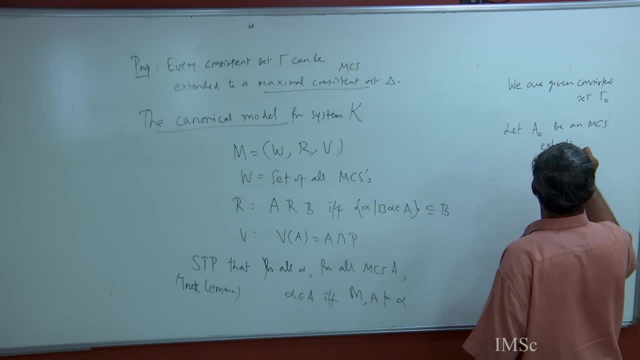 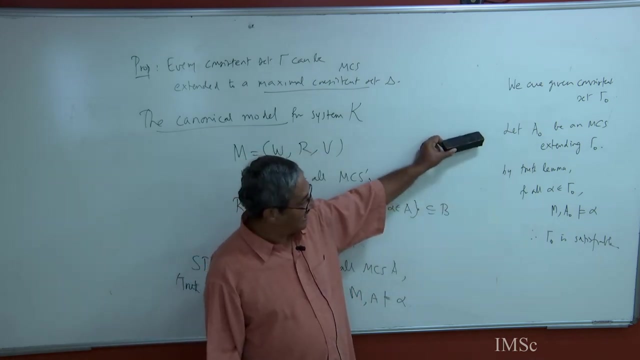 be an MCS extending gamma 0. By truth lemma. Okay, For all alpha belonging to gamma 0,. therefore, this is exactly our original right. Once you have an MCS extending it by truth lemma, you know that for all alpha in A 0,. 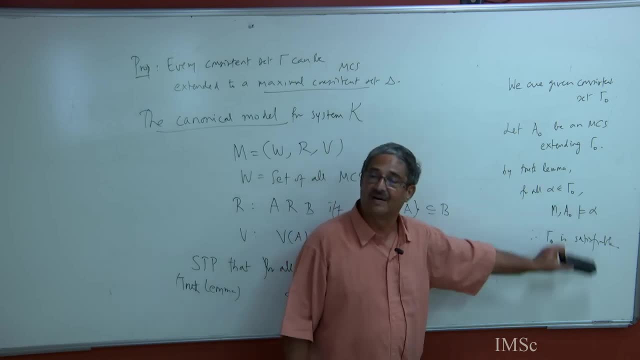 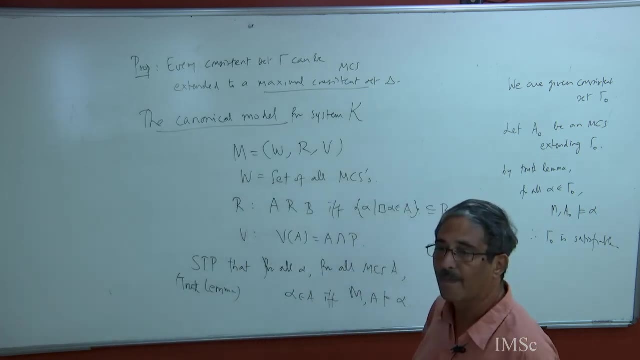 so, in particular, for all alpha in gamma 0.. This particular alpha is true at this particular world A 0 that we have. so this is all we need to do. Yeah, Is this clear? So we need to prove this truth, lemma. and that is, of course, the heart of all completeness. 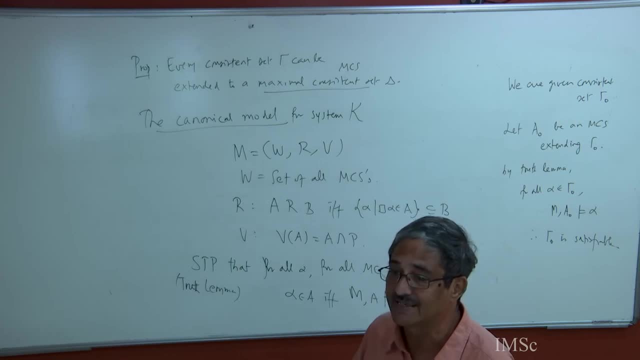 arguments, and let us so remember: so far, we still have no axioms, no inference rules. It is only in the matter of proving the truth, lemma, that you discover what axioms you need. right, And that is how it should be. 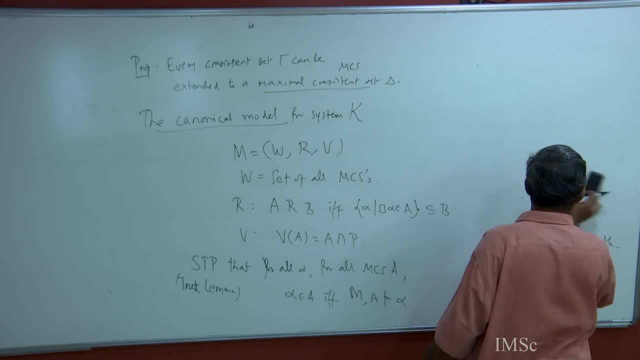 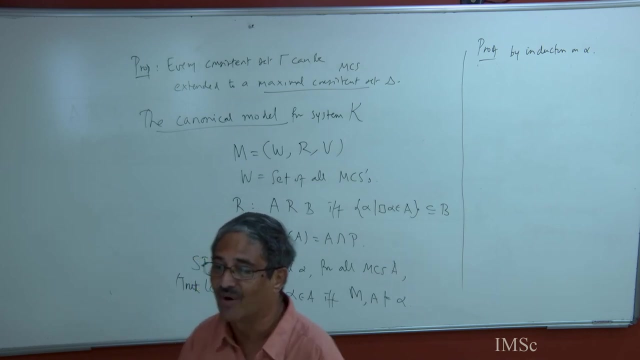 So let us go over to the proof of the truth, lemma, and you will see that everything goes through as you would expect. there are no deep surprises. it is a matter of just coming up with the axioms. Yeah, So proof by induction on alpha, by which we mean it is like what we did in the labeling. 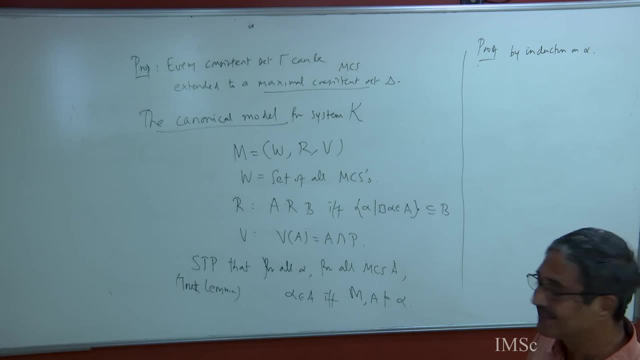 algorithm right. Checking for truth. Yeah, We have a formula in a model in this thing Similar to: first you look at alpha for all the sets right, Then you look at negation alpha for all the sets alpha or beta. 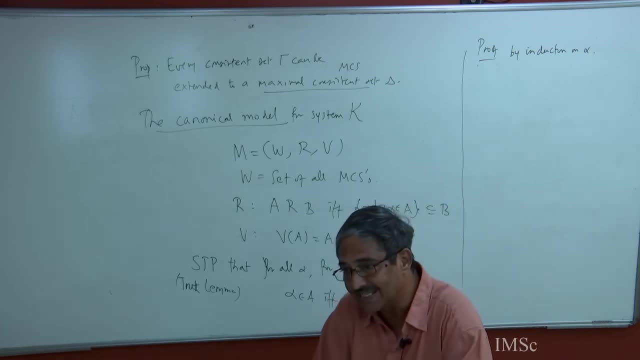 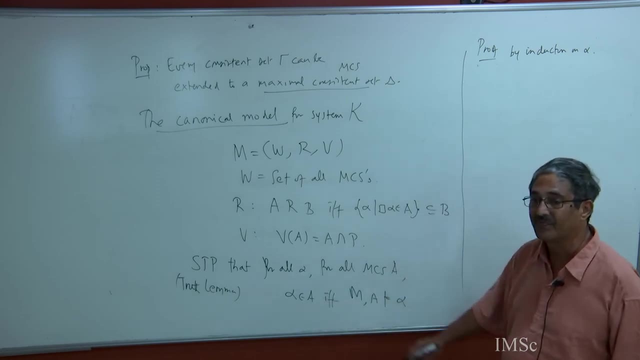 So any time you look at alpha, all the smaller formulas have already been decided in all the sets. that is what it means, right? This is, we will give you this for all A right. ok, so that is useful. 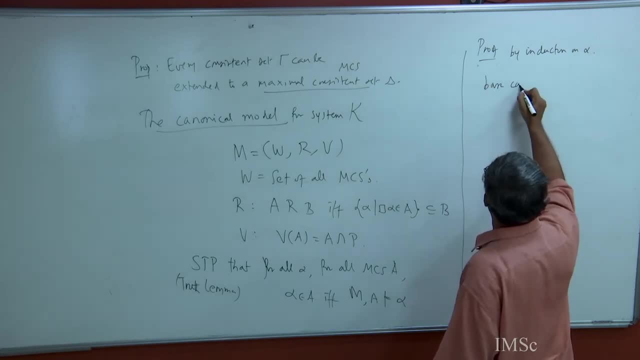 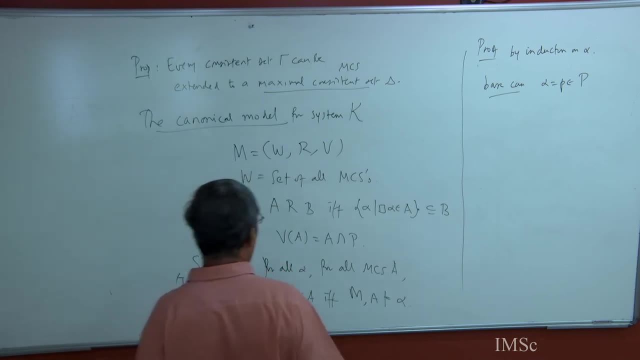 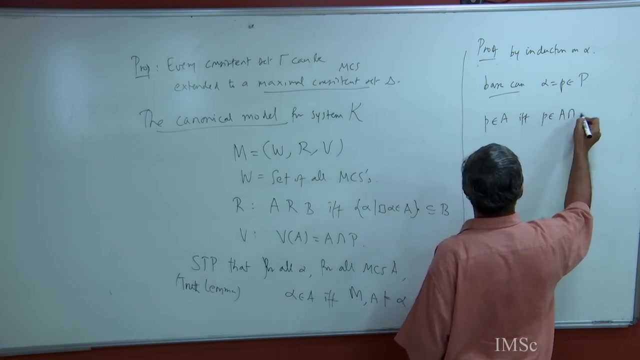 So base case alpha is a proposition. Ok, Some atomic proposition. Then what do we know? P belongs to A if, and only if, P belongs to A intersection, A intersection P if, and only if, M comma A satisfies P right. 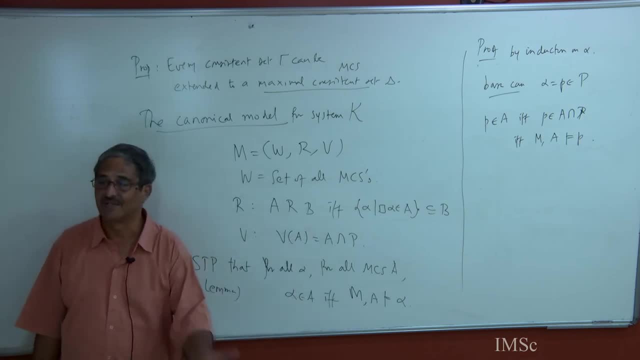 This is exactly what you, this is how we have defined it, So there is no other. P belongs to A is the same. it is a proposition. right? we are starting with P in P, So it belongs to A if, and only if, it is there in the intersection, if, and only if, the valuation 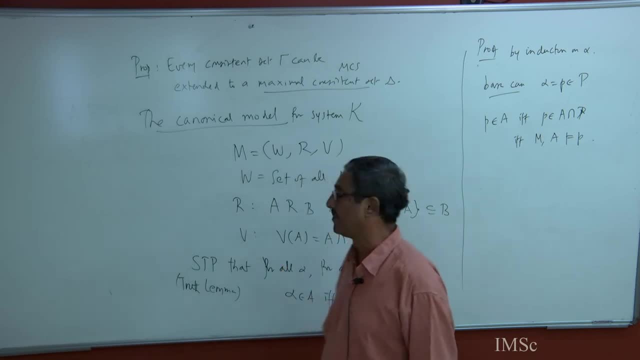 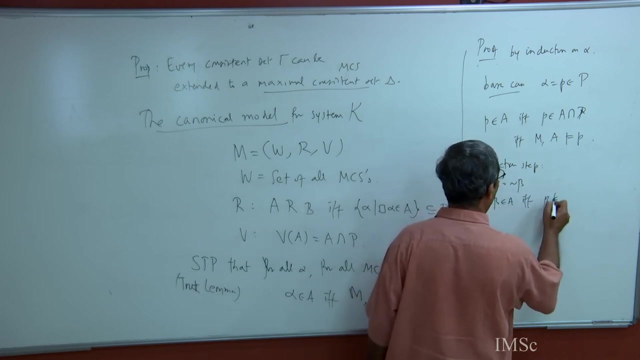 makes it true if, and only if, it is true in the model. So induction step, The Boolean cases are routine. right alpha is of the form not beta. not beta belongs to A if, and only if, beta does not belong to A. 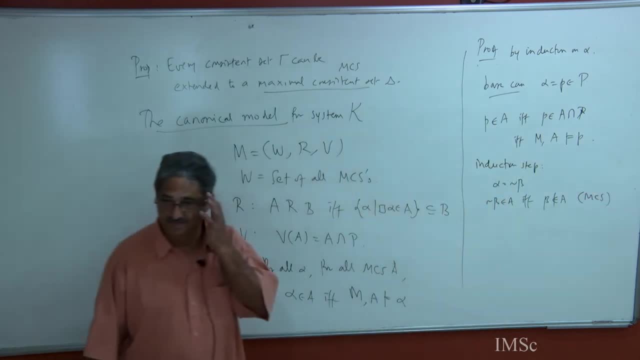 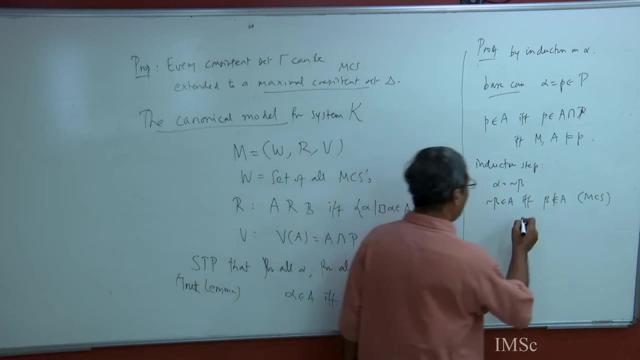 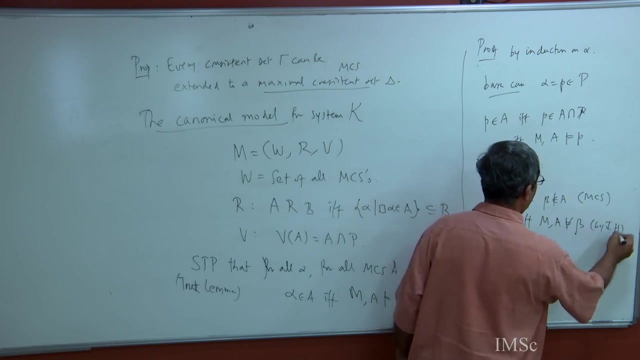 And this is because it is a maximal consistency, consistent and complete right. So if not beta is there, then beta is if and only if. beta does not belong to A, if and only if. M, A by induction hypothesis, if and only if. by semantics, yeah, I mean this. 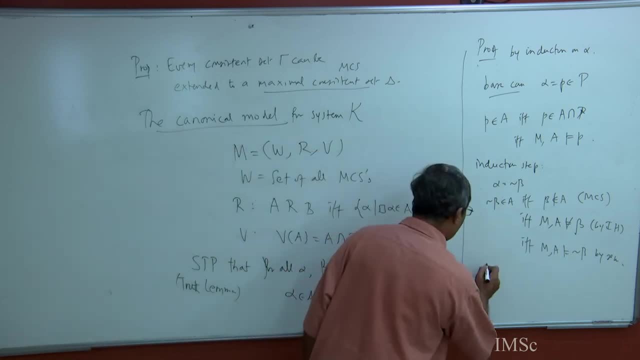 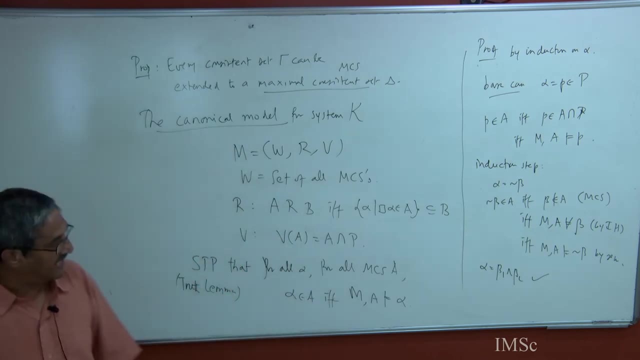 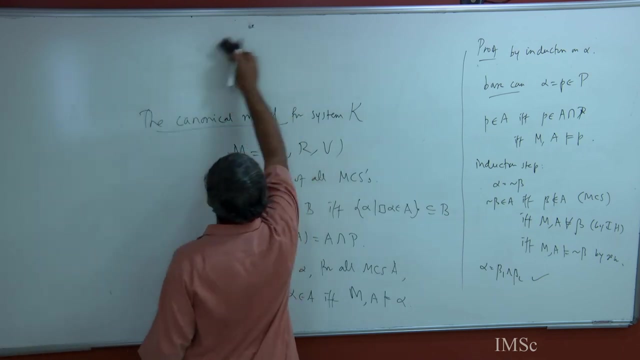 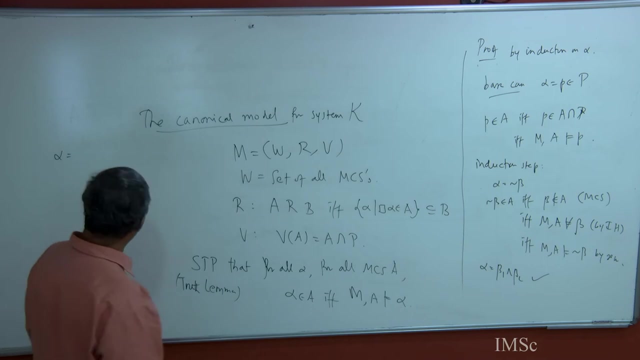 is all propositional reasoning, Similarly. Similarly, alpha is of the form beta 1, let us take the model case. So that is the interesting one. So one part is again straightforward: If alpha is of the form box beta, or let me try this way, yeah, 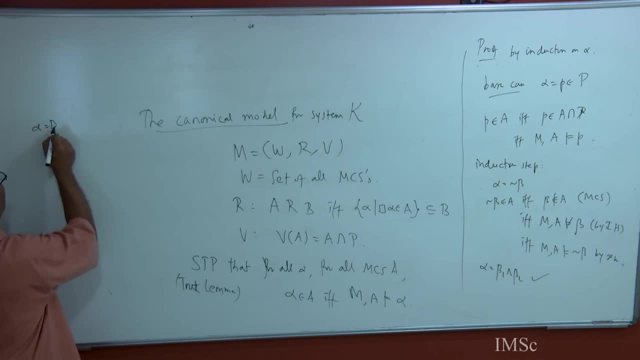 Suppose box beta belongs to. so alpha is of the form box beta. Suppose box beta belongs to A. to prove M: A satisfies that is box beta. is true in the model at A. ok, So consider B such that A is related to B. 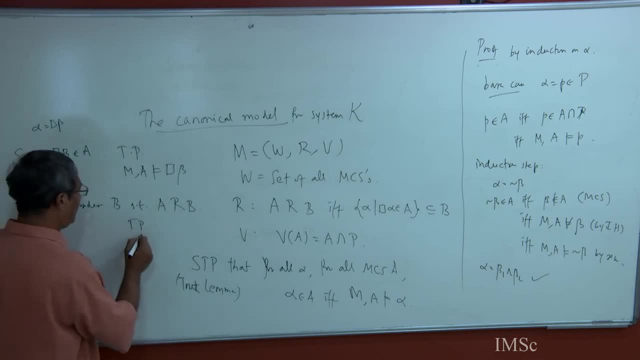 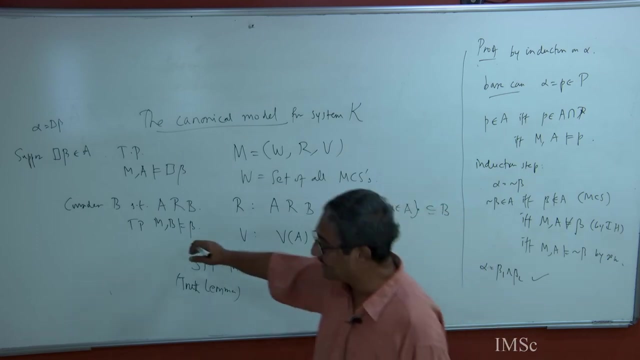 To prove M B satisfies beta right. that is what it means. How do you show that box beta is true at a world A? Look at all the successors and show that. take an arbitrary successor and show that beta is true in it. 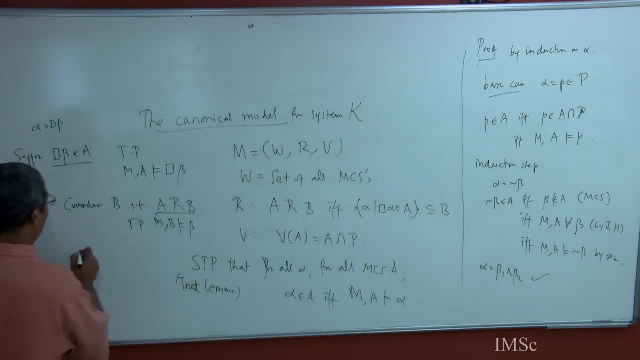 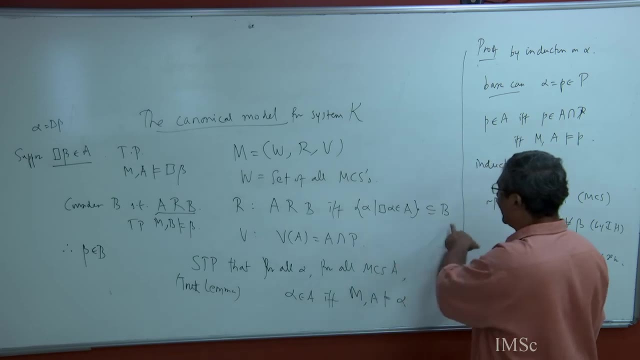 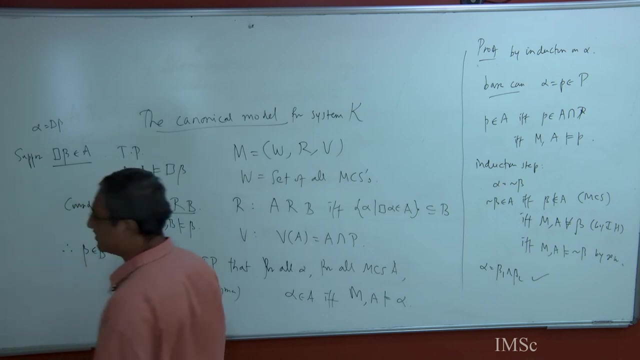 But box beta belongs to A and A is related to B. therefore beta belongs to B. This is the definition. Ok, So box beta belongs to A, then beta belongs to B and then by induction hypothesis, we are done. Still no need for axioms, inference rules, and this is the point I am making right. 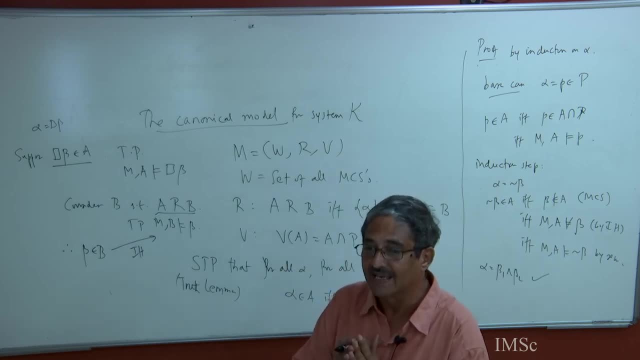 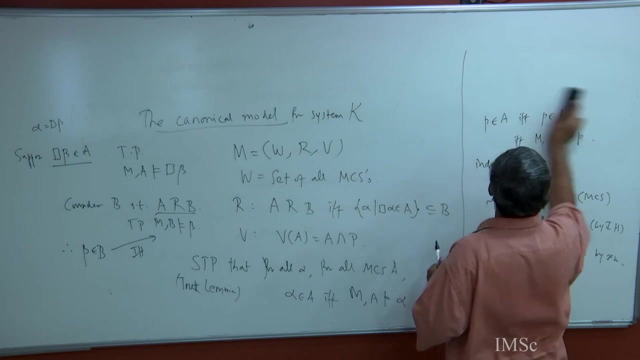 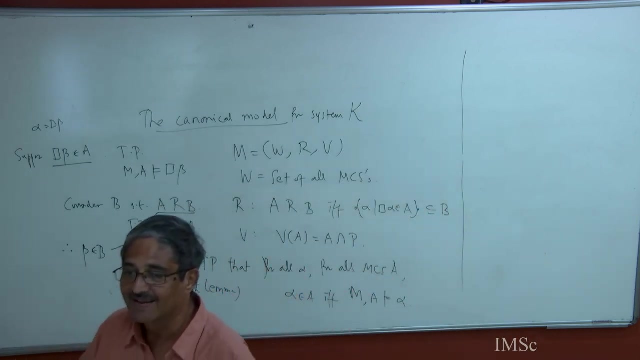 Everywhere we have just routinely lifted propositional reasoning, and so the only place there is one step in the induction argument, and that is what forces the axioms and inference rules. What is that? Well, So let us see And remember: this is exactly what happened when we did the decision procedure as well. 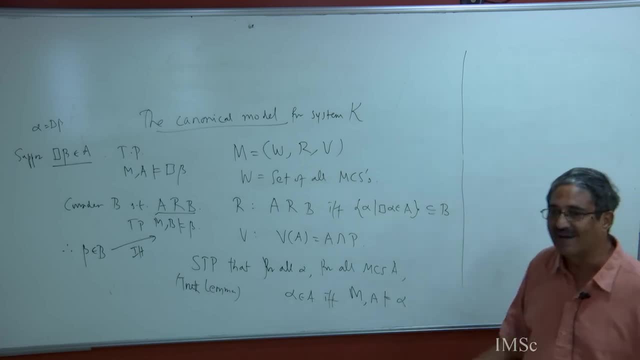 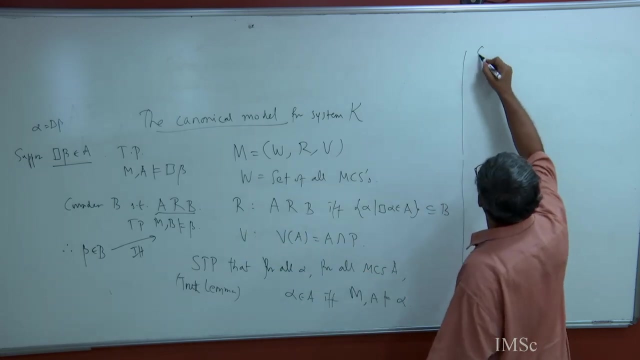 There is no reason to build up an elaborate model at all. Well, you need worlds, But why do you need more than one world Only when you have diamond formulas right, and that is exactly what we are going to get to. So suppose, 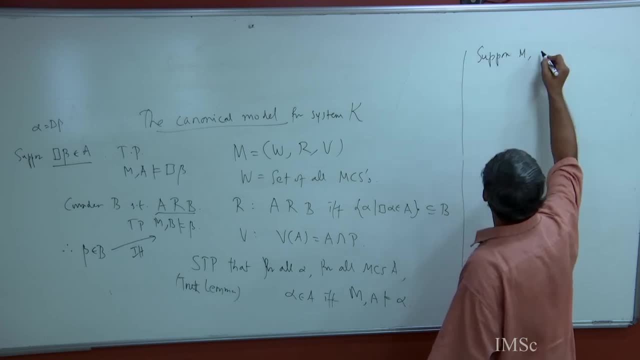 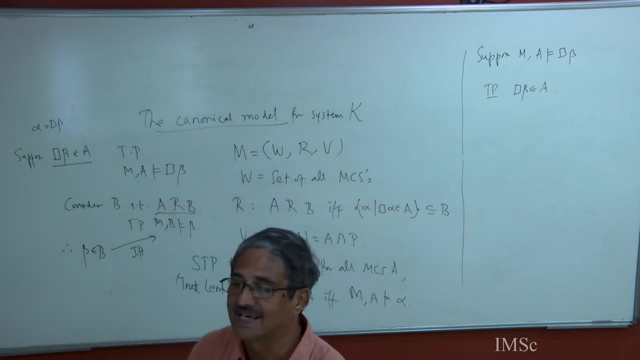 Ok, Ok, Ok, Ok, Ok. So you can see that you have this. ema satisfies box beta. to prove: box beta belongs to A. How do you ever prove that a maximal consistent set has a formula? Well, I mean, we have no particular way. 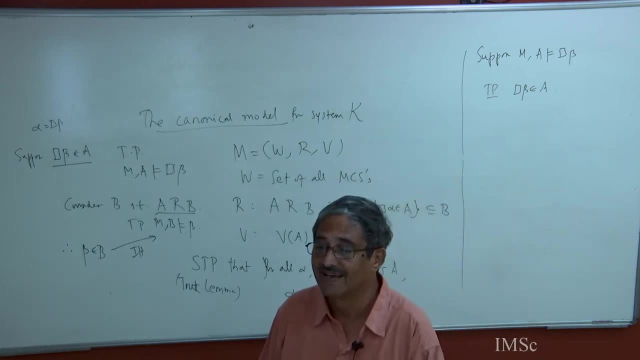 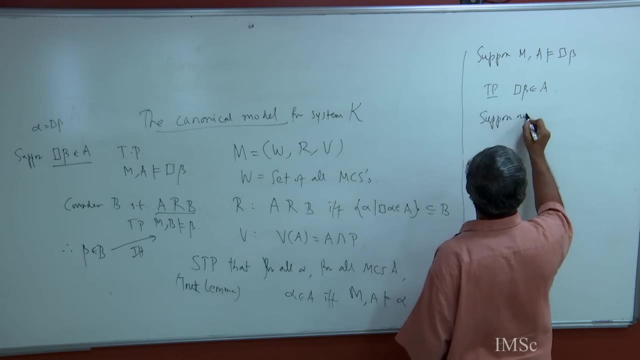 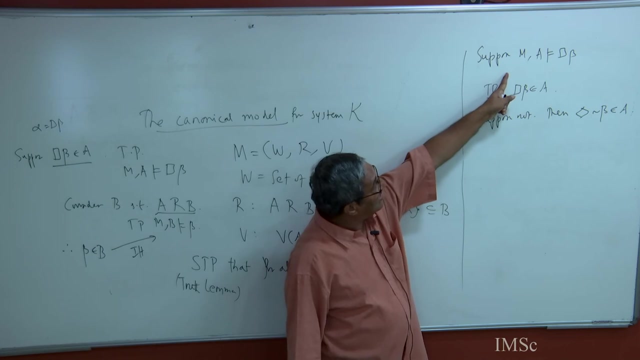 The only way to say is that it is a consistent formula, right? Ok, So this is where. So The only option that we have got really is to say: suppose not, then diamond, not beta, belongs to A. I have to get a contradiction from this. I have to get a contradiction from: 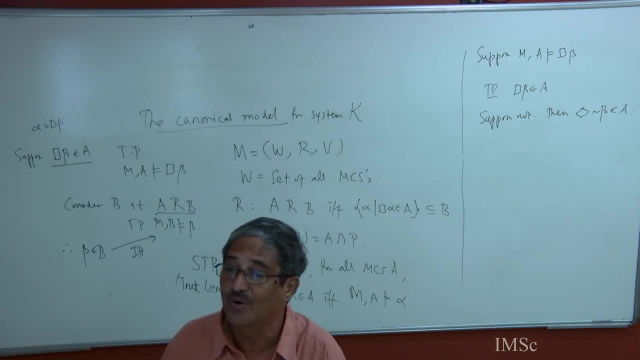 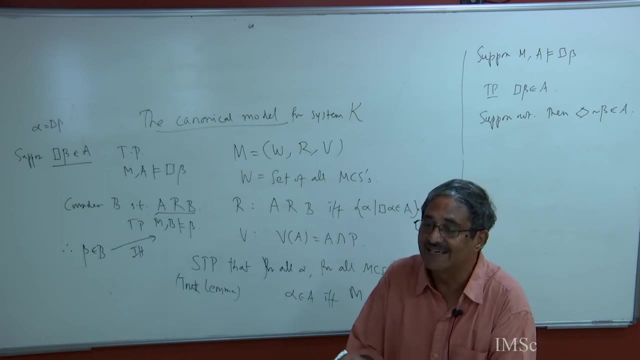 box beta is not true. what I want to say is: box beta is not true in A. Why would box beta not be true in A? When is it that in modal logic formula, box beta is not true in A? When is that Not beta is true in A? 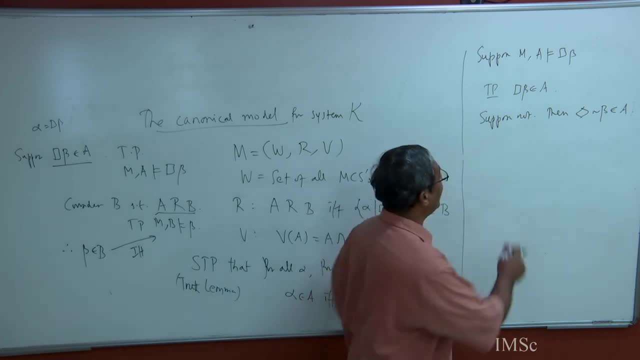 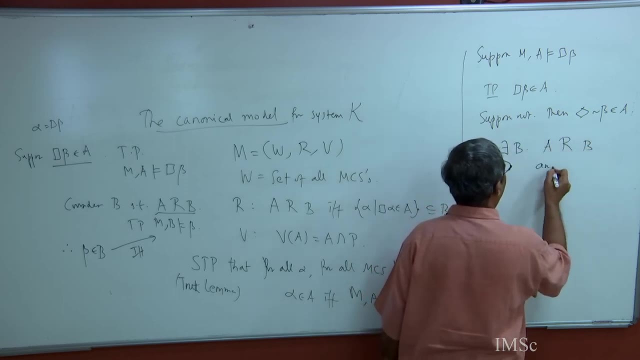 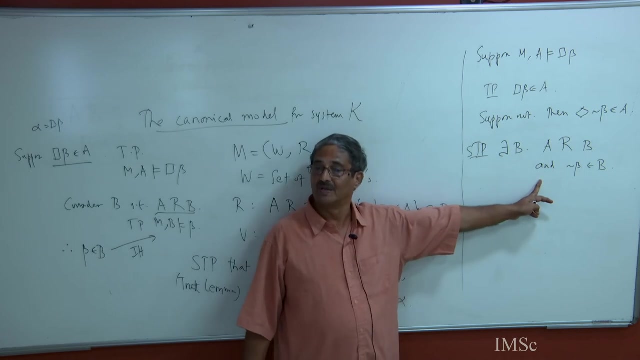 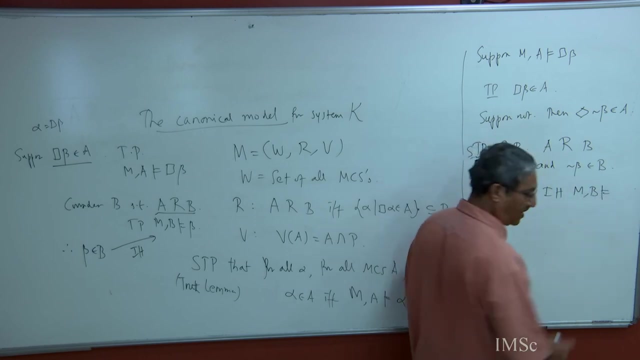 One of the successors, right? So we want to argue that to prove there exists a successor B and not beta belongs to B, Right, I will put sufficient to prove, because if we- this is true, right- suppose there is a successor such that not beta is in B, then what do you know by induction hypothesis? 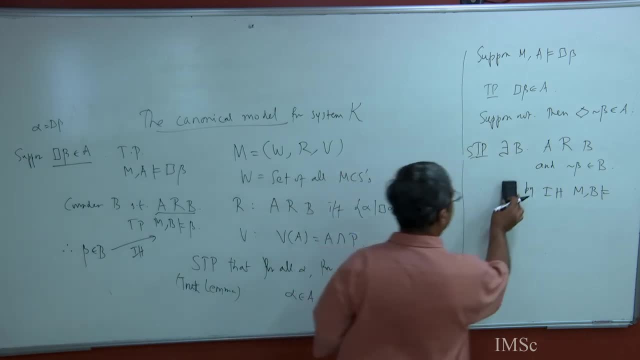 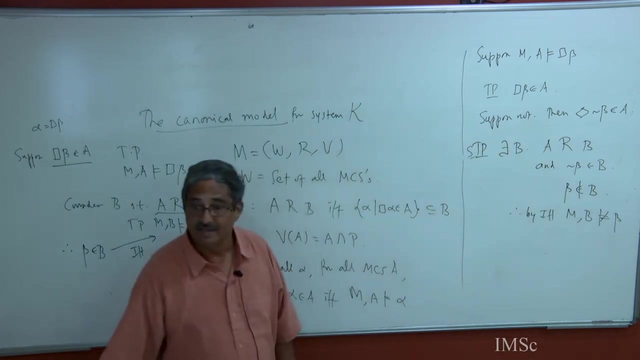 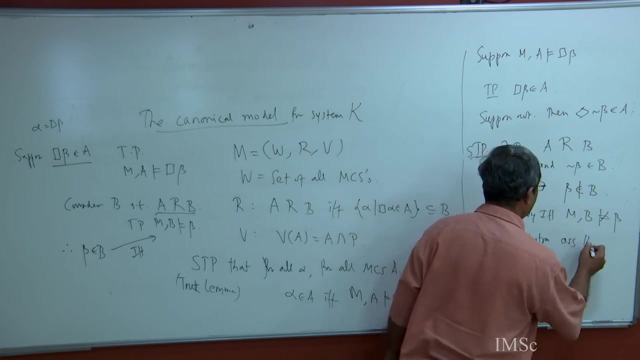 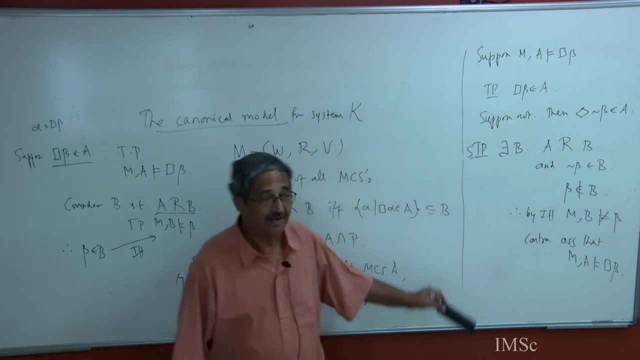 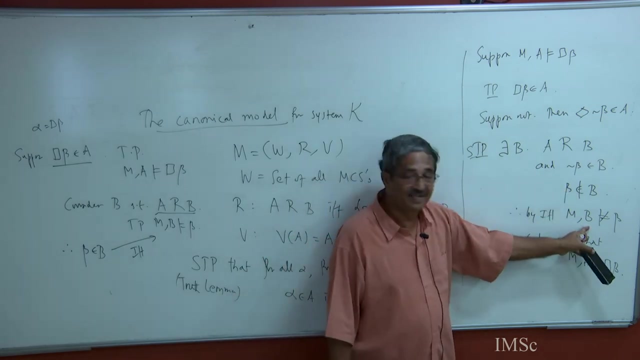 in particular, beta does not belong to B. beta does not belong to B. Therefore, by induction hypothesis B does not satisfy beta. but that contradicts, contradicts assumption that, yeah, we said A satisfies box beta. how is that possible? right, because we have found a successor which? 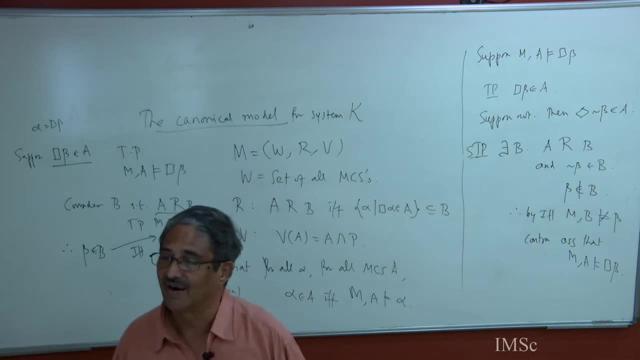 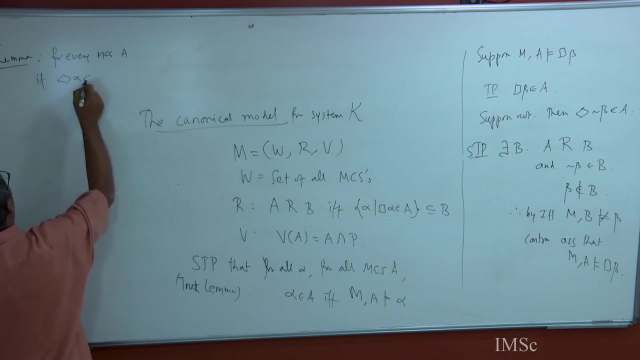 does not satisfy beta Right. So that is a contradiction. So it suffices to prove this, and so this is the generic statement that we want. We want to prove the following lemma For every MCS A: if diamond alpha belongs to A, then there exists a successor B such 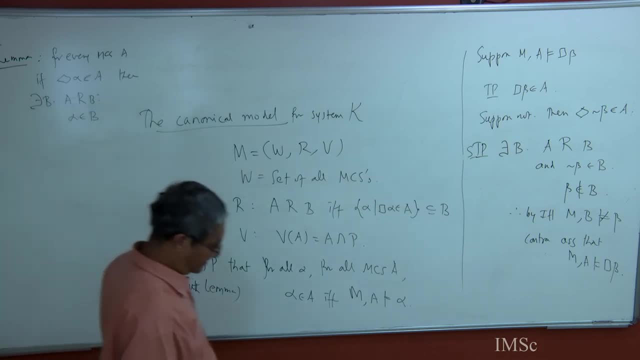 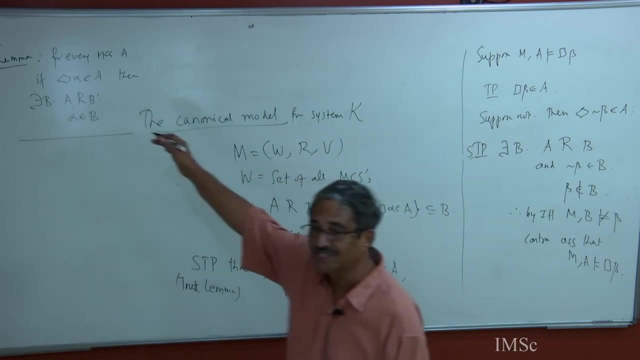 that, yeah, if we prove this lemma, we are through. right, So the entire completeness proof will go through if we prove this lemma, and this makes eminent sense, right? Remember again our decision procedure. the only reason we add edges is: 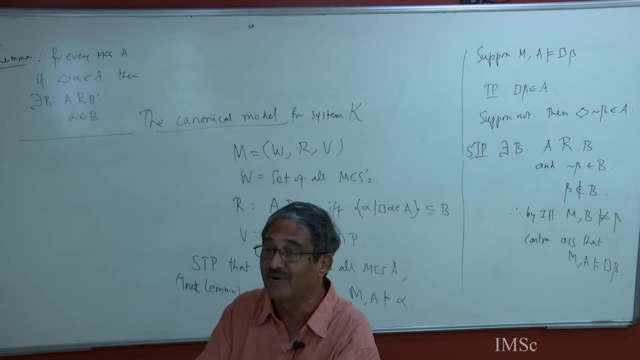 because there are diamond formulas, right, and that is in fact the key argument to say that the branching degree is, you know, bounded Right. Depth is bounded, depth is linear. everything depends on this argument and it is not surprising that when we build an axiom system also, this is the only thing that forces the axioms, and 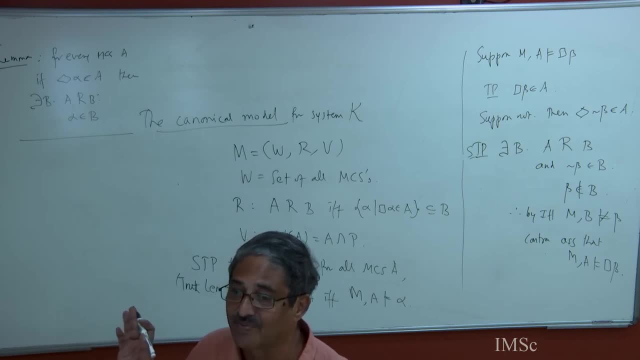 inference rules Right. So far we have nothing. we have only a propositional logic in which we are working Right. So the modal part begins only when you look at diamond formulas, and that makes, as I said, you know, eminent sense. 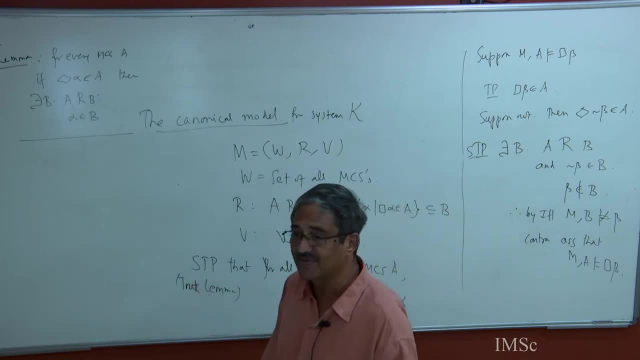 So let us try to prove this and, of course, in the process of proving this, we will have to add some axioms, inference rules. Let us do that, Okay. Diamond alpha belongs to A. We want B such that A is related to B. So we want B such. 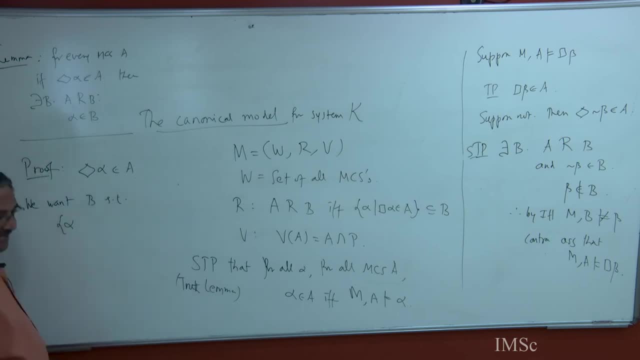 that set of all. we call this beta, Okay, Right, Okay, So set of all alpha, such that box. alpha belongs to A union. beta is contained in B. This is what we want, Right? Why? Because we want this property to hold. this should be a subset of B, and I want beta to. 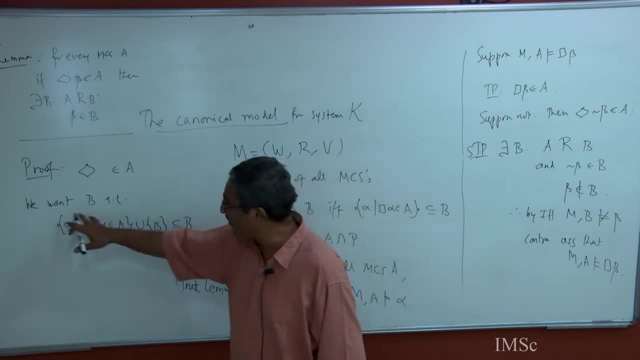 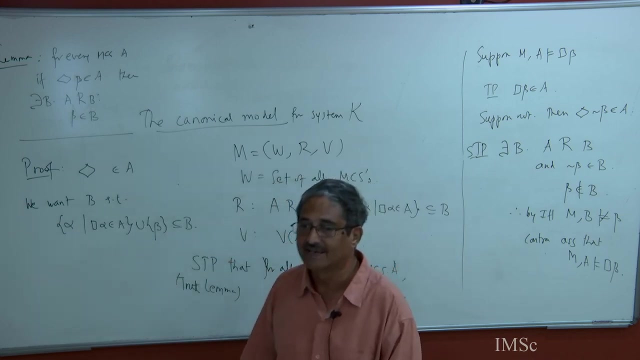 belong to B as well, Right? This is what we want. We want a maximal consistent set such that, whenever box alpha is in A, alpha should be in B and this particular beta should be in B, Right? Is this clear? Yes, Siddharth. 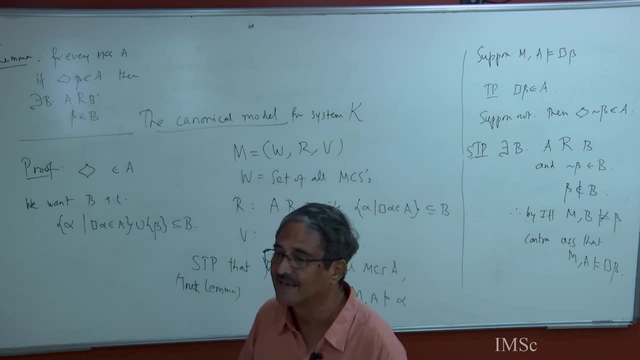 Sir, diamond beta in first line. No, diamond Diamond beta in first line. Yeah, yeah, Of course, Yeah, So we started with diamond beta. This is what we want. If now, how do you show that such a maximal consistent set exists? 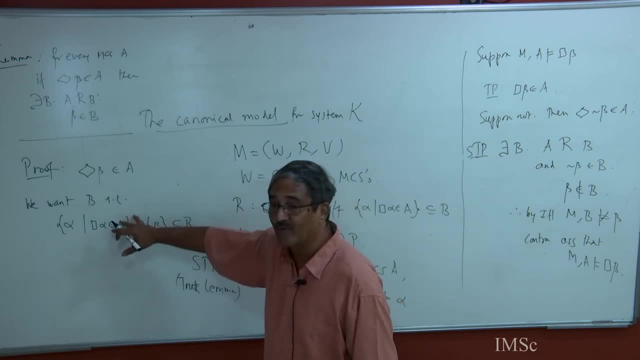 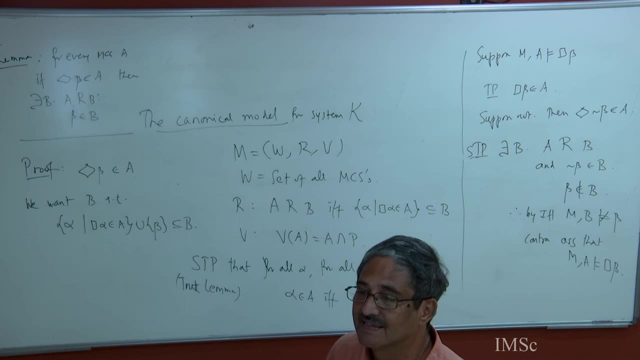 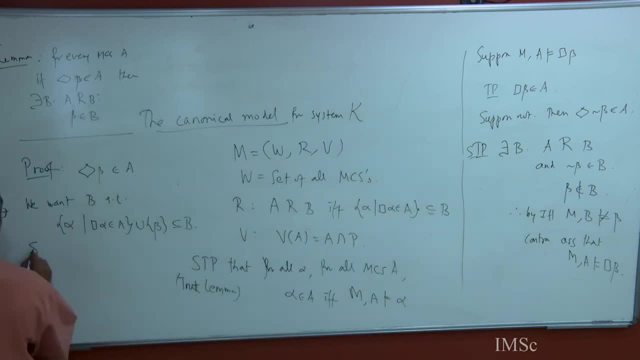 Answer is completely easy: Sufficient to prove that this set is consistent. Why Remember our proposition? If this set is consistent, Then there is a maximal consistent set extending it Right? We know that you give me any consistent set, So therefore there exists a, B and then that is done. 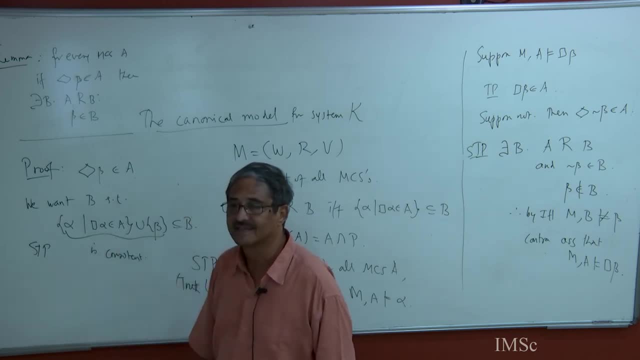 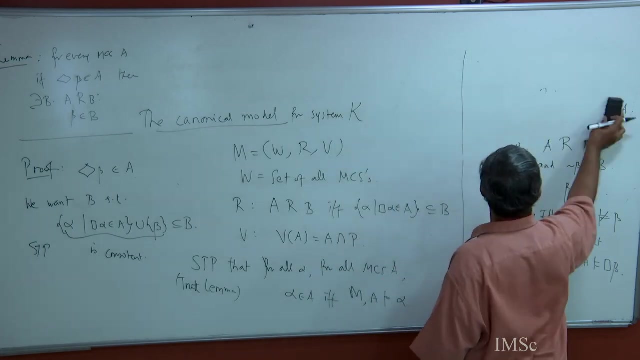 So that entire lemma depends on showing that this set is consistent. Is this clear? So again, we are going down further. all inference axiom system is only in proving that this set is consistent. very good, So let us go further and prove this. 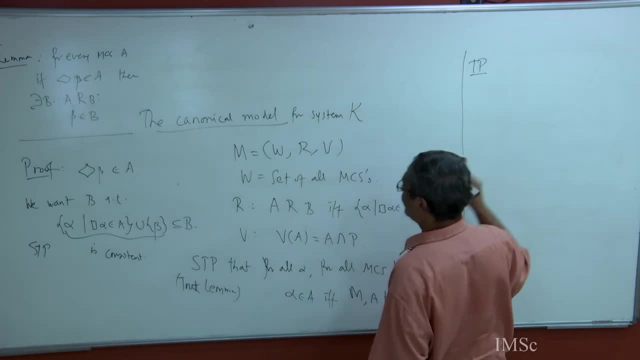 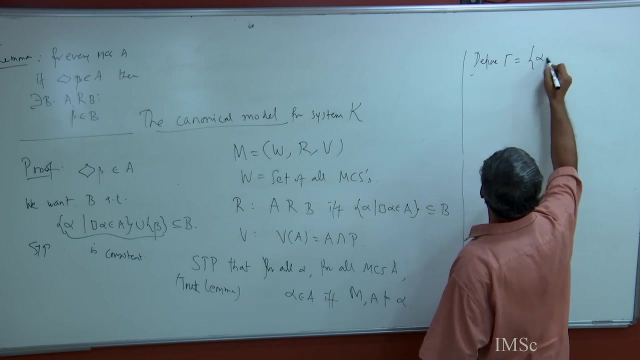 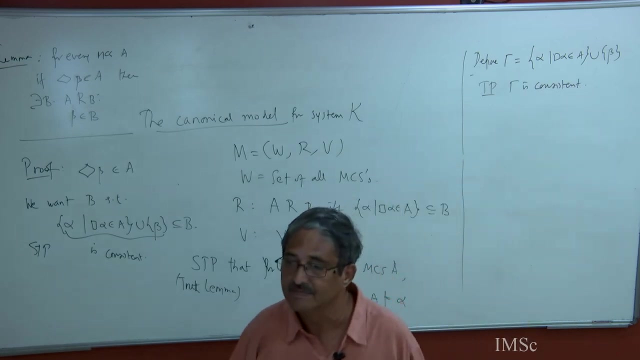 To prove this set is consistent, let us call that set something define. gamma equals the set of all alpha, such that box alpha belongs to A. To prove gamma is consistent. how do I hope to prove that gamma is consistent Again, how do you ever prove that a set is consistent? 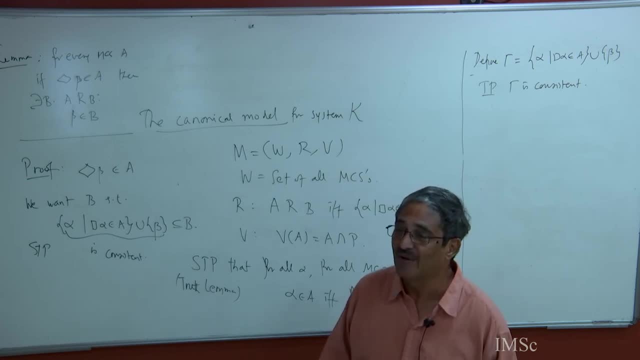 How do you ever prove that a set of formulas is consistent at all? I do not know any way. there is only one way. Say, suppose not, you will get a contradiction. That is a derivation. use the derivation to go into the axiom system and do something. 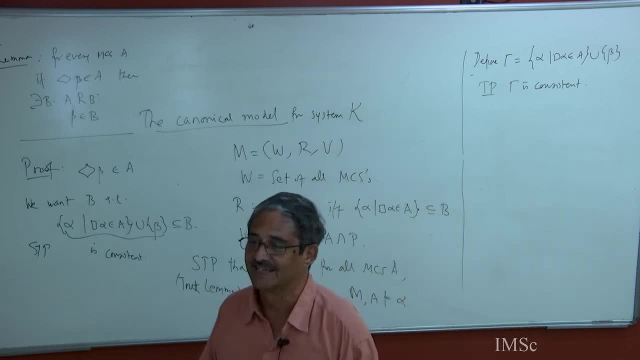 out there. This is our standard way of doing something, Because proving a set is consistent otherwise is hard. What is the meaning of this statement that it is consistent? there does not exist a beta such that beta is derivable as well as alpha is derivable. 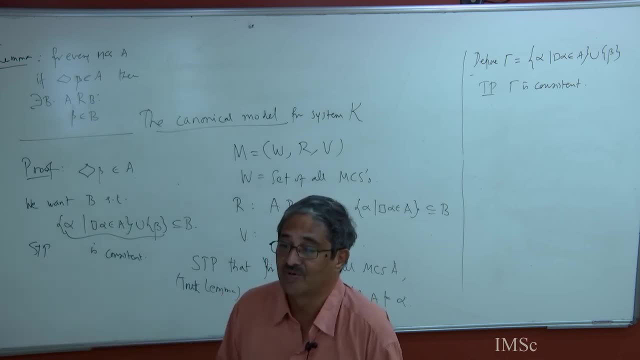 Okay, What is negation? beta is derivable. How do you ever hope to prove something like that? It is much easier to say suppose not and get a contradiction: Suppose not. what does it mean? I have a derivation of beta and I have a derivation of not beta. 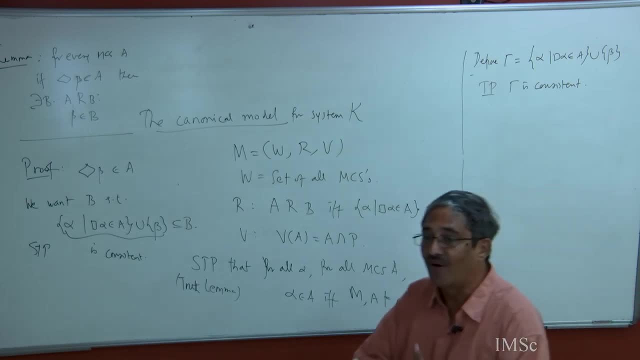 In fact I made you do in the exercises some equivalent forms of these things with consistency. You remember there is some 2-3 definitions. One of the definitions comes in handy immediately, Suppose not. Then there exists A finite subset which is inconsistent. 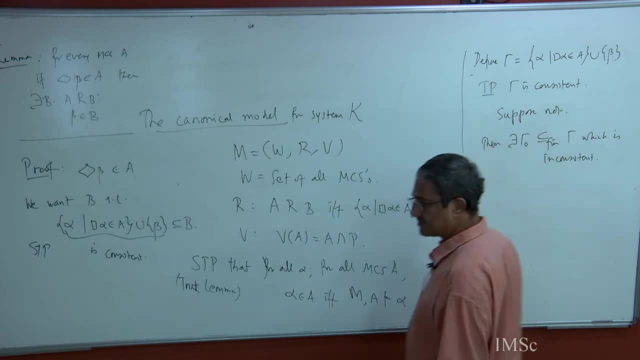 Yeah, You remember, we know this right. I mean, if a set is inconsistent, there is a derivation of beta that will give you a finite subset, gamma 0.. There is a derivation of not beta that will give you finite subset, gamma 1.. 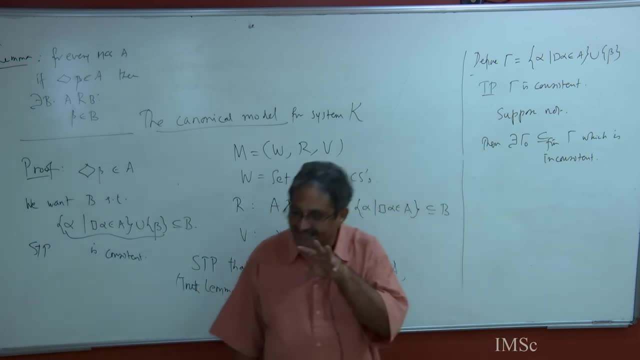 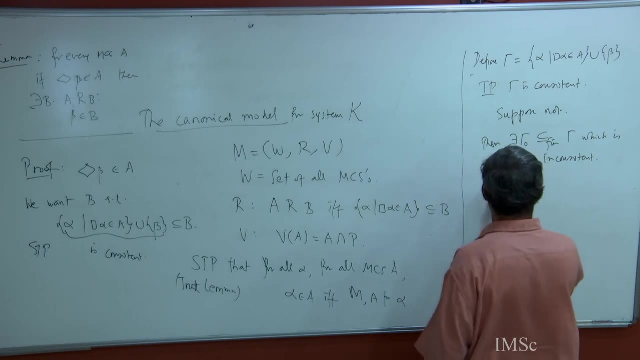 Take the union. So in general, if set is inconsistent, There is always a finite subset that is inconsistent. Is this clear? Now, without loss of generality, I can write gamma 0 to be alpha 1 through alpha k. union, beta, Right. 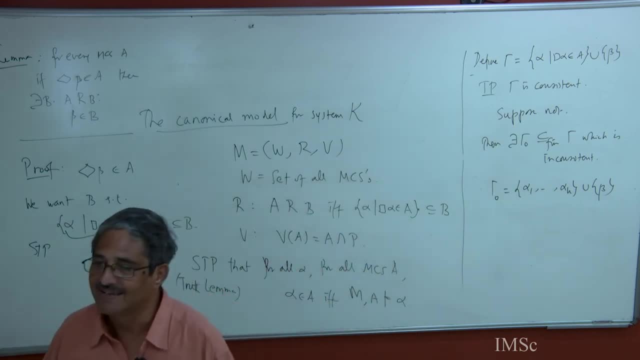 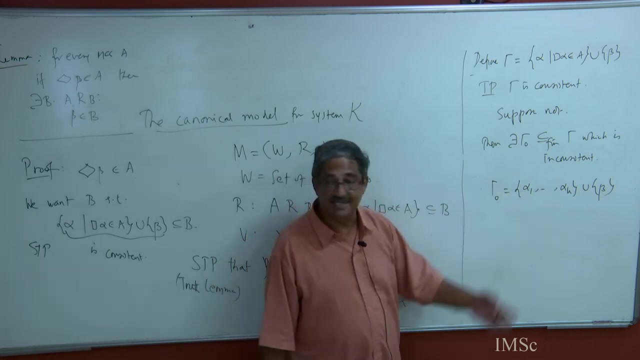 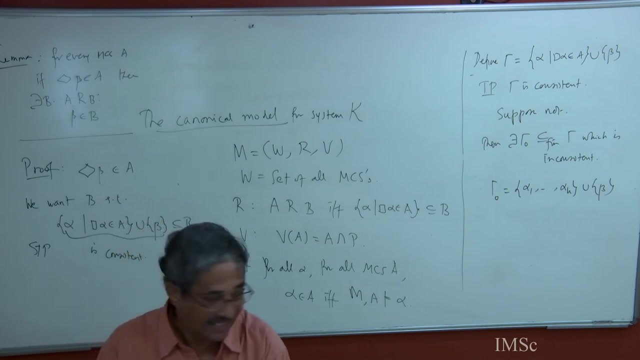 It is a finite subset of that given set, So pick some finite number of elements from both. Yeah, Okay, Now we have to prove that and we are told that this set is inconsistent. Now what does it mean for a finite set of formulas to be inconsistent? 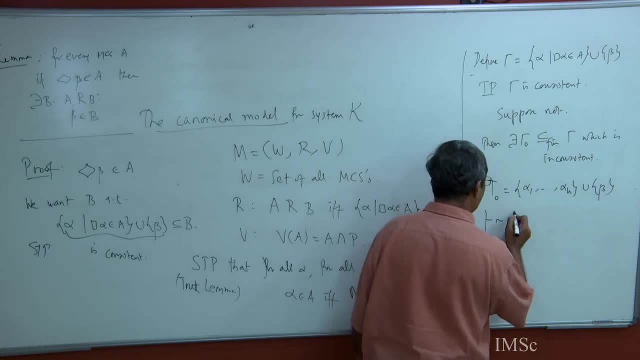 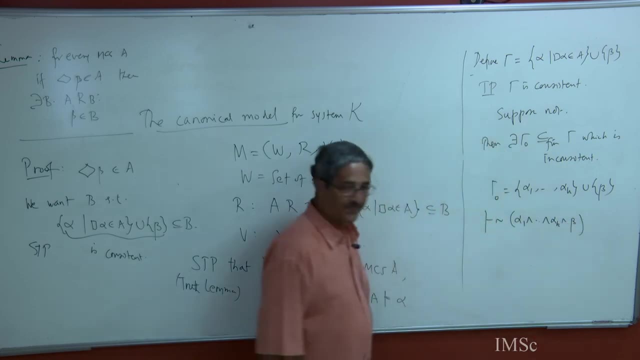 That means that the negation is derivable. Yeah, Again, by propositional logic. In general, Right, A finite set of formulas is inconsistent if their conjunction, the negation of their conjunctions, is derivable. This is one of the exercises that we had long ago. 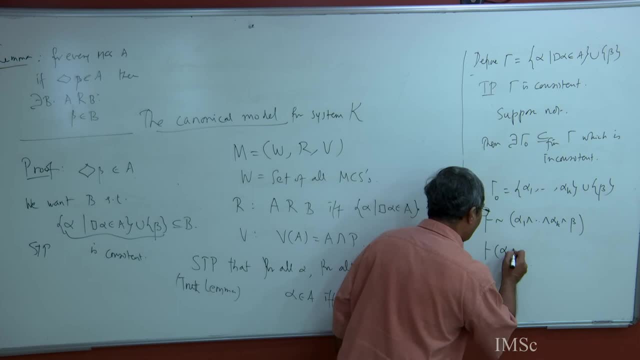 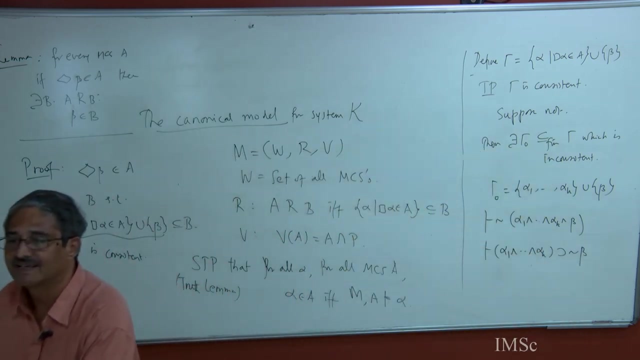 Right Now. this is the same as saying alpha 1 and alpha k implies not beta. I hope this is also clear. This is propositional logic. Yeah, Negation of A and B is the same as A implies not B. Please make sure you understand what. 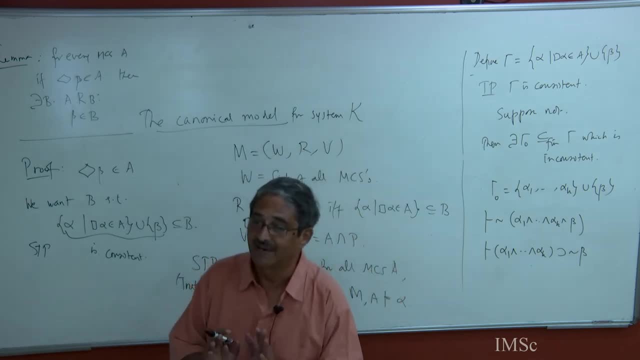 I am saying: All this is just by propositional logic. I am not doing anything modal out here, Right, Okay, Now, at some point now, as I said, I have to use modal logic. Right Now, I see something happening. What is that? 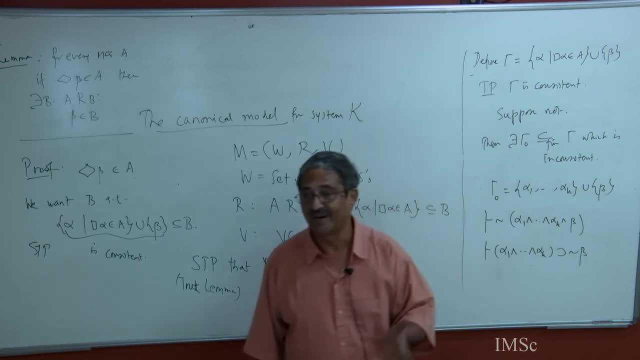 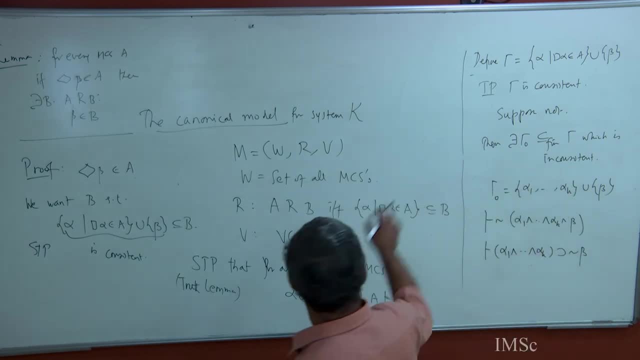 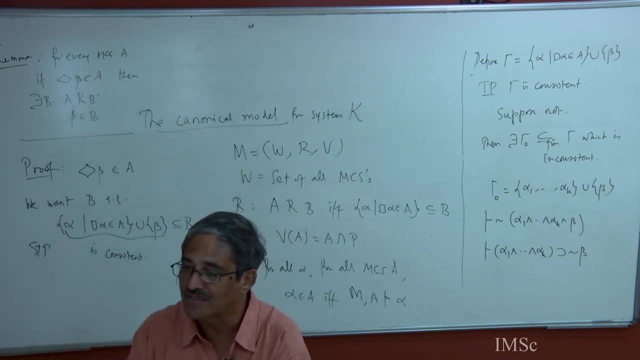 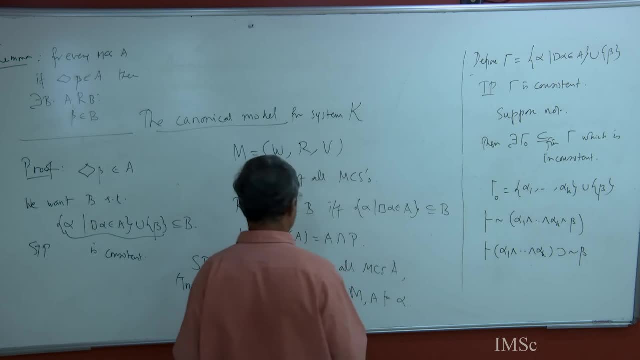 Right. If somehow so, this is the proof strategy. now, What is the proof strategy here? How do I expect to get a contradiction from this? I appeal to the fact that I started with something in A Right. So I know that box alpha 1 belongs to A Box. alpha k belongs to A. 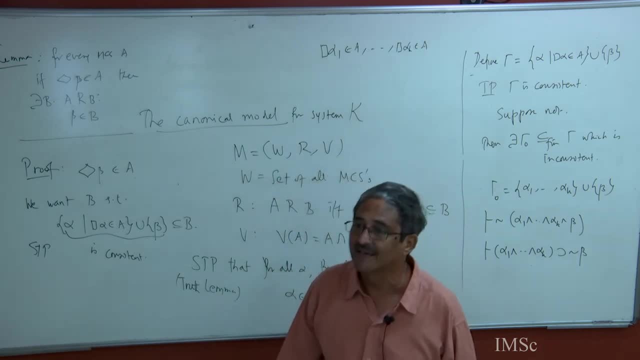 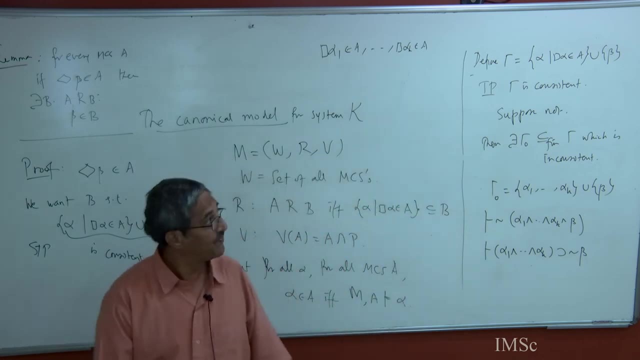 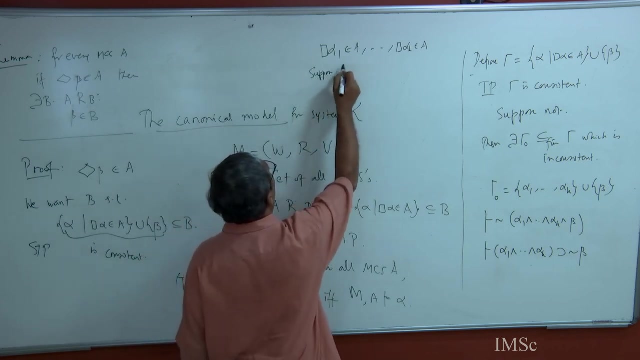 Okay, A right. Actually, I do not even need to distribute right Here, this will do. Okay, I will leave it at that for the moment. yeah, All these belong to A right. Suppose from these, from these I can infer box of alpha 1 and alpha k belongs to A right. 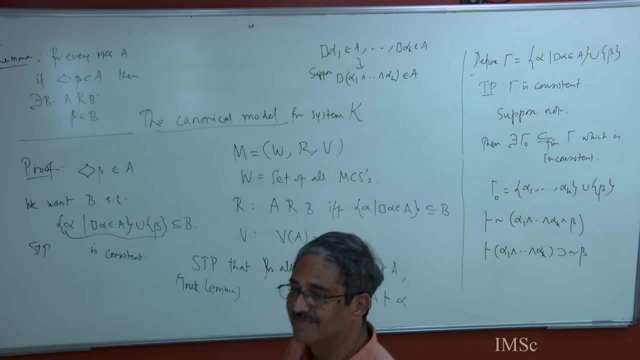 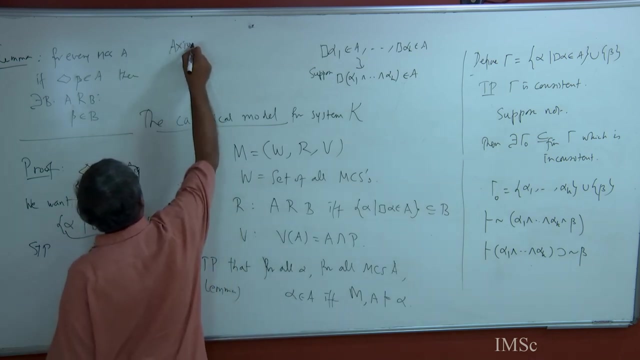 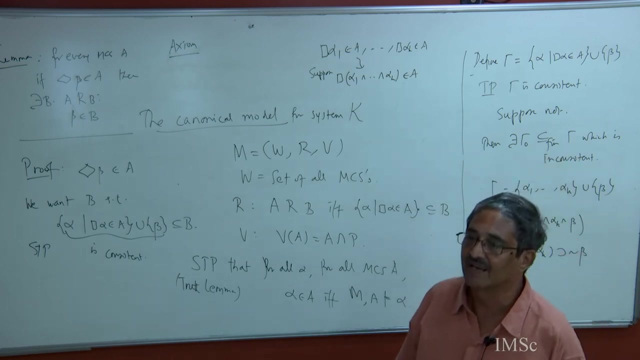 Somehow, if I can use an axiom system to whenever all these belong to A, this formula belong to A as well. And what do I need? how do I make A? do that? What is the axiom that I will need? What axiom will help me to go from here to here? Think of k equal to 2 and tell me. 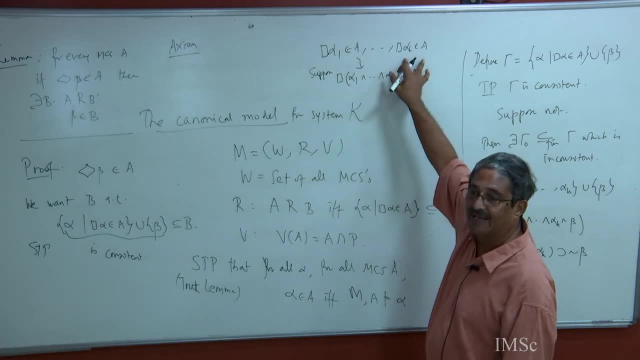 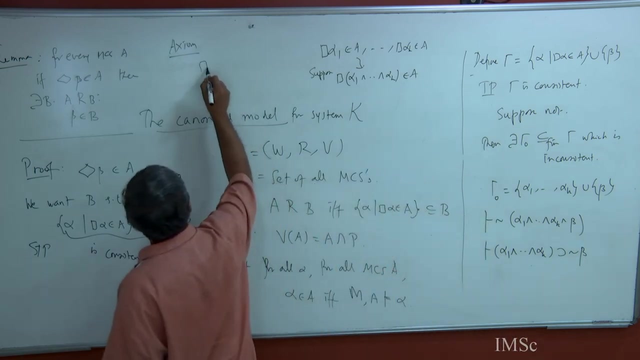 I am told box alpha belongs to A and box beta belongs to A, And I want box of alpha and beta belongs to A. So what is the axiom we want? I need some valid formula, right. What is the valid formula? Simple, If this is an axiom, we know it is valid, You know it is valid, no, In fact it. 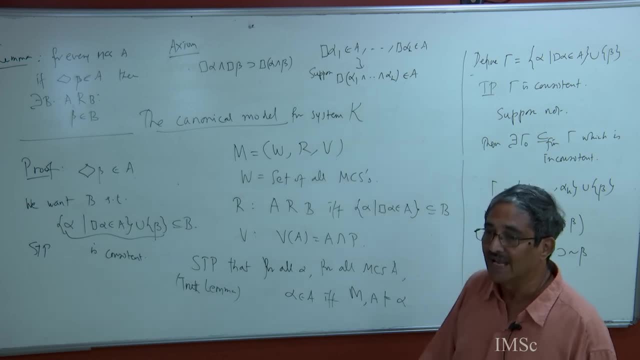 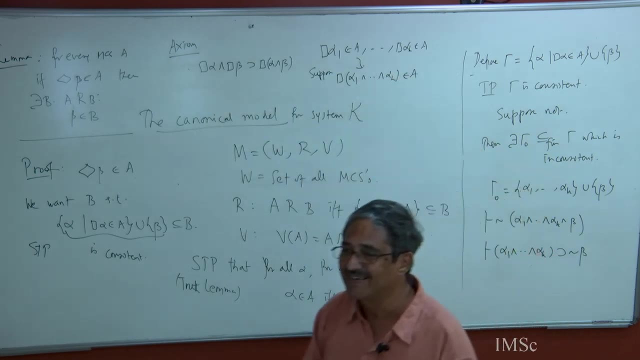 is an if and only if. In particular, if I have this as an axiom, then of course I can the k do not worry about it, right, Because I can always call this alpha 1 and this is alpha 2 through alpha. 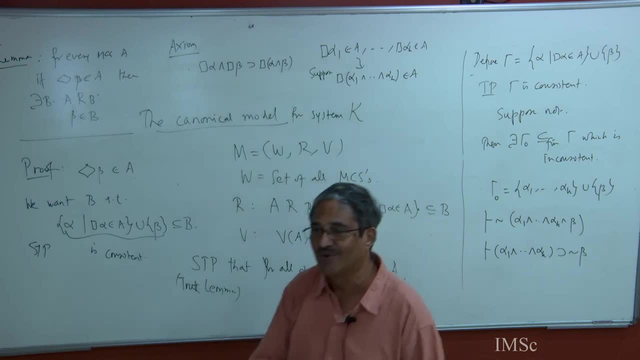 k right. Apply the rule many, many times and you will get it. That is all usual, right? So with this as an axiom, I can go from here to here, ok, So this much is clear, right? So if I go from here to here, I know that diamond beta belongs to A. That also was given. 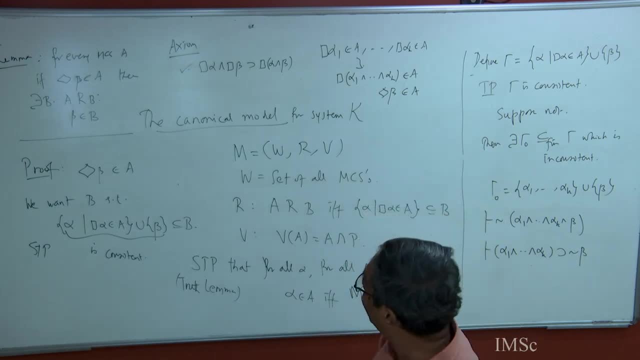 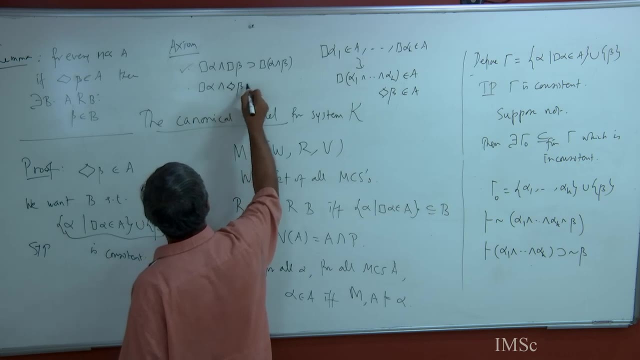 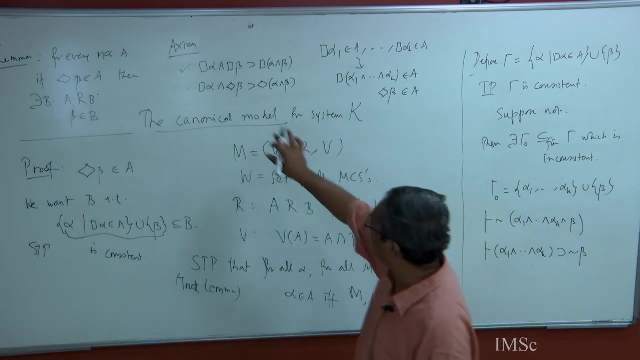 to me. I have to use it somewhere right Now. notice that something. the axiom suggests itself. Yeah, Box alpha and diamond beta surely implies diamond alpha and beta right. If every satisfies alpha, one of one must satisfy alpha and beta, right. Is this clear? So this is. 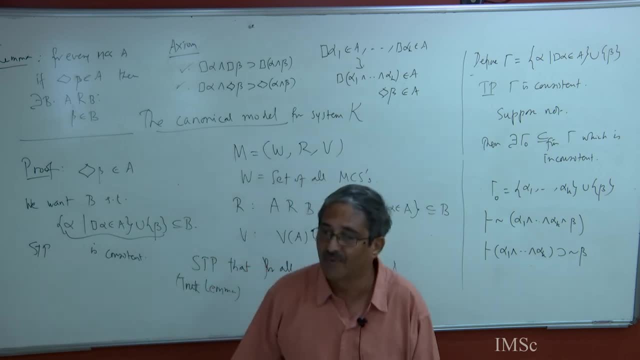 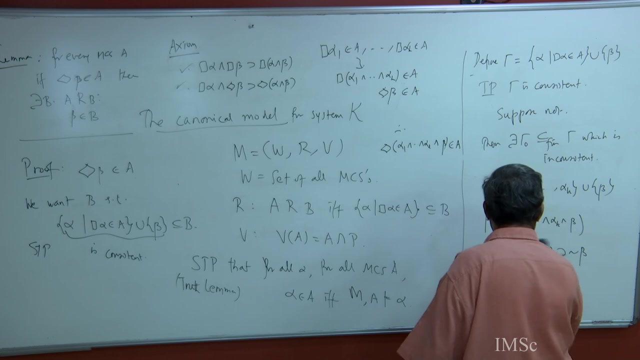 also a useful axiom. It is a valid formula. throw it in as an axiom. Now. what do I know? Therefore, diamond of alpha 1 and alpha k and beta belongs to A. We have come. I do not need this. we have come so far, right, So I do not even want. 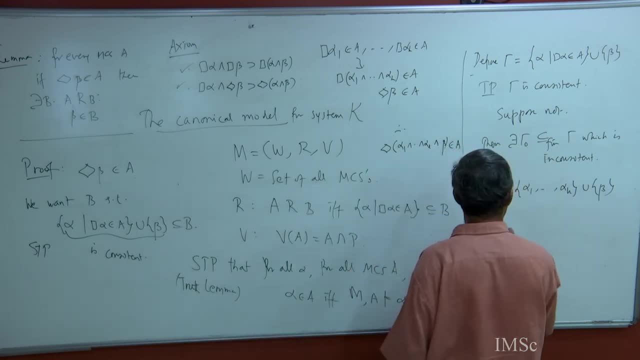 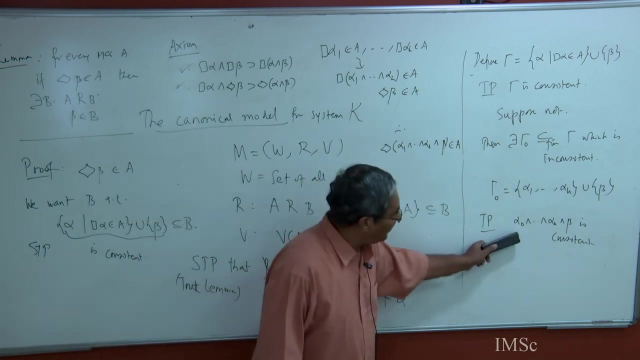 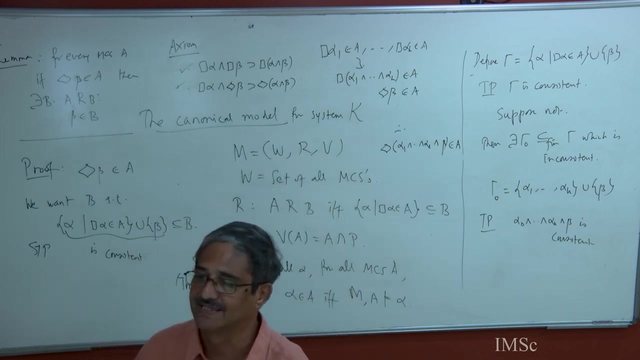 to get into this negation business. So, to prove that this formula is consistent, yeah, I want to prove that, this particular formula right? What does it mean for a finite set to be consistent? The conjunction of the formulas is consistent. So this is what I need to prove. How do I? 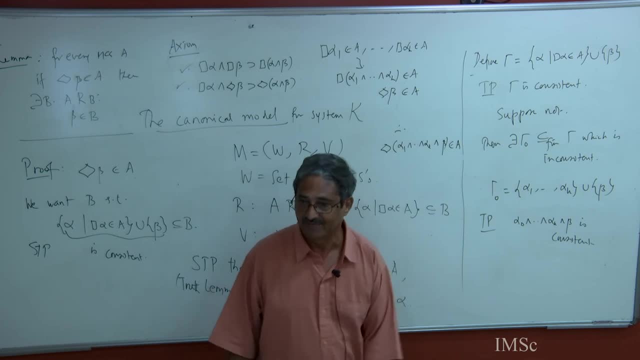 prove that this formula is consistent. Well, we will see. I have brought it down exactly to that. Now, something interesting is happening. We know that, therefore. so therefore, diamond alpha 1 through alpha k and beta is a consistent formula. 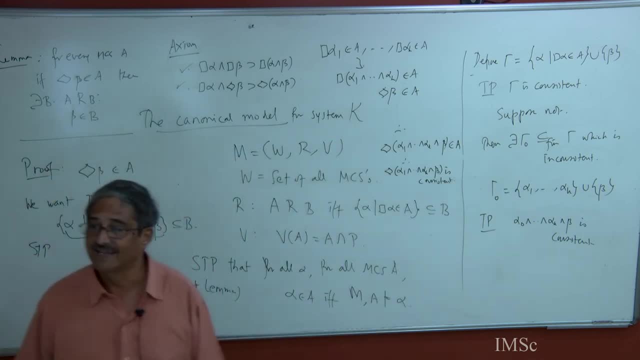 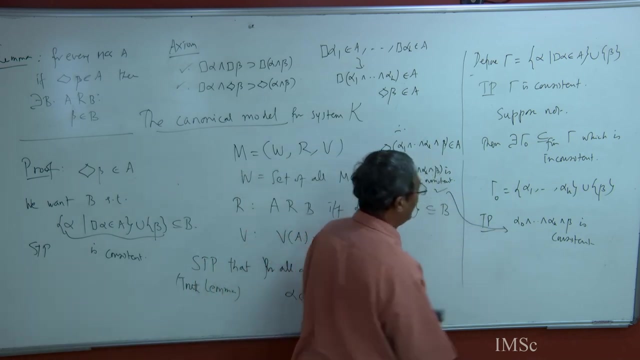 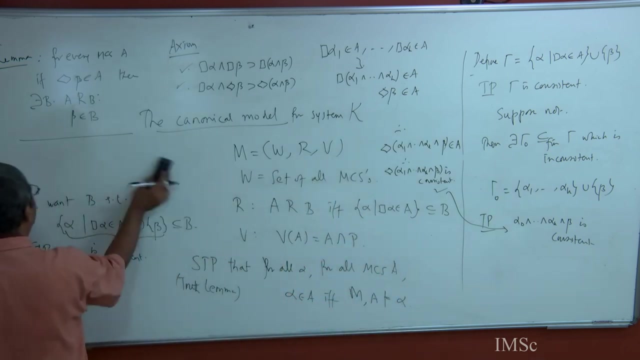 Okay, That is clear, right, It is a formula sitting in A. A is a consistent set, So every subset of a consistent set is consistent. So this is a single term set. So we know this so far. So from here I want to somehow go here. What is the form in which I want this now? 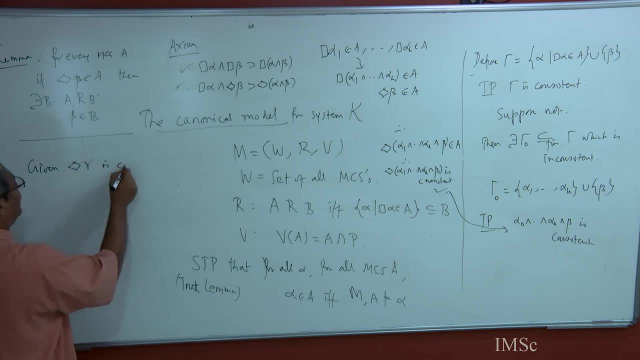 Given, Given, Given. So this is zacks as p by omega snap. So 1. 控enuptial degree inverse x, k, comma ztax: You are getting a devotional steady price. So it should be, it should be…. 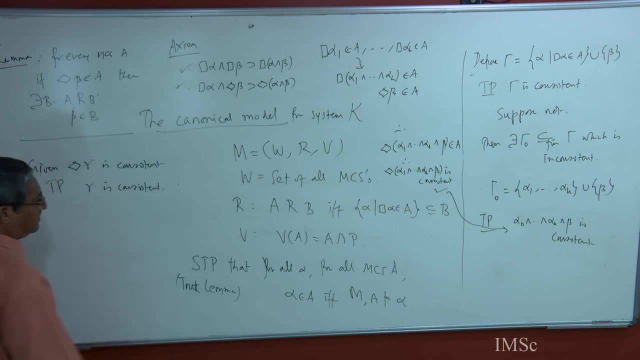 gamma is consistent. Now, what I mean by gamma is consistent? Great, I take a. 2. To prove gamma is consistent. How do I ever hope to have this? So this is the 1 time you are seeing an inference rule of this kind. Suppose I have an inference rule. oh, if you want, I will write it as contrapositive. 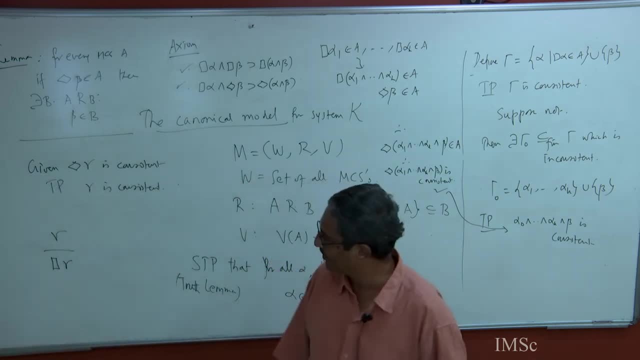 If 2 takes the estou, then gamma is equal to 2 0 0,. if 2 takes the superimposed quantity of gamma, it means 0.ke Great. If diamond gamma is consistent, then the contrapositive is: if gamma is inconsistent, then diamond. 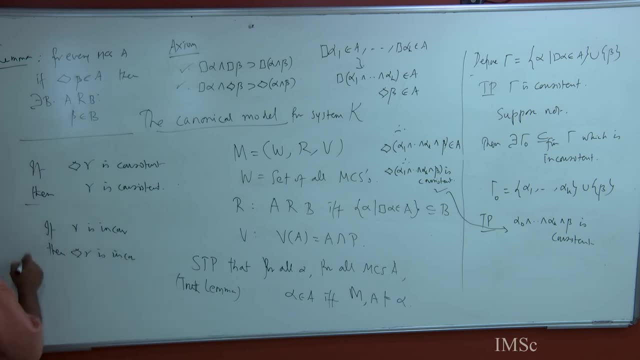 gamma is inconsistent, right? What is gamma is inconsistent mean? If negation of gamma is a theorem, then what is diamond gamma is inconsistent means? what Negation of diamond gamma? that is the same as box, not gamma. So if not, gamma is derivable, I want to show that box, not gamma, is derivable. 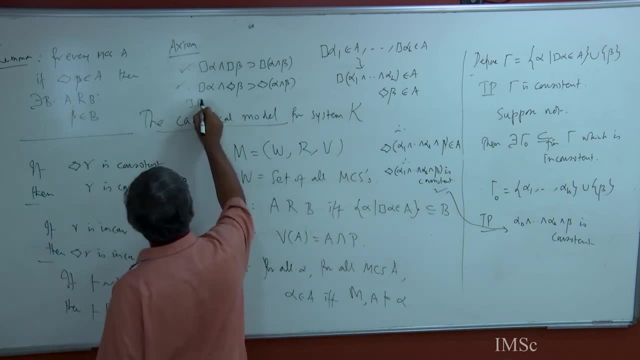 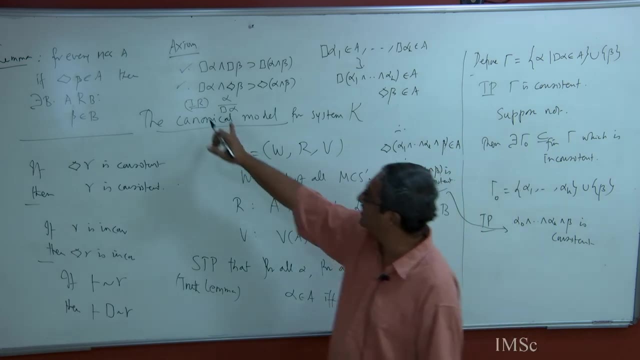 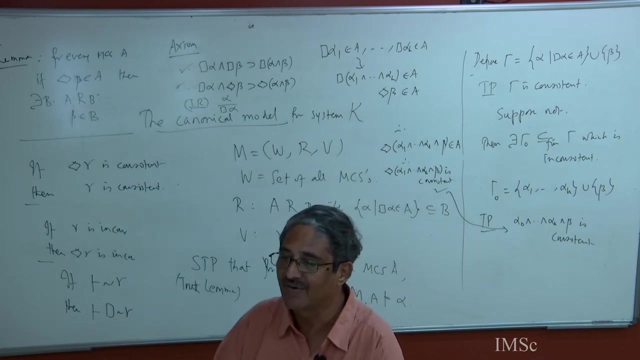 So the simplest thing is to add an inference rule, and we know it preserves validity. If not, it does not. If alpha is, remember first order logic, we said generalizations are always allowed. right. Whenever you have got some alpha, you can always throw in for all x alpha. 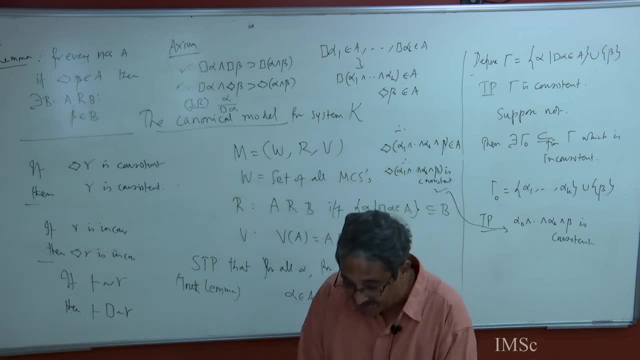 The equivalent here is in model logic box. If alpha is true everywhere, it is true in every model, every world. So of course, box alpha is true everywhere. How do you prove this? Suppose this is valid, it is not. What does it mean? 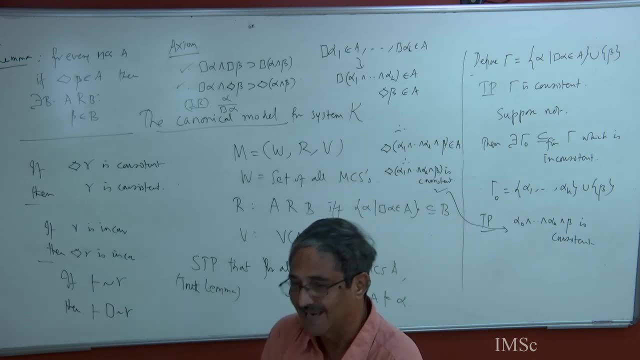 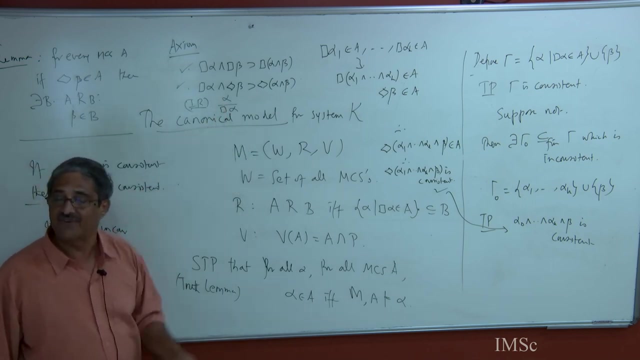 There is a particular world where box alpha does not hold. That means there is a successor where alpha does not hold, But that will violate validity of alpha right, and that is it. So therefore, if, whenever you have got a rule like this right, if alpha is derivable, then 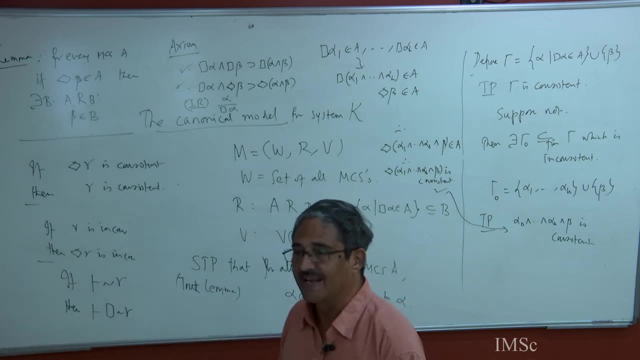 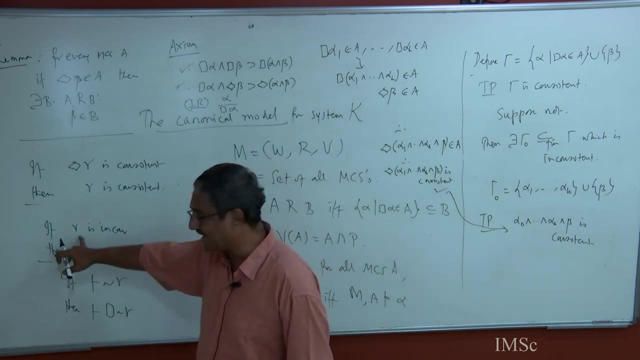 box alpha is derivable. That is the same as by substitution we get. if not gamma is derivable, then box, not gamma- is derivable. That is the same as saying if gamma is inconsistent, then diamond gamma is inconsistent. Therefore it goes the other way. 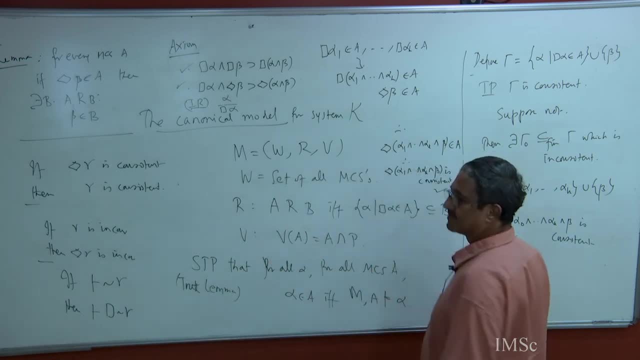 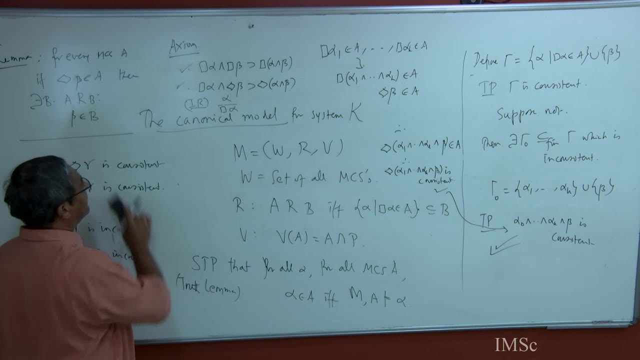 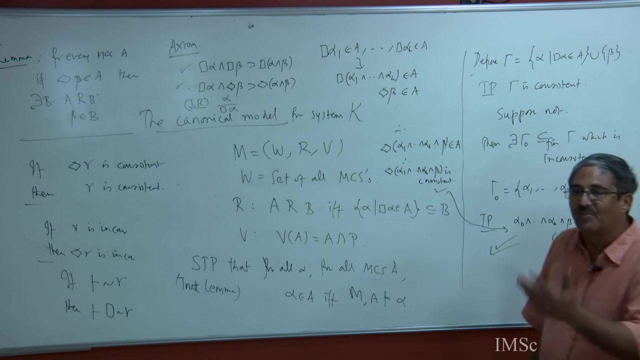 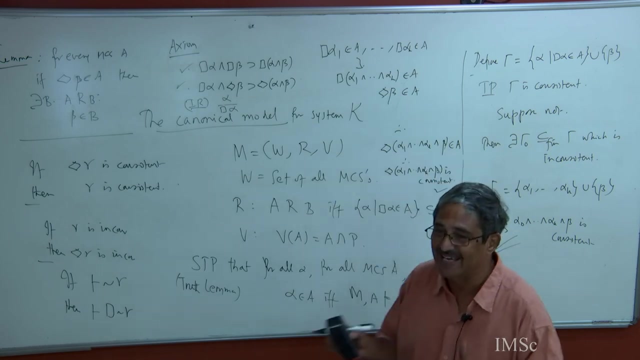 So, and we are done right. So, finally, and that is it, So I am going to leave the steps here for a moment. So this completes the completeness proof: two axioms and one inference rule. What are? and the axioms are natural, right, right. 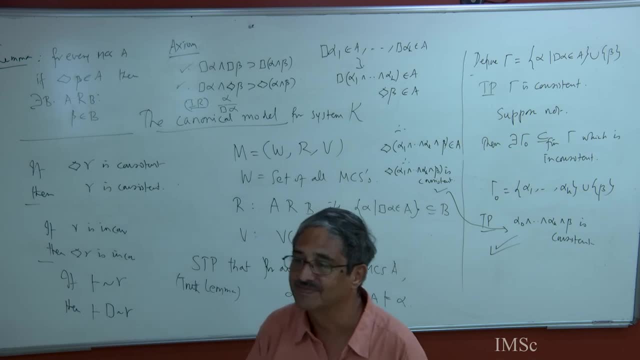 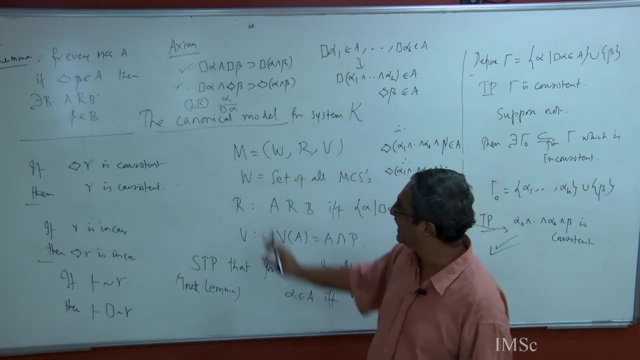 This is really the meaning of What your modal formulas right? If something is true everywhere, it means that you can combine the box. The second one says that once you have got a box and a diamond, it results in a diamond. And this is that wherever you, yeah. So I hope this proof is clear. So now, 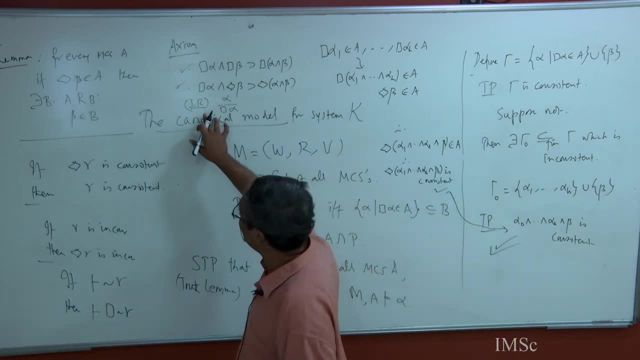 you are learning one important thing, which is the how the rules relate to consistency. right, When you have an inference rule, it says: if something is derivable, something else is derivable. So, consistency wise, what it is saying is you have to go the other way. 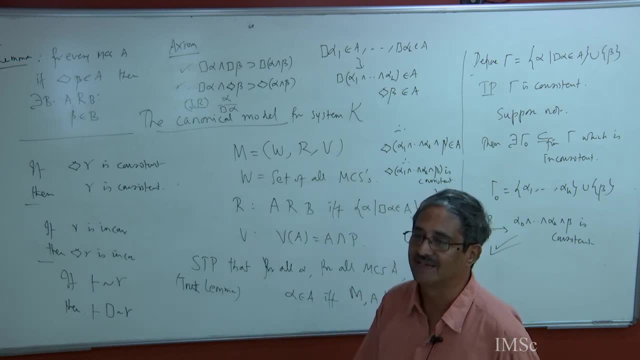 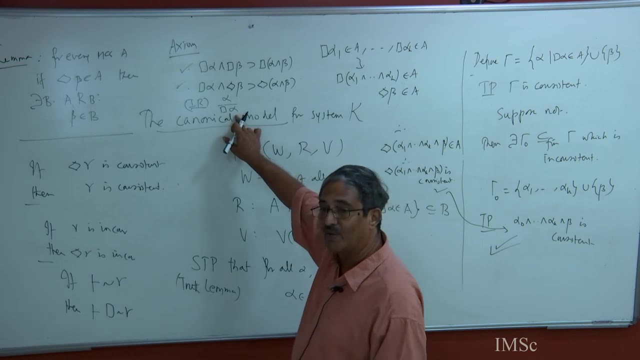 If the conclusion is consistent, then the premise must be consistent, right. But in a dual the dual of the conclusion is consistent. So here it is box alpha the dual. If diamond alpha is consistent, then alpha is consistent. I mean this is true in first order logic, as 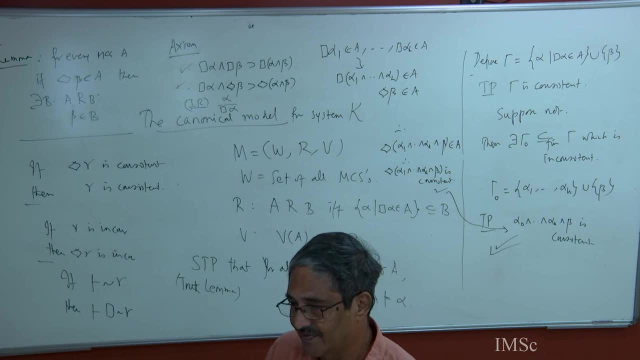 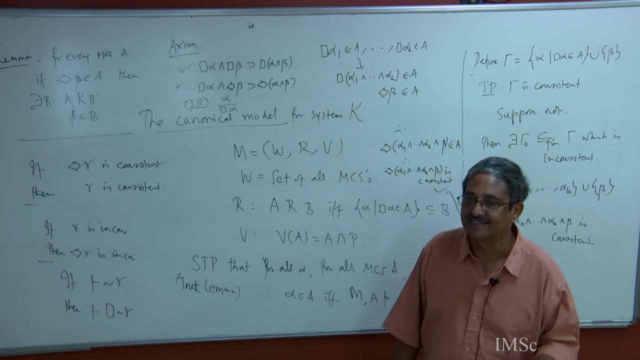 well, If there exists x alpha is consistent, Then alpha with x replaced by some particular term, t right is consistent. This is real And that is how you build the Geidel completeness proof right. There exists x, alpha is given. 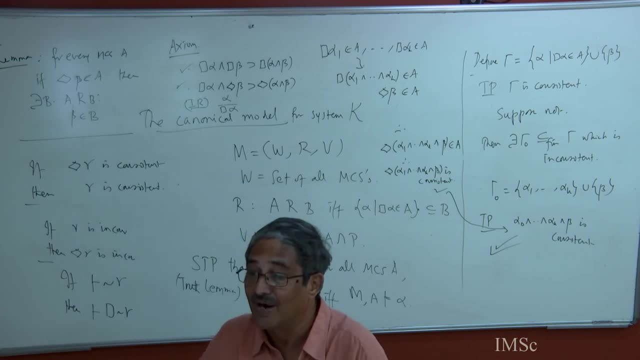 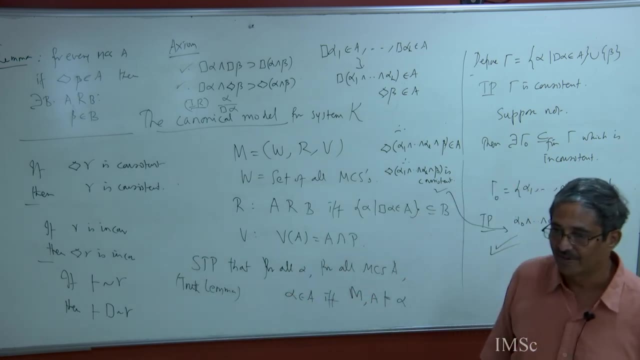 to you. You guess some term t right, Remember a new variable or something that you do and you put it in right And you preserve consistency. That is exactly the same argument, ok, So it is one uniform kind of idea that we are following through in all this. ok. 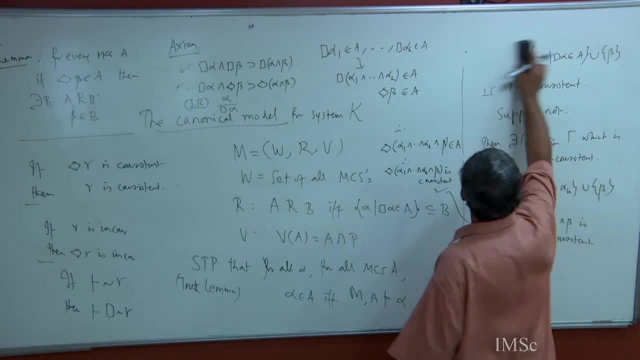 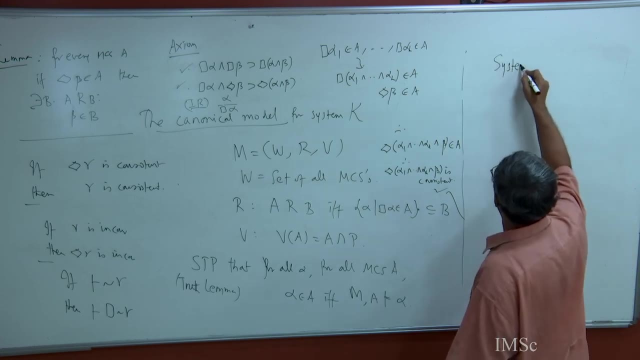 Thank you, Thank you, Thank you. So this is the Kripke axiom system for modal logic, So system k as it is called, But instead of these two axioms. so of course you have first axiom is always all substitutional instances. 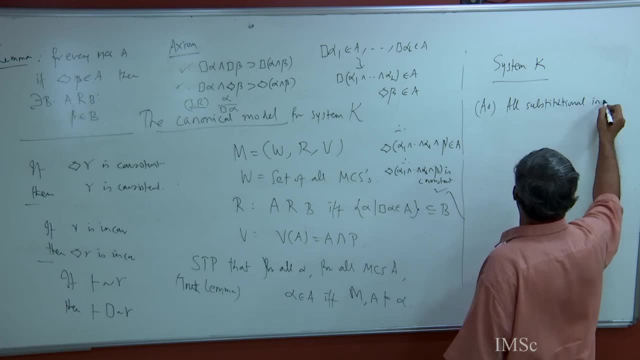 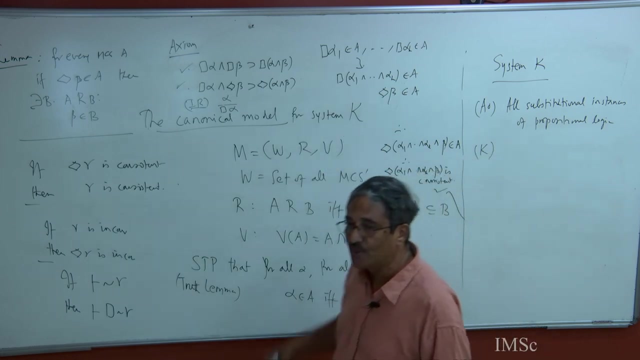 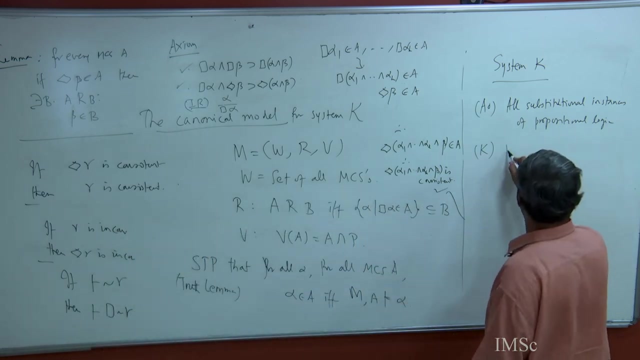 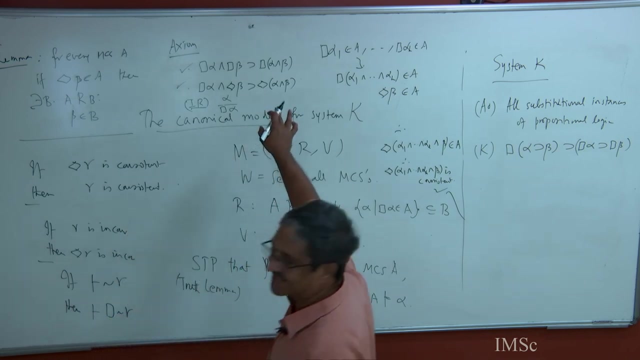 of propositional logic. Ok, Ok, Ok. And then the K axiom. instead of these two acorns, Kripke proposed a single axiom from which all these things are derivable, And this is the axiom, rather than conjunctions. right, This is the general. I mean, this is old Hilbert thing. 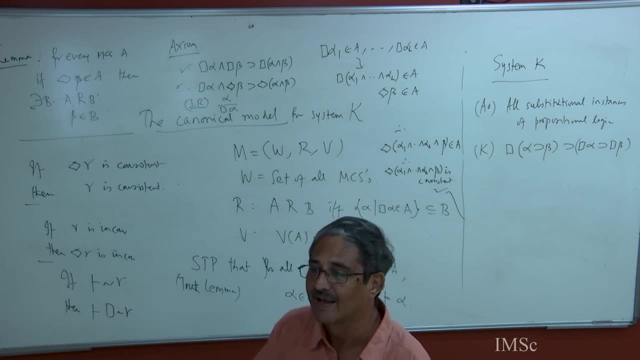 and, as a matter of convention, people try to follow that. And also it is really beautiful because it always brings it down to essential thing. So this is called axiom K, and notice that it is valid. I hope it is clear that it is valid, right? How do you prove that? 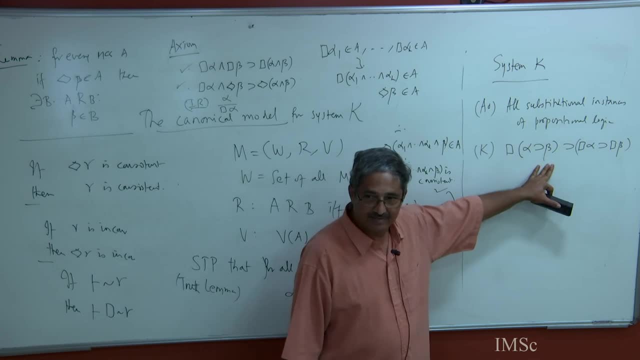 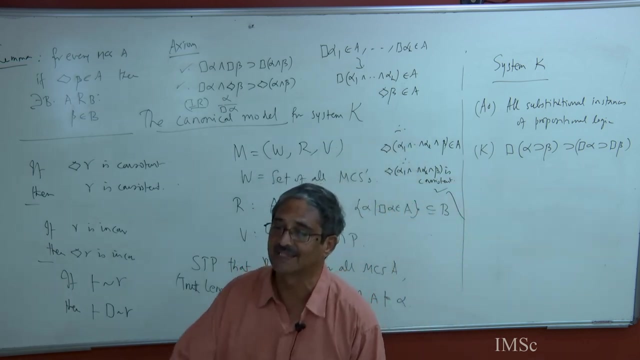 it is valid. Suppose not assume this is true at some world but it is false at some world. False at some world means box alpha is true in that world, but box beta is not true. Well, that is a problem. Box beta is not true meaning there is a successor where beta is false. 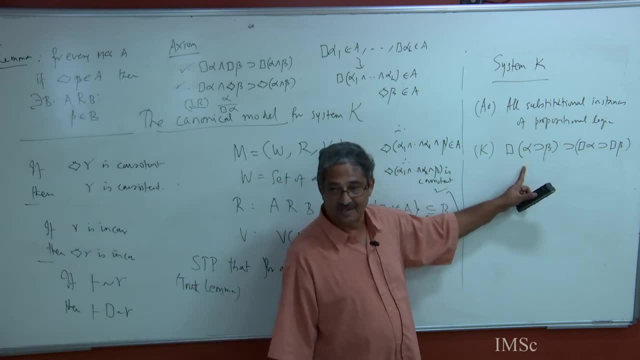 right. Well, alpha implies beta was true at that world w and alpha was true at that world right Box, alpha was true. that is Therefore in that successor world that we are looking at. alpha implies beta must hold as well as alpha must hold. Then how did beta become? 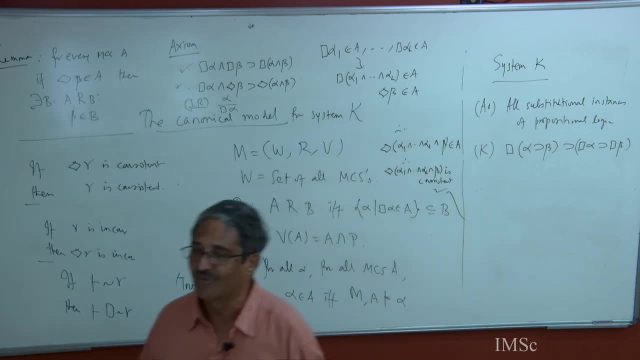 false Beta also. So it is. you know, this is exactly what right The modality preserves. consequence is the idea. This is what logicians will say: right, If necessarily alpha implies beta. once you have necessarily shown that alpha holds, you have shown that necessarily beta. 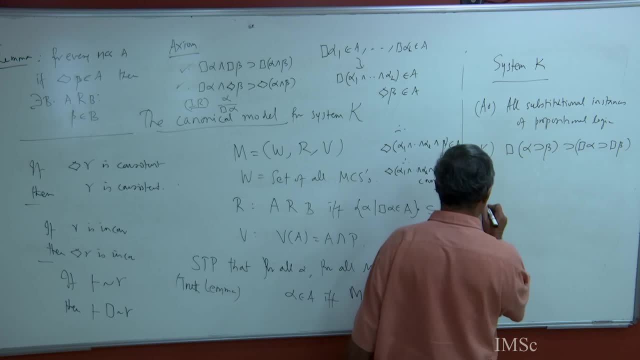 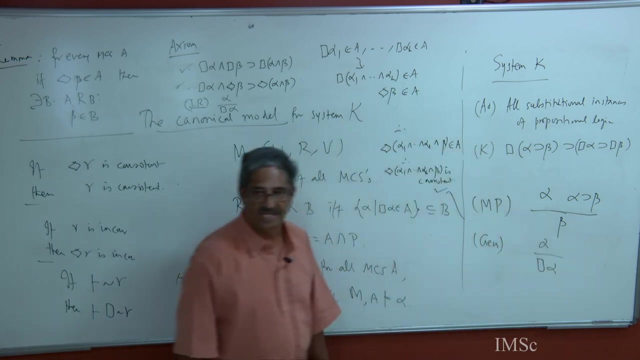 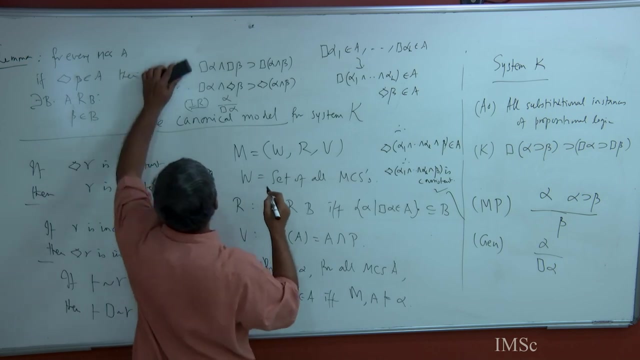 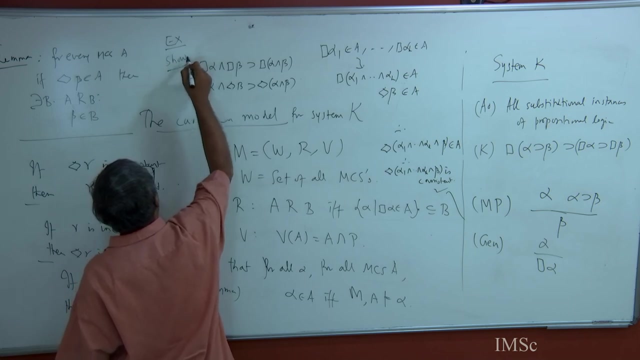 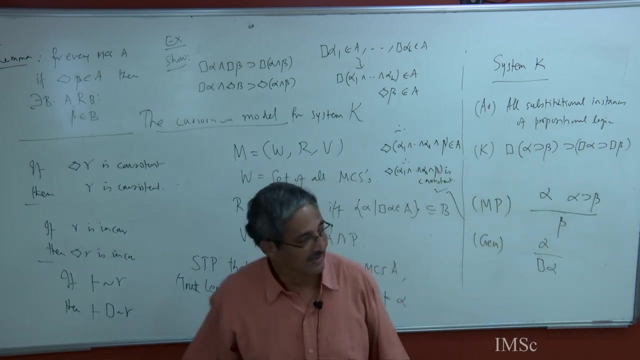 holds as well, And then the inference rules, modus ponens And generalization. That is it. Now. it is an exercise to show that, show that these are derivable. Yeah, This is enough From this. you can derive it, Okay, Thank you. 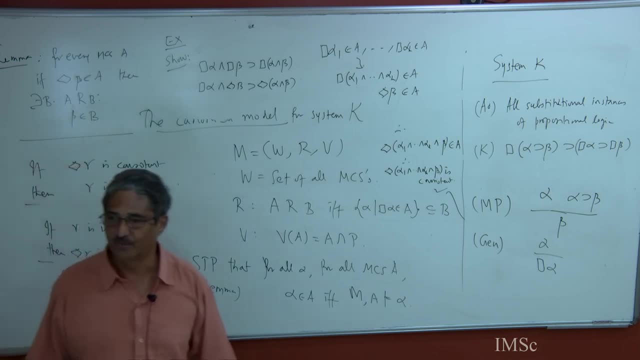 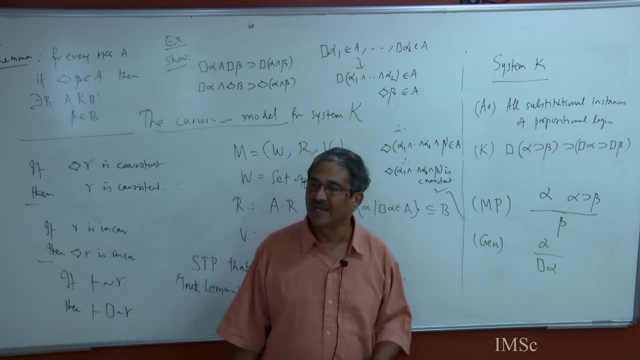 Thank you for your attention. Thank you for your attention. So that is a nice exercise to take upon, right? So that is. Is the flow of the proof clear, Like I have told you earlier, also completeness proofs: it is always good to discover what is going on by a construction, But after that you 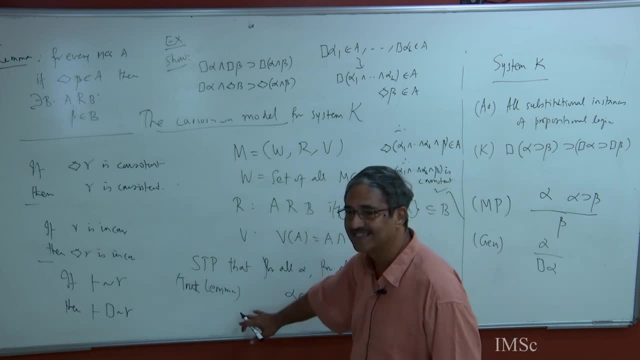 have to do a bottom up proof right. Here are the definitions. here is this right. We have to prove that every consistent set can be extended to a maximal consistent set. Define the model, do the truth lemma. what are the steps? base case, propositional case. 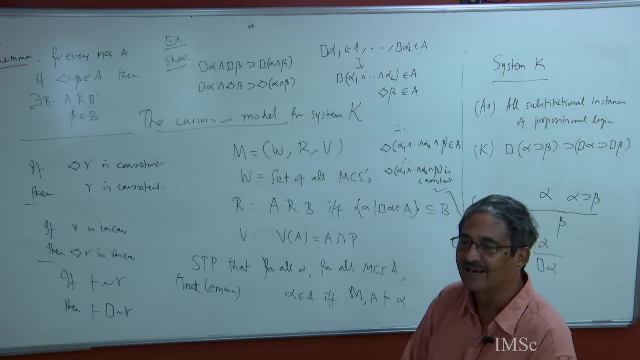 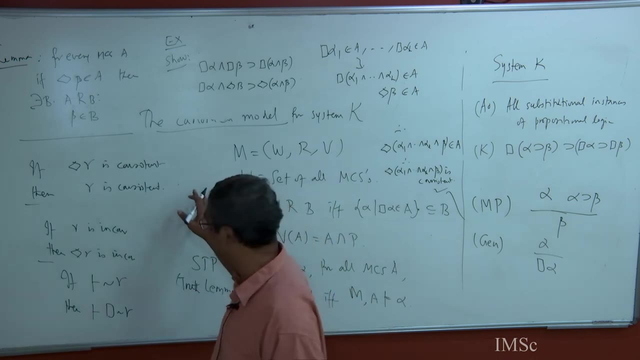 follows: by definition, Boolean cases are routine. and then you come to the modal cases. For box alpha, it is by definition of the relation that takes care of it. For diamond alpha, you show that it suffices to prove this lemma. How do you prove this lemma? 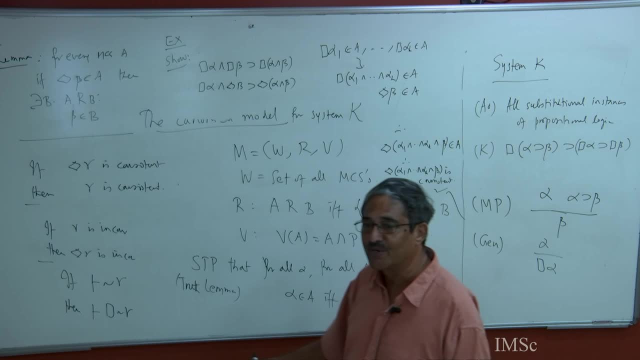 Define that set and show that that set is consistent. How do you show that set is consistent? Bring it, suppose not. actually you do not have to. To show that a set is consistent, you have to show every finite subset is consistent. Consider an arbitrary finite subset. show that it. 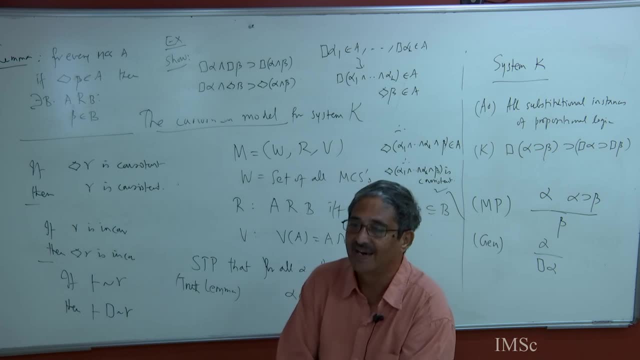 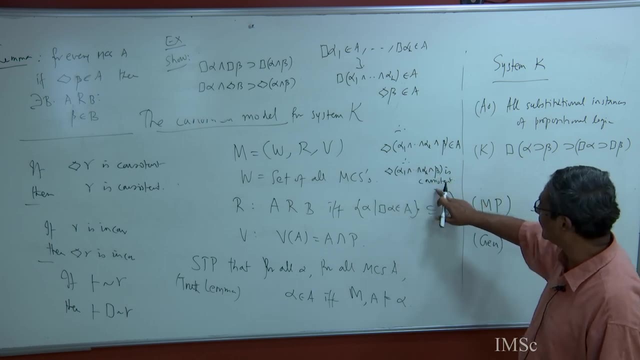 How do you show that set is show that the formula is consistent. That formula is consistent. it suffices to show that diamond of that formula is consistent. Well, to show that this diamond of this formula is consistent, it suffices to show it belongs. 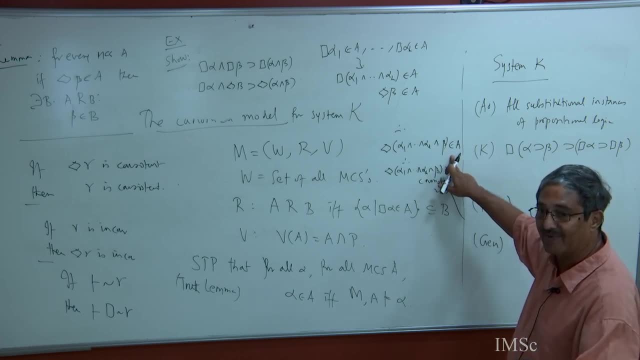 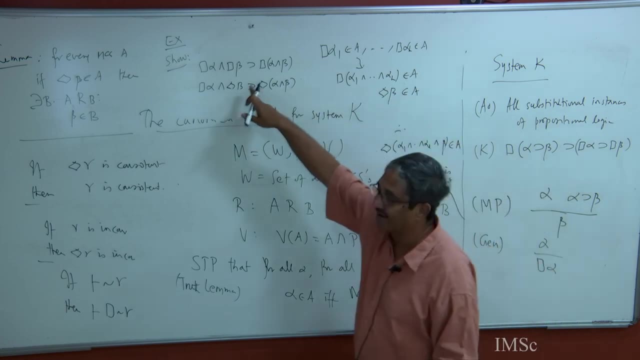 to A. A was the set that we built. We began with. well, why should this formula be in that set? A? well, it is because of these, and we have derived these. So it is like so the way completeness proofs are presented: you start with these axioms. 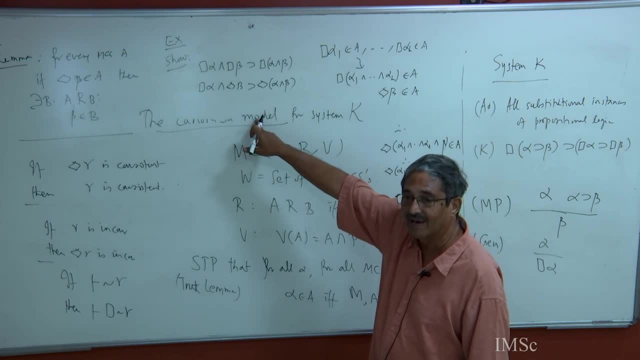 and inference rule show that these two are derivable, right? And this is in a conjunctive form. So how do you get it in? well, it is not very difficult. you know all these. it is just propositional manipulation, so you can get it. 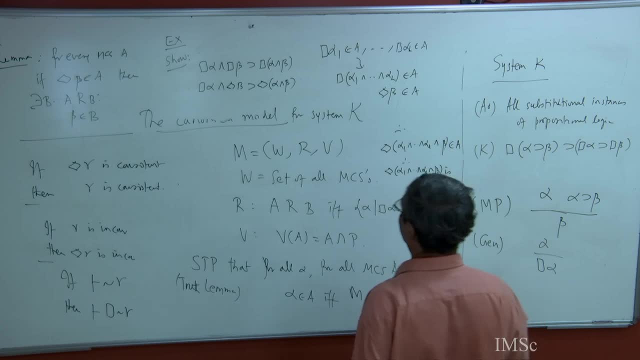 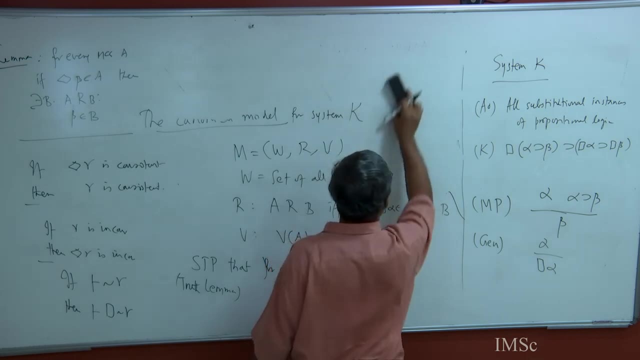 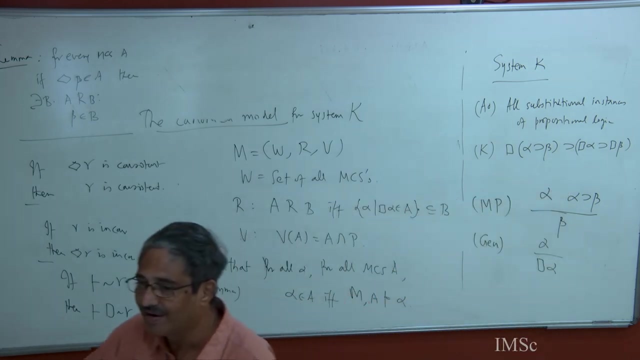 So I hope you can follow up, Thank you, And complete the proof. So this is the main, and it is really a beautiful proof. I mean, it is a very elegant argument. Kripke showed the way, really right, Because now look at something extremely interesting that follows. what is that? 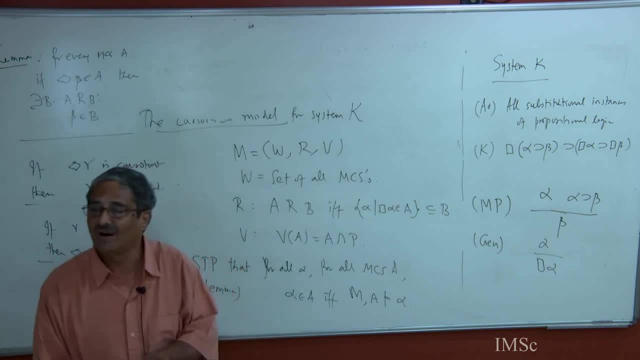 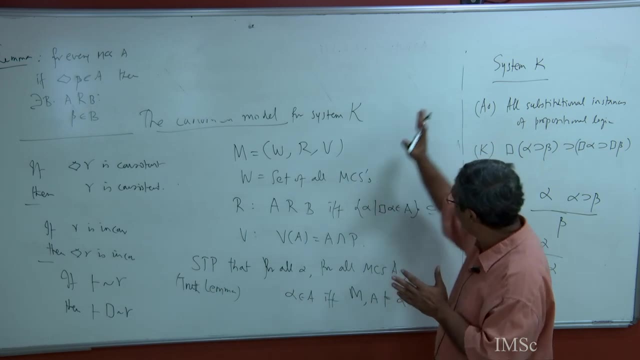 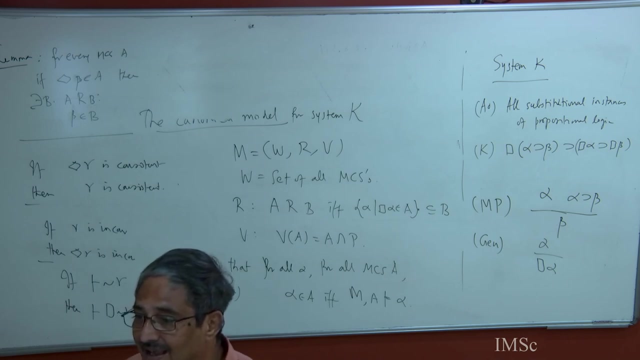 So system K is now complete for propositional model logic And, in fact, what we can, What we can do is to use the same system and prove completeness, not by using the canonical model. You can do a model, what I would call a small model. I mean, this is a crazy model, canonical. 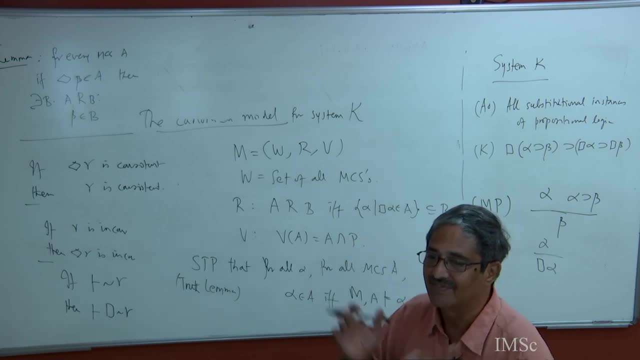 model is anything but small, right. It has the cardinality of the continuum. Who says you should take set of all maximal consistent sets? suppose instead you are given. I want to prove decidability right. Formula alpha is given right. 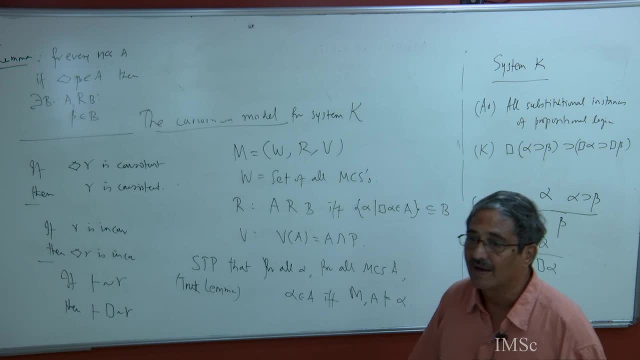 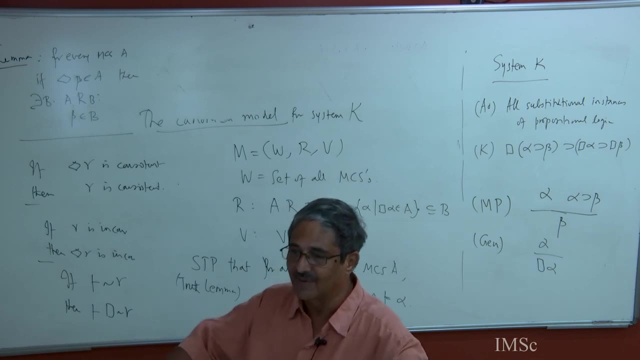 Now I want to show that I mean. what I am saying is: you can do a completeness come decidability proof. We did a separate completeness argument and last time we did a decidability proof. right, You can combine both into one. How would you do that? 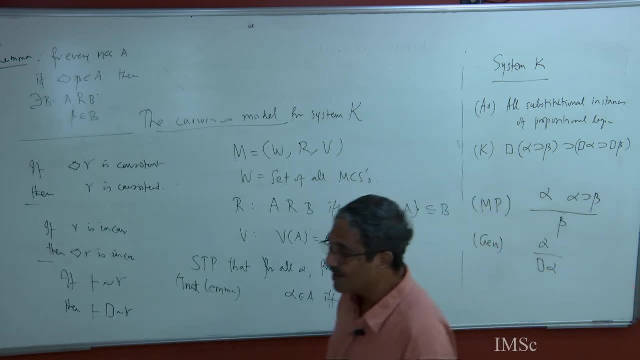 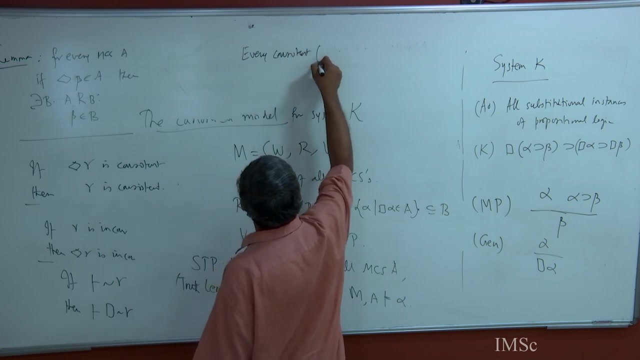 Let me just give you the outline of how it goes. it is not very difficult. I have to show that. Okay, So you give me any formula alpha, consistent formula. So we prove that every consistent formula alpha is satisfiable in a model of size directly. 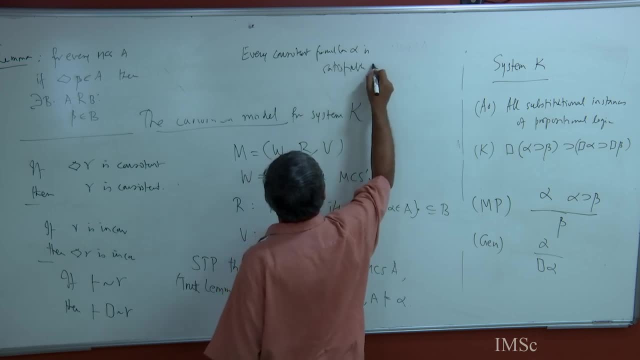 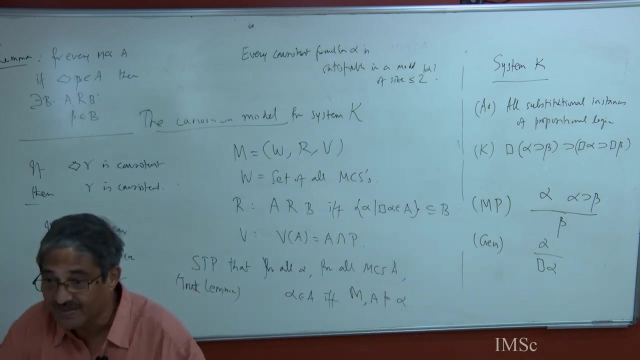 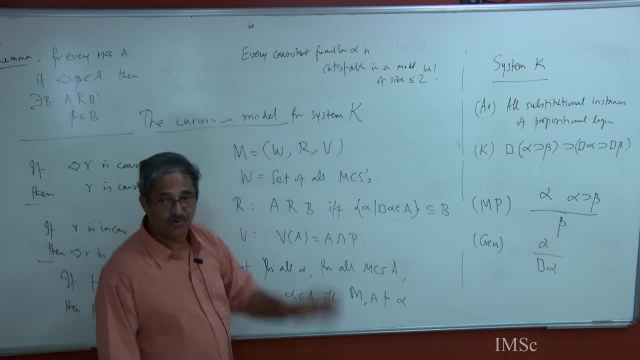 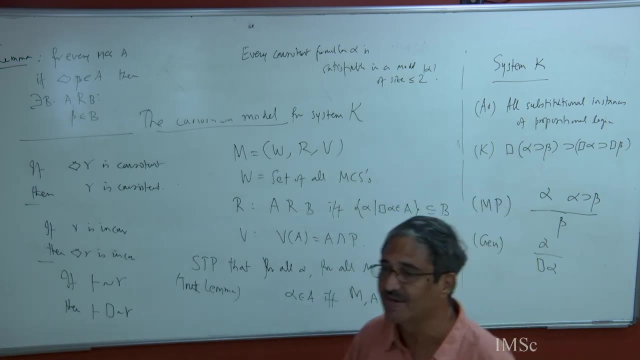 satisfiable formula has consistent. So if you prove this, we have proved that alpha is satisfiable if and only if it is satisfiable in a model of bounded size. That gives you a decision procedure automatically, right, Okay, so you can always do a completeness come decidability proof. So how do you do that? Well, instead. 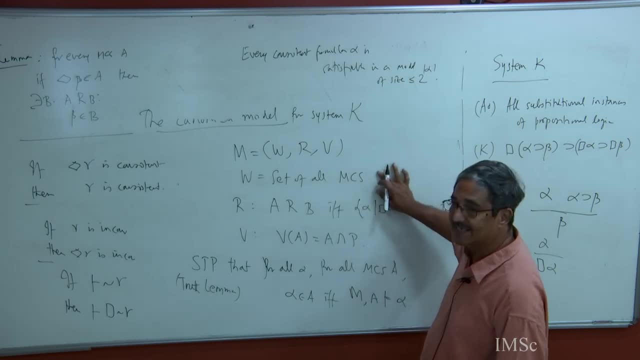 of taking W to be the set of all maximal consistent subsets. I take maximal consistent subsets of sub formulas of alpha naught, No problem. what is stopping you from doing? Take the set of all. So you are given a formula- alpha naught, right, I look at set of all subsets. 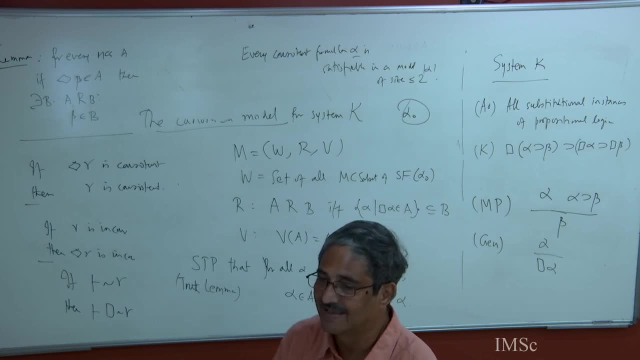 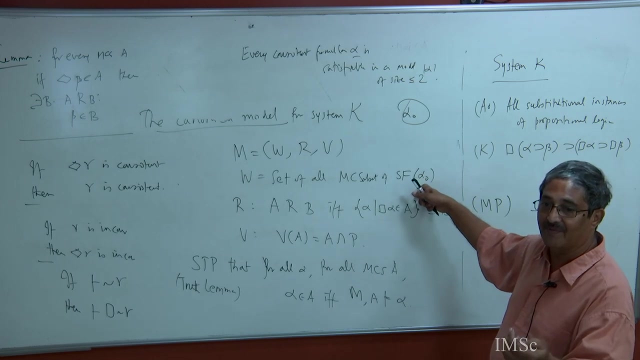 of alpha naught. right, Each subset is a consistent set or not right, Take a consistent set. What do I mean by maximal consistent subset? Well, that means, for every formula, every sub formula of alpha naught, let me say gamma. this particular one will either have gamma, 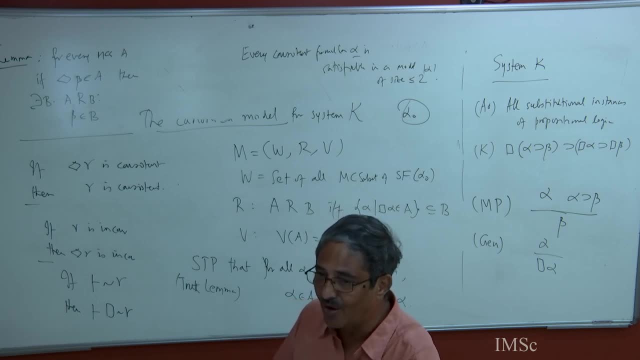 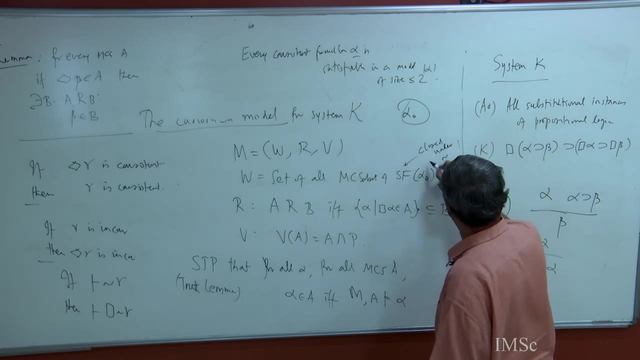 in it, or negative, So it will have negation gamma in it. So all we need to make sure is that sub formulas are closed under negation, which is easy. It will continue to be linear right. What I am saying is, whenever gamma belongs to sub formulas of alpha, naught throw in negation. 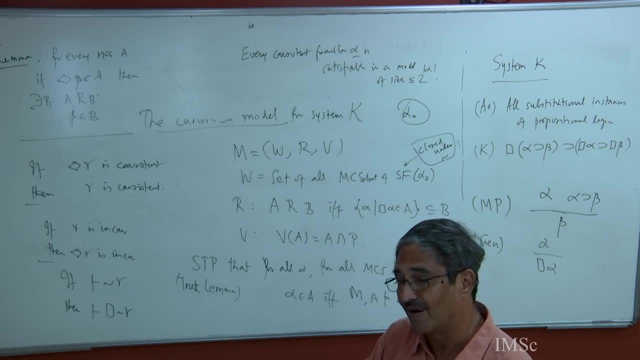 gamma also. Then you will ask what happens to not, not gamma, not, not, not, not gamma. but we can collapse them all right. Not, not gamma is the same as gamma, So I do not have to put it once more. Thank you. 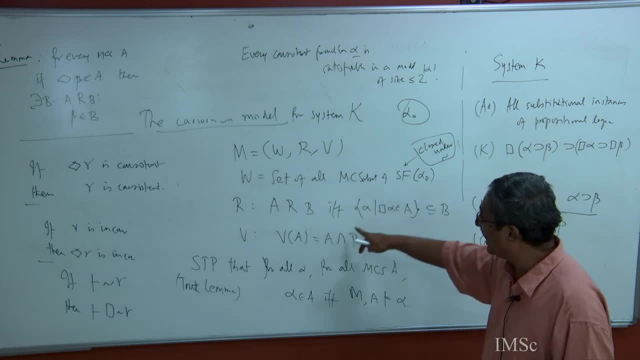 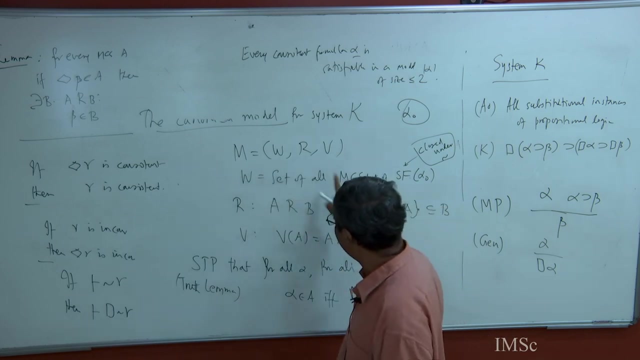 So then, what about this definition? This definition is exactly as before. What about here? Well, exactly as before. The only change is now. notice that the model that we are building right Now, what is the size of W now? What is the size of W?